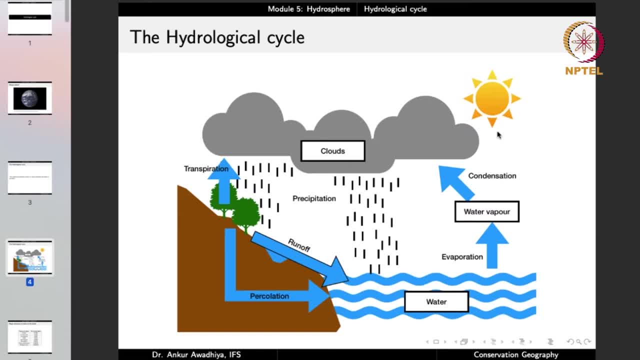 6., 6., 7. lakes and so on. Now this water on getting heated with the heat of the sun, it gets evaporated. So evaporation is the process in which this liquid water converts into water vapor. Now 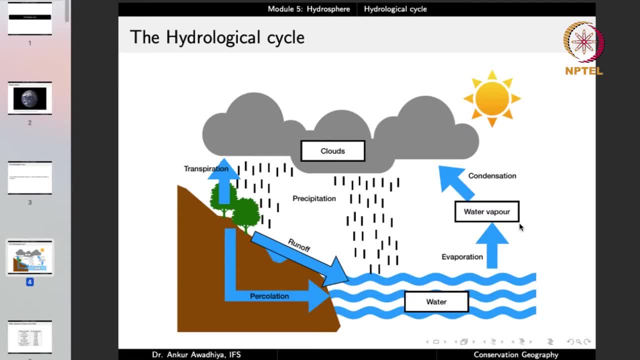 once it has converted into water vapor, it has reached into the atmosphere, So it is now a part of the atmosphere. Now in the atmosphere it can move from one place to another place with the winds. So it moves up using convection currents and then it moves also through advection. 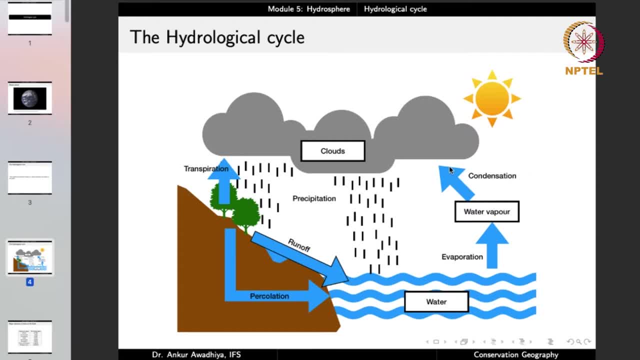 And when it cools down, it condenses. When it condenses, it forms structures such as the clouds, But there are also a number of other structures, such as fog, mist, haze and so on. Now, in these clouds, these clouds can also move with the winds and later on. 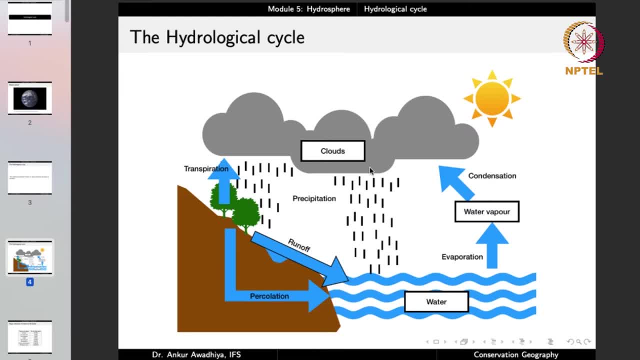 when the water is completely evaporated, it is considered a part of the atmosphere. So when the water is completely evaporated, it is considered a part of the atmosphere. So droplets in the clouds: they coalesce together, they increase in size, they become too heavy. 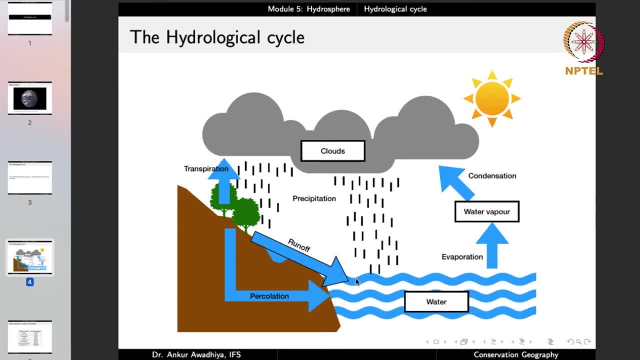 too heavy to remain suspended, and in that case they come down as precipitation, that is, rain. so we can have precipitation in the form of rainfall, in the form of snowfall, in the form of hailstones and so on, and because the clouds can also move together with the winds, we can have this. 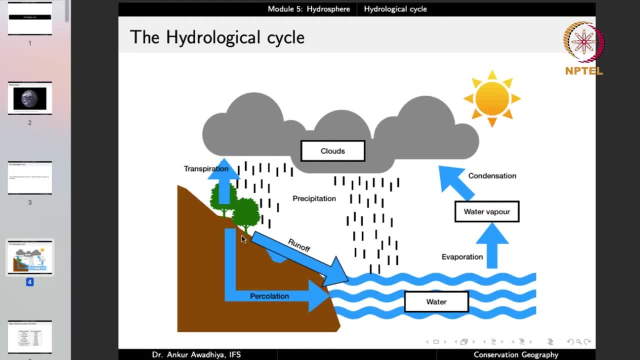 precipitation over the water bodies, or we can have this precipitation over land. now, when the water is there on the land, it starts to move according to the gradient of the land, according to the slope of the land, because of gravity. now this water movement is known as runoff, so some 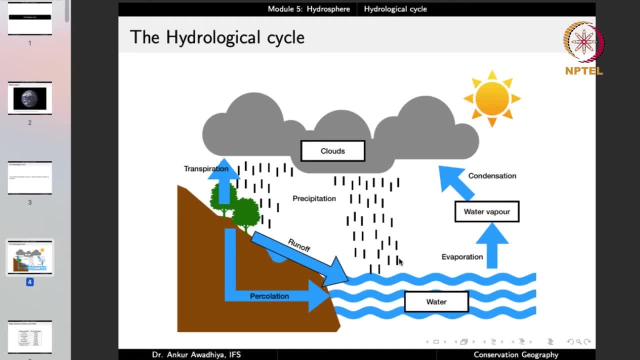 portion of water will run off to these bodies, which are the oceans and the seas. some portion may stand accumulated in the earth, and these accumulated bodies are in the form of lakes and ponds. a fraction of water that has fallen on the ground also is seeped into the earth, so it becomes a part. 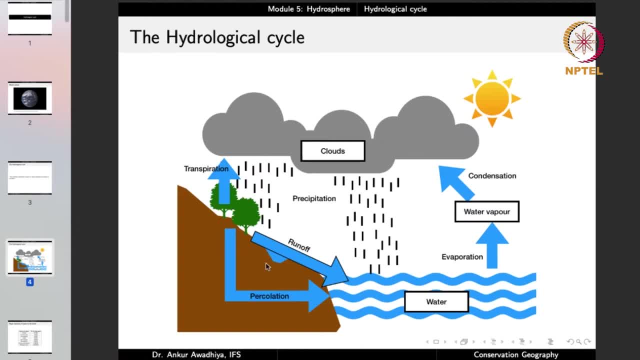 of the ground water. the water in the ground can be taken up by plants, and these plants will then release this water into into the atmosphere through a process that is known as transpiration, or this water that has entered into the ground, it can come out, it can join the surface runoff, or it can directly drain itself into the 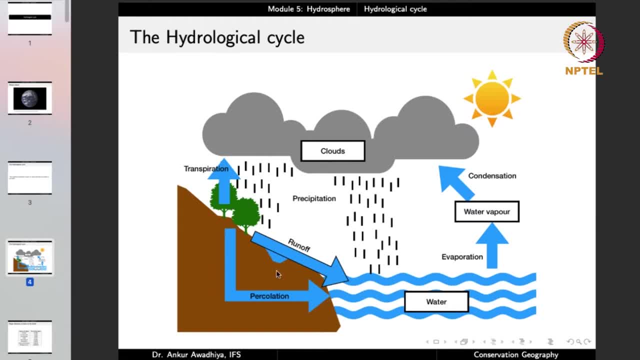 seas and the oceans. so, essentially, if you take water at any point, if you take water in the clouds or if you take the water in the oceans, we can look at a complete cycle. so water starts here, it completes a cycle and it comes back here. so this is the hydrological cycle. 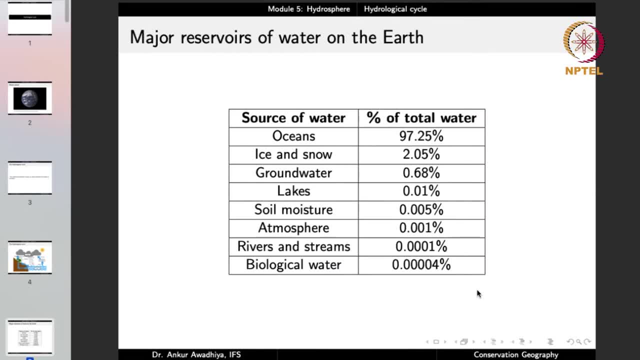 and the hydrological cycle moves water through all the different reservoirs of water on the planet. so we saw that the oceans are the largest reservoir. around 97.25 percent of water is there in the oceans. then we have ice and snow, ground water, lakes, soil, moisture atmosphere. 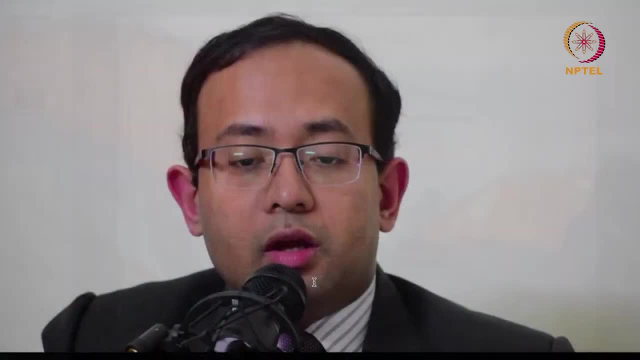 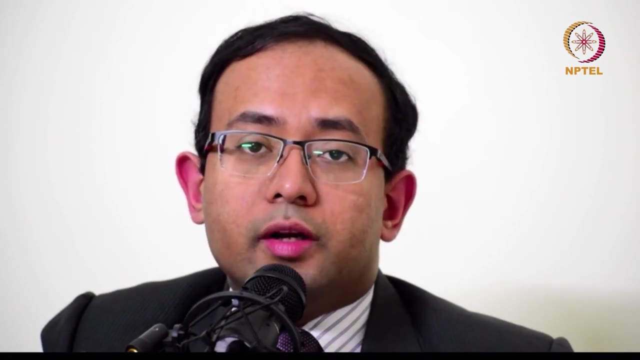 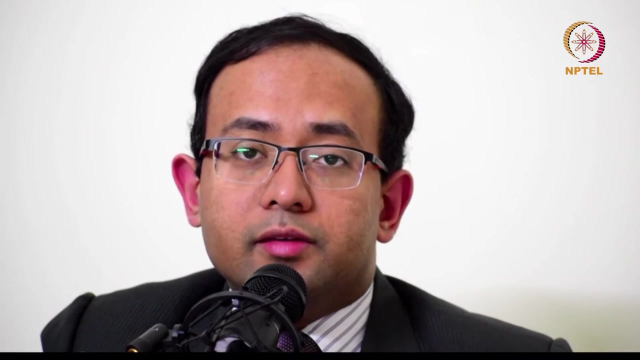 river, sand stream and biological water. so the water cycle is moving water through all of these reservoirs now, because some reservoirs hold water in the form of solid, some other reservoirs hold water in the form of liquid and some of the reservoirs have water in the form of gases. so we have different processes. 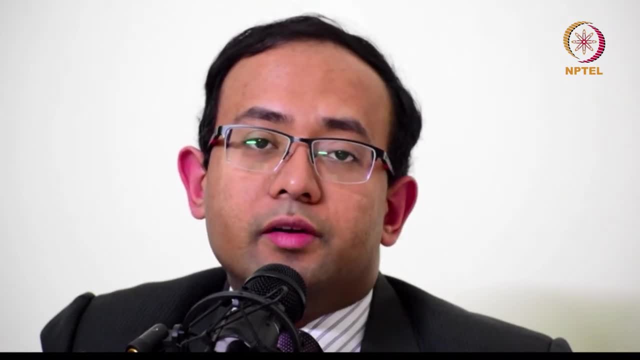 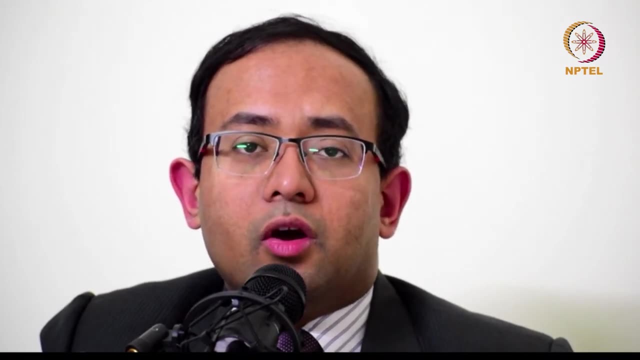 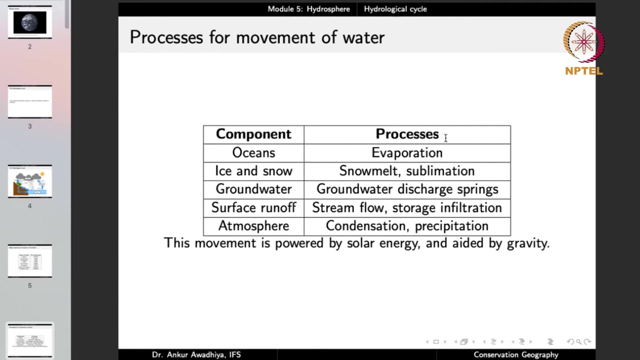 that take place to move this water from one reservoir to another reservoir, so we can have the process of evaporation, condensation, precipitation, sublimation and so on. so in the oceans the major movement or the major process is evaporation. so water leaves the oceans in a 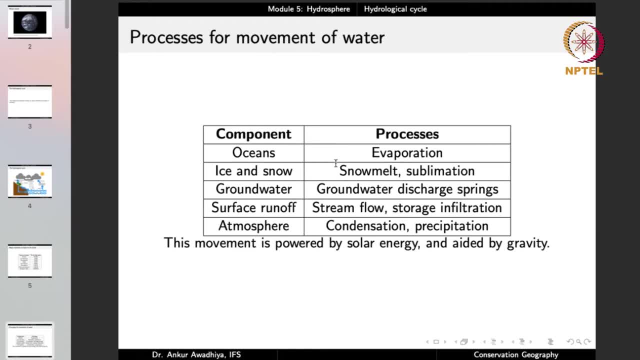 in the form of evaporation In the ice and snow components. we have snow melt and sublimation. So snow melt is the conversion of solid ice into liquid water and sublimation is the conversion of solid ice directly into water vapor or the gaseous form. So the water leaves this component through. 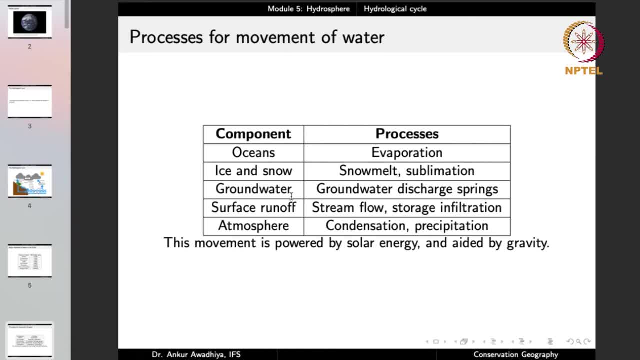 snow, melt and sublimation. Water leaves the groundwater in the form of groundwater discharge springs or it may directly be released into the oceans. Water leaves the surface runoff component in the form of stream flow, in which case it moves into the oceans or it moves in the form. 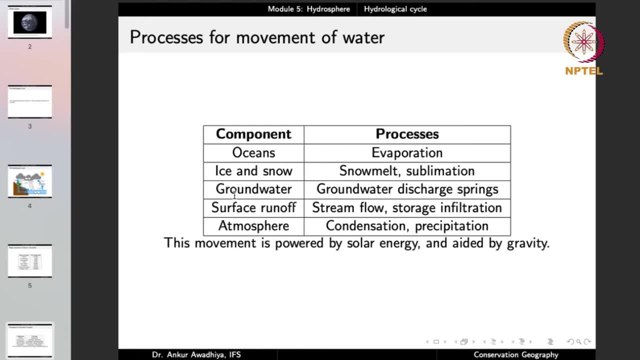 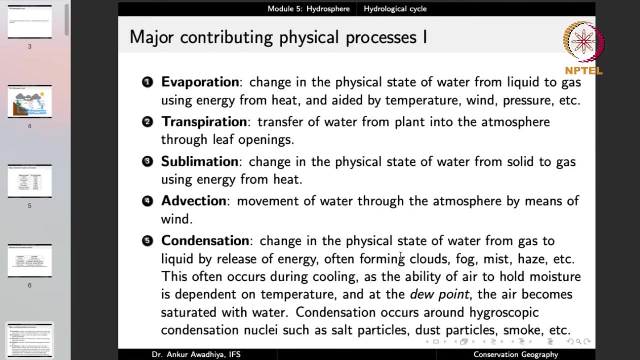 of storage infiltration, in which case it moves into groundwater And water leaves the atmospheric component through condensation and precipitation. And all of this movement is being powered by solar energy, aided by gravity. So let us now have a look at the major contributing physical processes. We have evaporation, which is 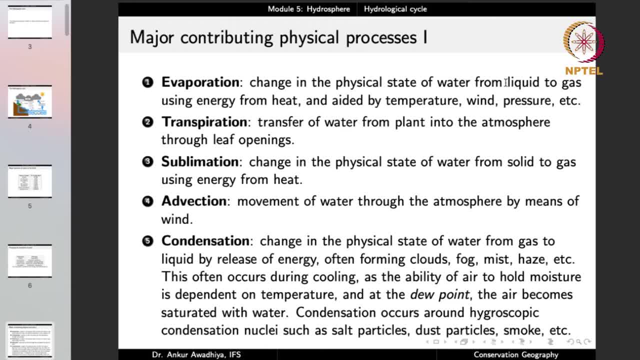 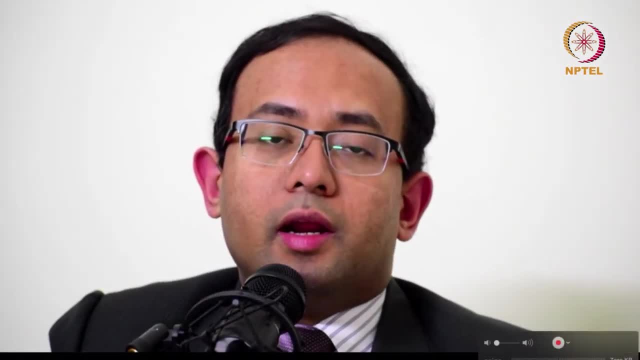 change in the physical state of water from liquid to gas, Using energy from heat aided by temperature, wind pressure differences and so on. So evaporation is the conversion of water from liquid to gas. Now, when water has to convert from liquid to gas, it requires energy. The heat comes simultaneously from theviolation, It is the energy that gets evenly released from the water, which is the latent heat of evaporation or the latent heat of boiling. So in this case this heat is taken from the hoyling and evaporation. The restrictive heat is the surgical heat getRID. 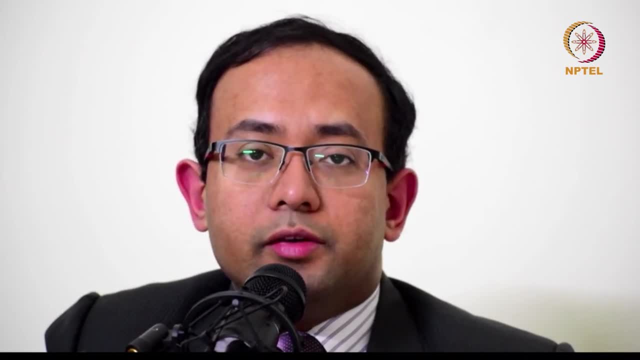 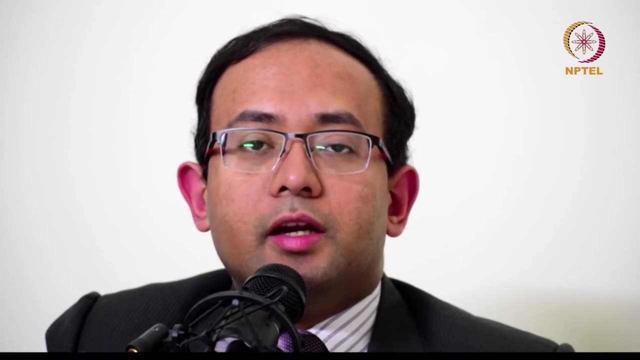 We need to approach the solar feel. when there is a change in flowing stirrum to the którzy make the circulation and another constant water movement which may cause a decrease in theÓ. heat is from the. the solarITY when the electrical energy is seen from all gases. Well, we already talked about east masons. When windشر that bring in evaporation or gas waiter, get this quick Favor, Getting a chance to try our here or here a solution to this problem. think about how. don't not jump this land for your own analysis. ________________________________________________________________〜. increases. It is aided by temperatures, So when temperature increases, the air can hold a larger quantity of water vapor and so more amount of evaporation takes place. It is aided by pressure differences, So if the pressure in an area lowers, then water will convert into water vapor to take. 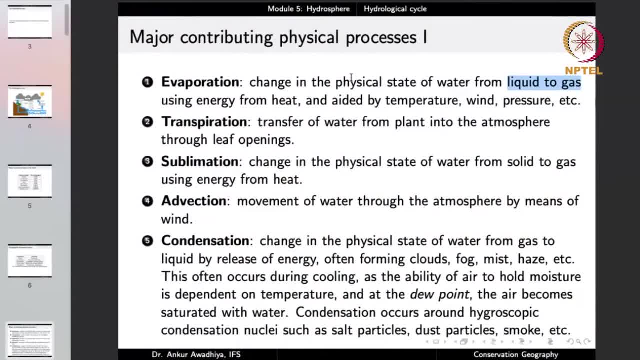 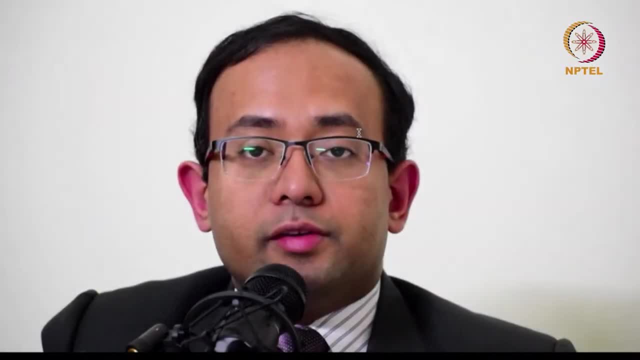 the space. So these are the various aiding mechanisms for evaporation. Then we have transpiration. Transpiration is the transfer of water from plants into the atmosphere through the leaf openings. Now these leaf openings are known as stomata. They are there in the leaves mostly. in the lower surface of the leaf and, through the process of transpiration, water is converted into water vapor and released into the atmosphere. And why do plants need to perform transpiration? It is there to create a pressure gradient So that the plants are able to suck up water from the ground. Now, the water that is coming. 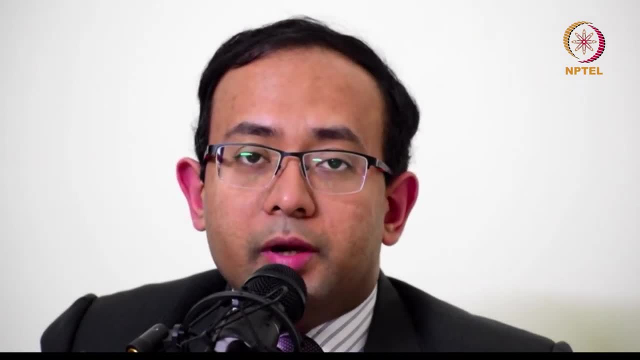 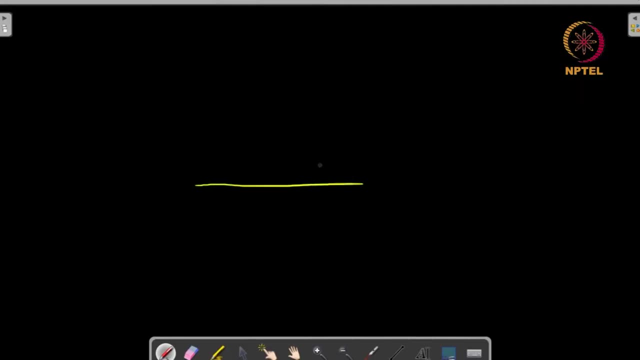 from the ground into the plants will also be carrying a number of minerals which are used as nutrients. So basically, what it means is that if you have a plant and here you have the root system, So the water that is coming from the plant is there in the ground is taken up by these roots, primarily through very small structures. 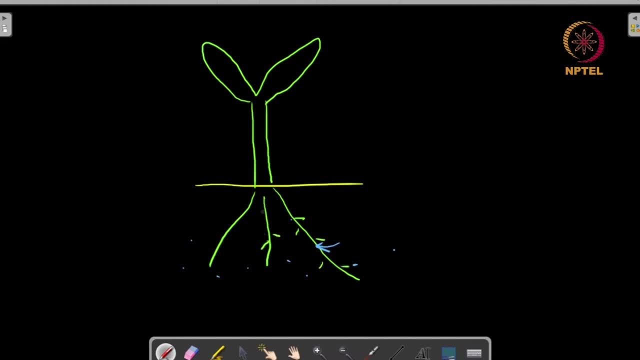 that are known as root hairs. Now, root hairs are there to increase the surface that is available to gather water. So these are the root hairs. Now, when water moves into these roots, then it also carries with it the minerals or different salts that are present in the soil. 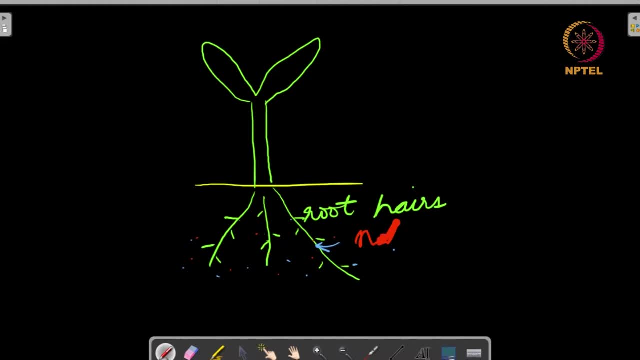 So these salts act as nutrients. So through this process the nutrients are moving into the plants. And to ensure that water keeps moving into the plants, this water, after it is taken up through the roots, it is moving through the stem, it goes into the leaves and from here it is lost into the atmosphere. 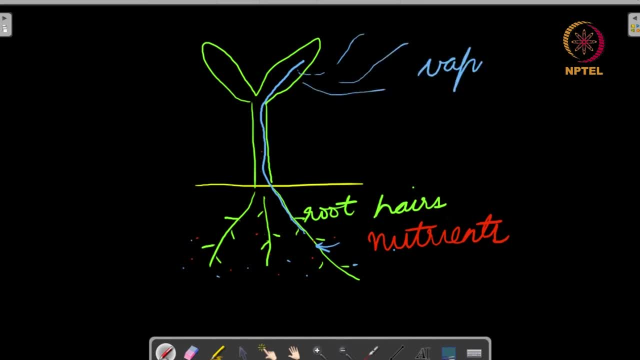 In the form of water vapor. Now this loss of water. if this loss of water did not happen, then where would all of this water go? The plants have a limited capacity to hold water, and if that capacity is exceeded, then this process would stop. 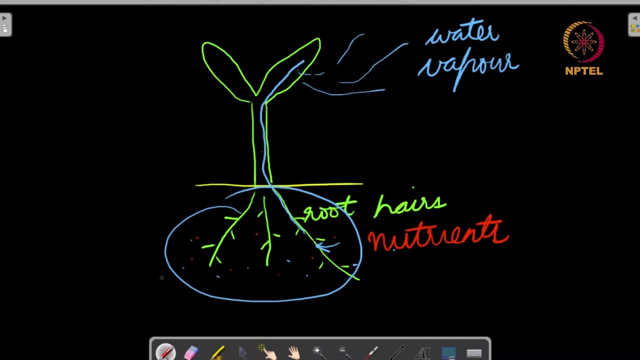 And in that case the plants will not be able to get their nutrients. At the same time, plants also require water to perform photosynthesis. So if we write the equation of photosynthesis it goes like this: 6 CO2 plus 6 H2O in the presence of light and in the presence of chlorophyll. 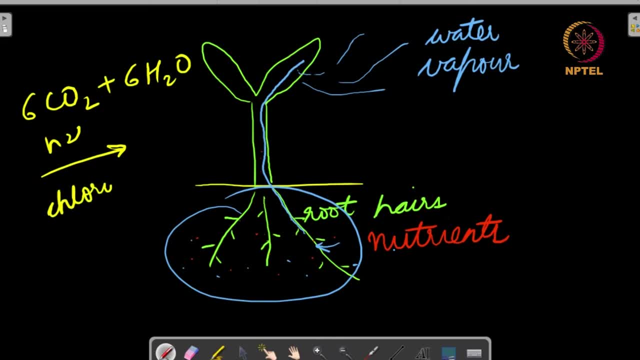 It gives C6H12O6,, which is glucose plus 6 oxides. So this is what we get. This is what we get. This is what we get Plus 6 oxygen. So, essentially, plants are using up carbon dioxide and they are using up water. 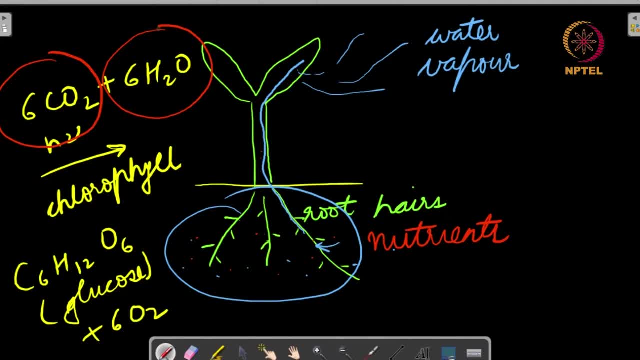 So water is also one of the reagents. to perform photosynthesis. They require light and they require chlorophyll, And when all of these are together then in the plants glucose will get generated. Glucose is a carbohydrate. Glucose is a carbohydrate. 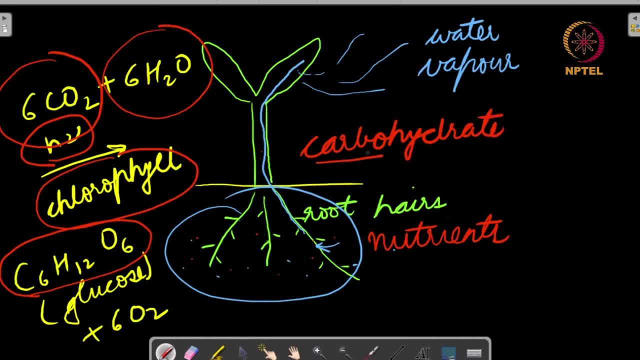 Glucose is a carbohydrate, So carbo refers to the carbon portion, So it has carbon And hydrate means that it has water. So basically you can write C6H12O6 also as CH2O whole 6.. So in this case it has carbon and it has water. 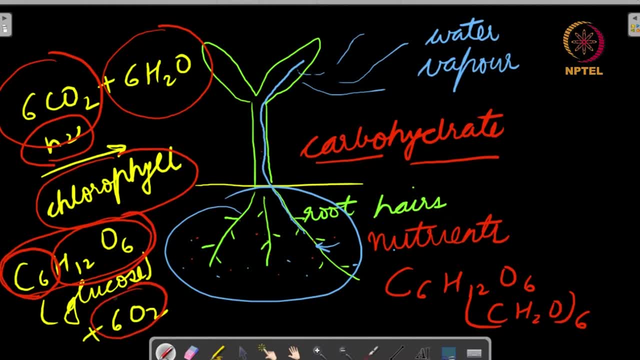 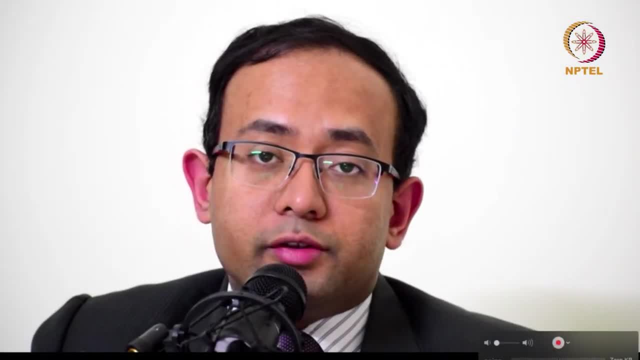 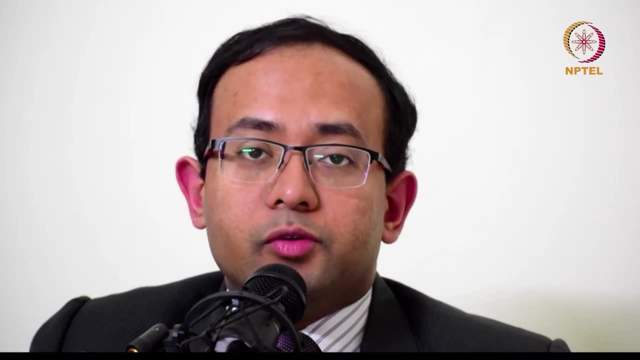 So it is a carbohydrate And it will also release oxygen, And we have observed before that this release of oxygen is what led to the great oxygenation event That changed the composition of the atmosphere. So this is where the oxygen in the atmosphere comes from. 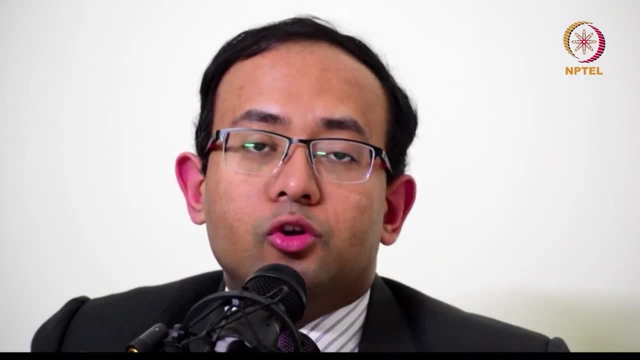 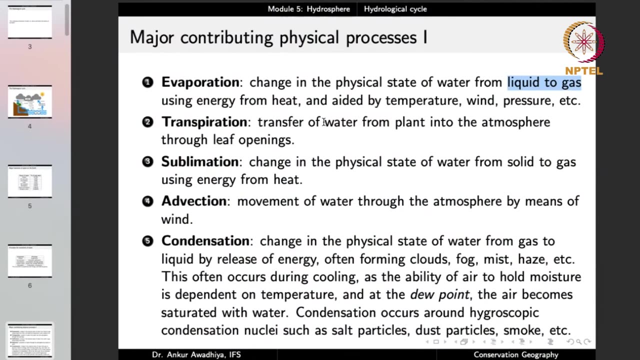 So plants need to perform transpiration to get water and the nutrients from the soil. So this is a process in which water in liquid form, which was present in the ground, is converted into water vapor and released into the atmosphere through leaf openings that are known as stomata. 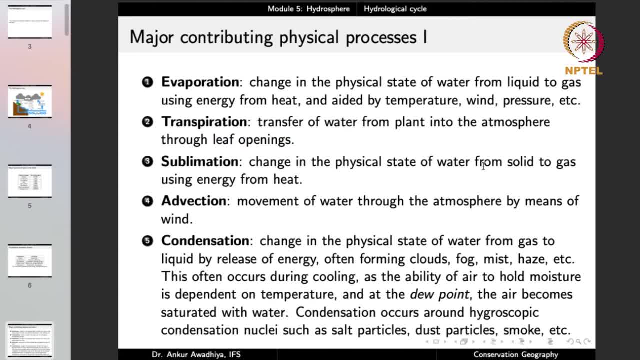 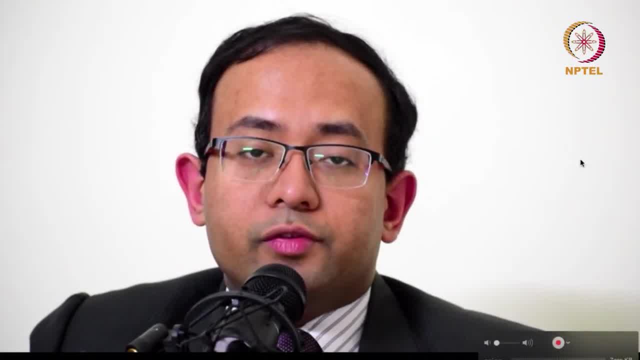 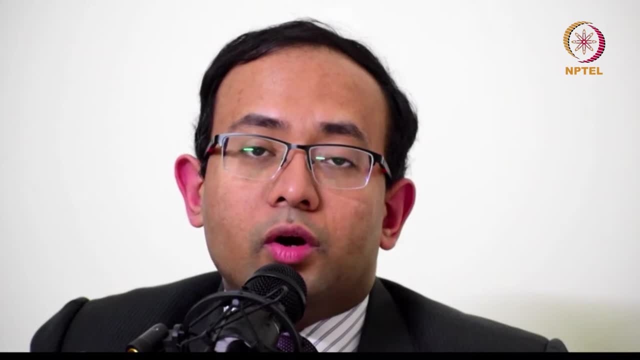 Then we have sublimation. Sublimation is change in the physical state of water, from solid to gas, using energy from heat. So in the process of sublimation water does not convert from solid to liquid and then move into gas. Water directly moves from a solid state into a gaseous state. 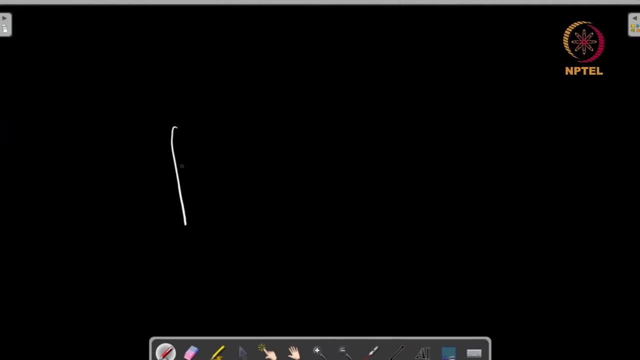 So, essentially, when we talk about sublimation, if you have a block of ice, then the water that is there in this ice will directly get converted into water vapor, And this process is known as sublimation. Another process is advection. 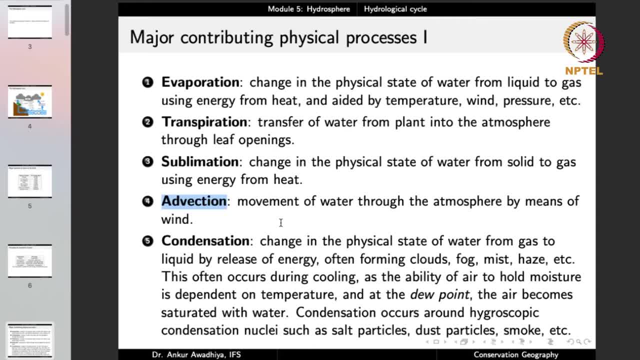 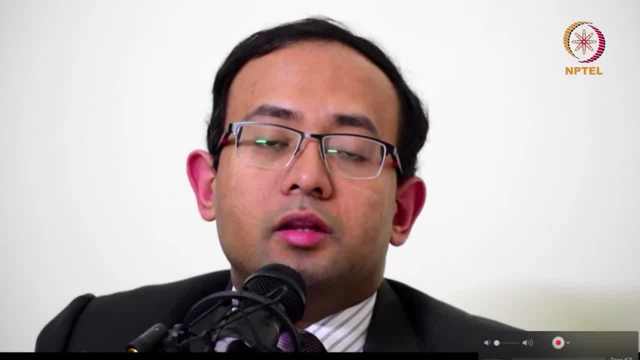 Advection is forced movement of water together with the winds. So it is movement of water through the atmosphere by means of wind. So when you have wind movement, the water that is there in the air in the form of water vapor that also moves. 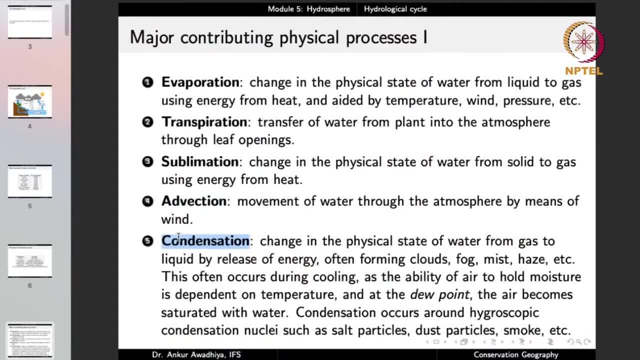 So this is the process of advection. Then we have condensation. Condensation is the opposite of evaporation. So in condensation it is a change in the physical state of water from gas to liquid by release of energy. So in the case of evaporation it required energy. 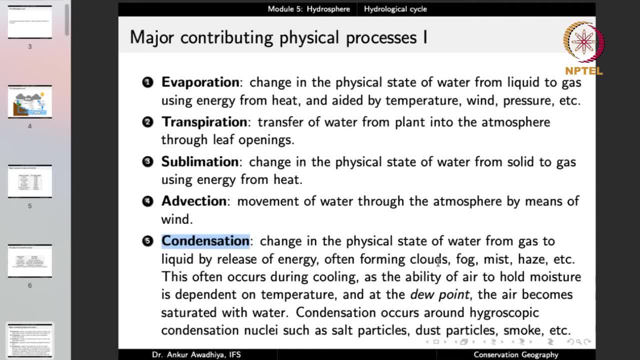 In the case of condensation, it releases energy, Often forming things such as clouds, fog, mist, heat Haze, etc. This often occurs during cooling, because you have to release energy in the form of heat, So this release of energy will happen in a cool surrounding. 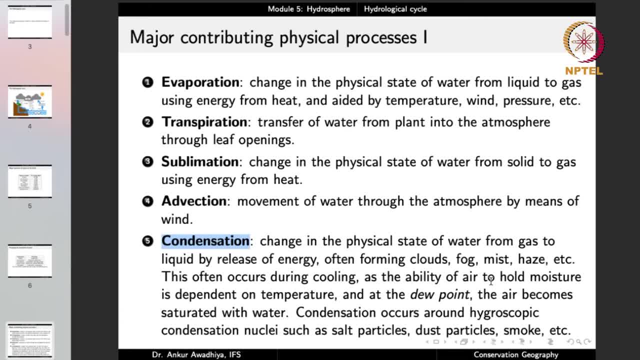 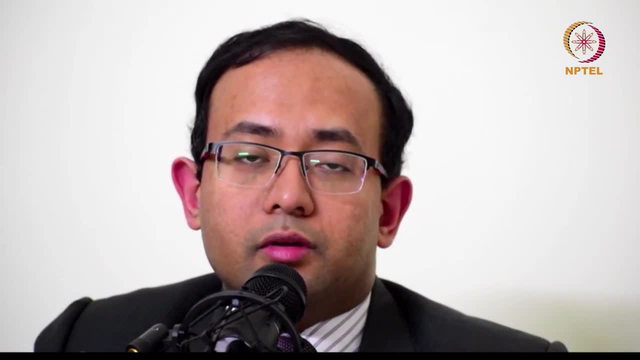 So this often occurs during cooling, as the ability of air to hold moisture is dependent on the temperature, And at the dew point the air becomes saturated with water. What does that mean? The air has a limited capacity to hold moisture. Now, the air has a limited capacity to hold moisture. It is dependent on the temperature. If you heat up the air, then it will be able to hold a larger quantity of water vapor. If air cools down, then it will be able to hold a smaller quantity of water vapor. Now, dew point is the point at which the air is 100% saturated with water. 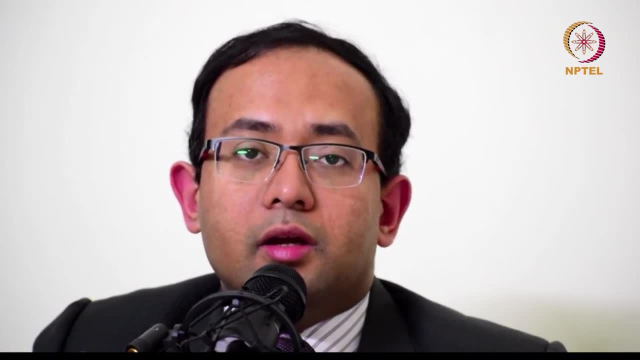 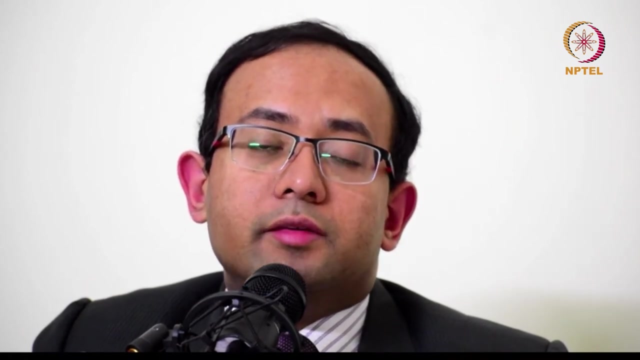 So you take air at a higher temperature, add moisture to it and then you reduce the temperature of the air, So at some point you will have air that is 100% saturated. That is, the amount of moisture that is present is equal to the capacity of air to hold moisture. 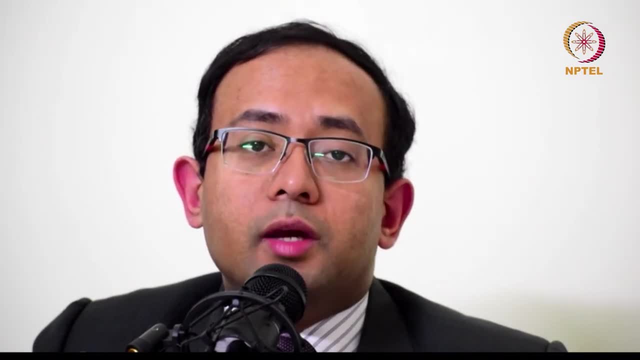 And beyond this point, the moisture has to be lost from the air because it does not have any further capacity to hold this moisture. So this loss of moisture will happen through the process of condensation. So in condensation this moisture in the form of water vapor, 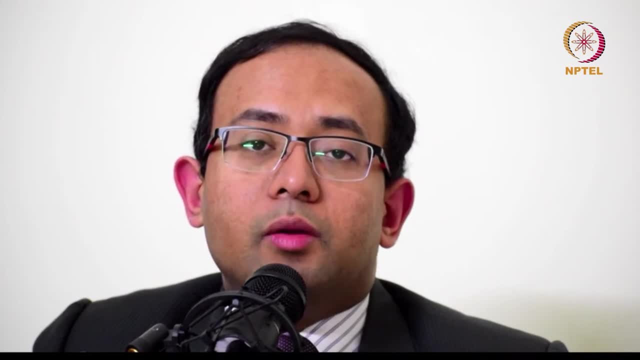 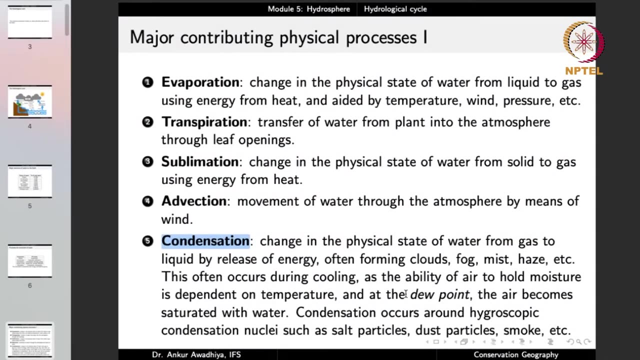 will be converted into liquid water and it will be shed out of the air, And this happens when the temperature is at the dew point or below the dew point. Condensation occurs around hygroscopic condensation nuclei, such as salt particles, dust particles, smoke, etc. 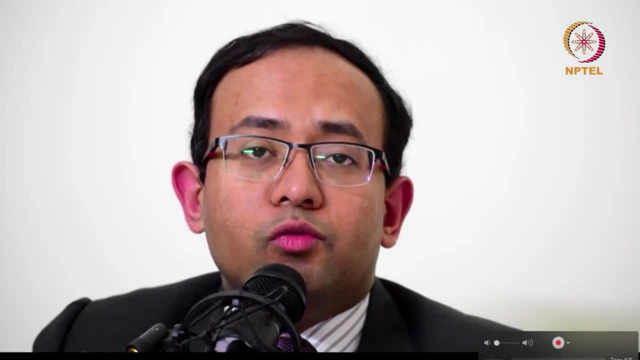 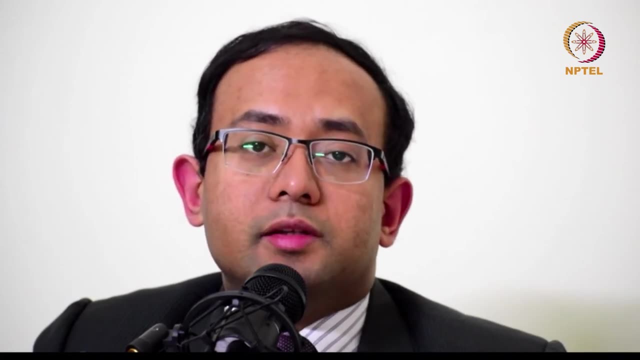 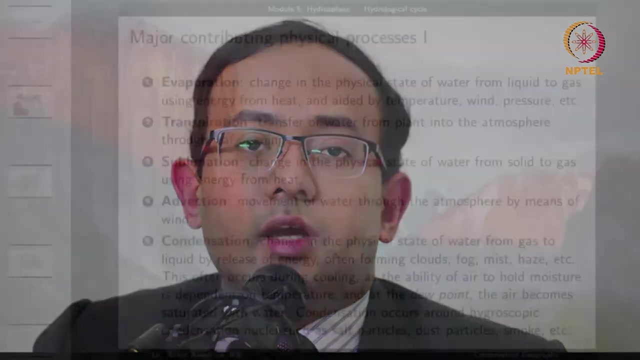 So when condensation is happening, it has to leave water somewhere, And typically the water is left around the hygroscopic particles such as dust or salt. So these are known as condensation nuclei, because when condensation occurs it is around these particles. 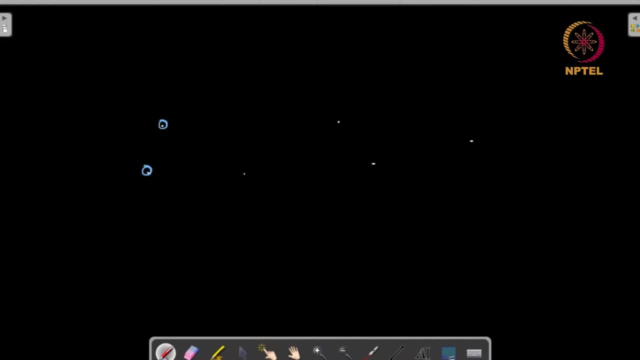 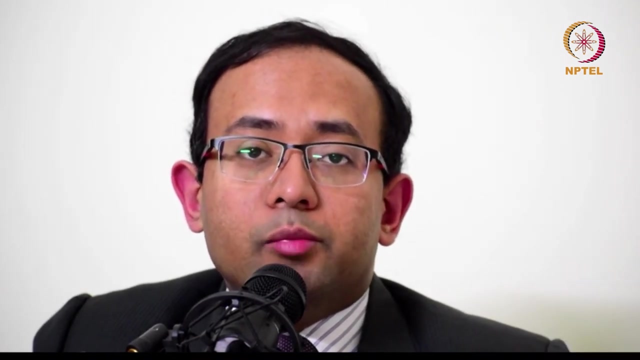 that the water will condense in the form of a liquid, So these act as nuclei to start the condensation process. If you do not have these nuclei, then perhaps the air would not find a mechanism to release the water, So it will become supersaturated. 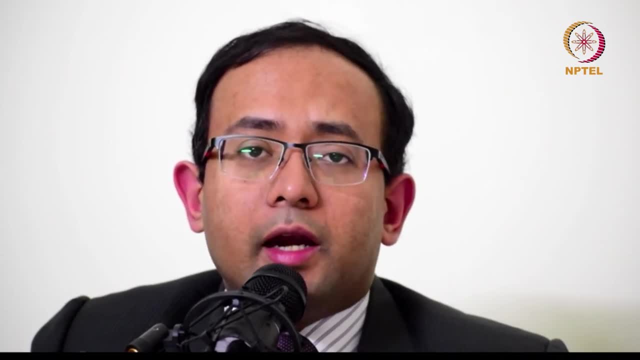 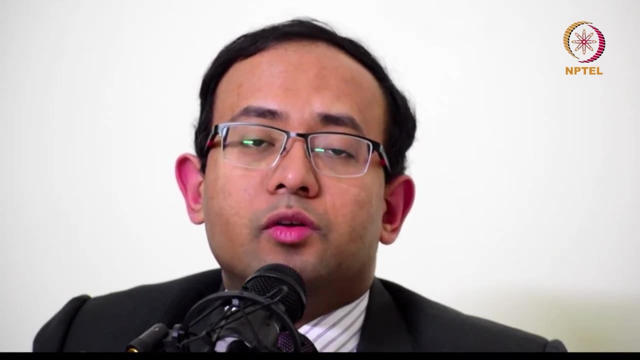 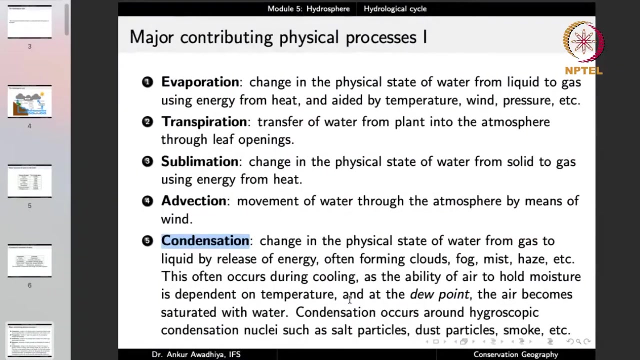 That is, holding water above its capacity. And as soon as it gets any impurity or it gets any surface on which it can shed the water immediately, it will shed the water. So these particles are known as condensation nuclei. Another process is deposition. 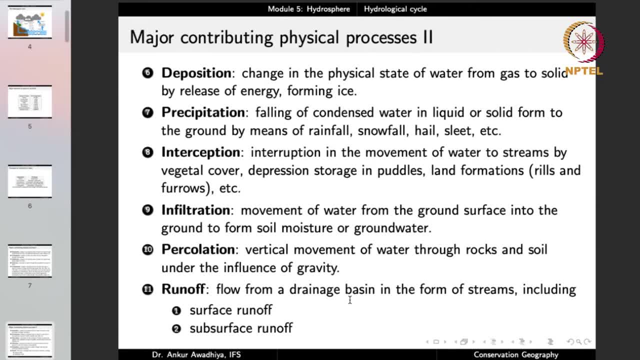 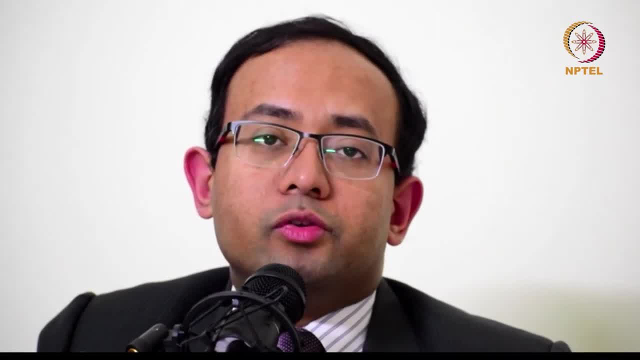 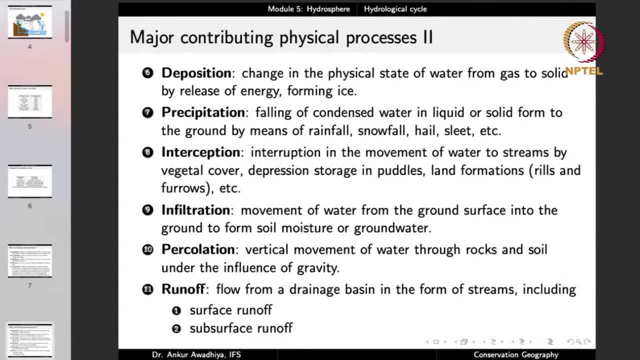 Now, deposition is the opposite of sublimation. In sublimation, water converted from solid to gas without going through a liquid phase. Similarly, in the process of deposition, water moves from gas to solid without going through the liquid phase. So deposition is the change. 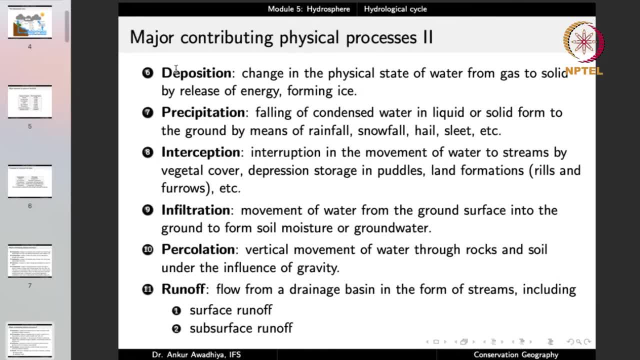 in the physical state of water from gas to solid, by release of energy and forming ice. Then we have precipitation, which is falling of condensed water in liquid or solid form to the ground by means of rainfall, snowfall, hail, sleet, etc. 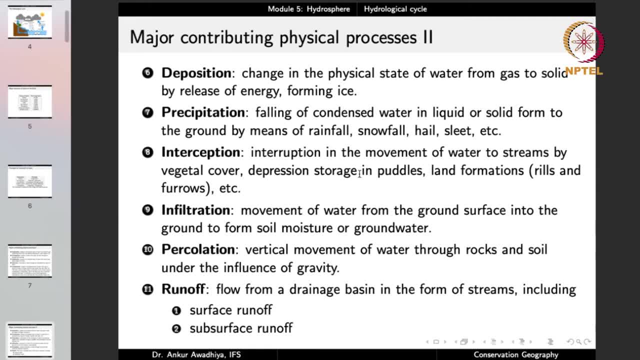 So the falling of the condensed water, either in liquid form, such as rainfall, or in a solid form, such as snowfall or hailstones, or a mixture, such as sleet. Now, sleet is a mixture of water and snow. So this condensed water in the form of solid or liquid, or a mixture, 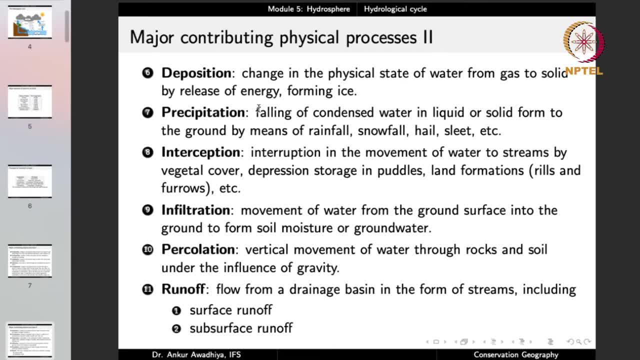 it falls to the ground by means of this process that is known as precipitation. So precipitation means rainfall, snowfall, falling of hailstones, falling of sleet, and so on. Next we have interception, which is interruption in the movement of water to streams by vegetal cover. 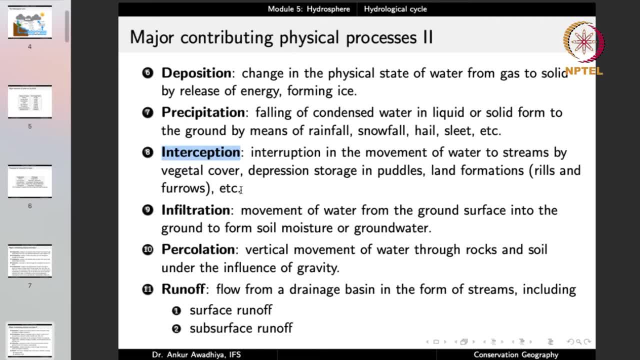 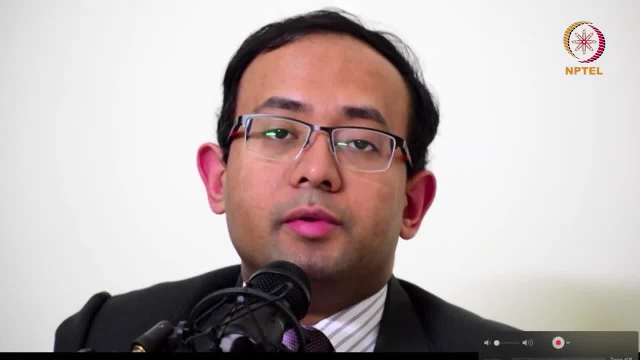 depression storage in puddles, land formation, rills and furrows, etc. Now interception is the interruption in the movement of water to the streams. So essentially what happens is that when you have rainfall, the water that falls down to the earth it tends to move towards the streams and with the streams it will tend to move towards the oceans. Now, interception is the interruption of this process That is, in the process of interception, the water is interrupted from moving into the streams and into the oceans. 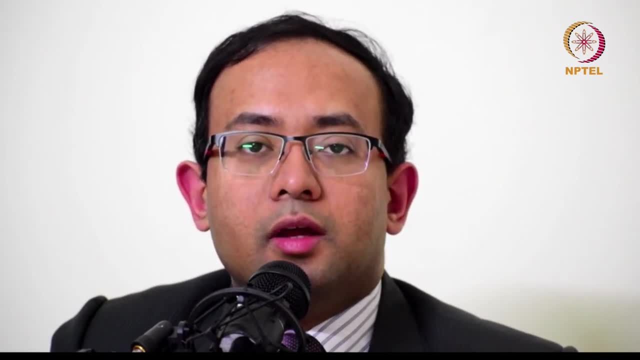 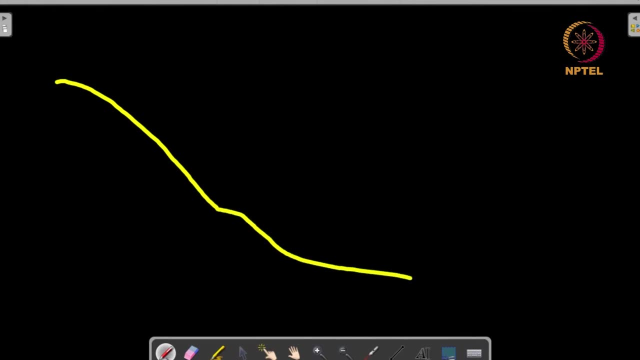 Now, how can we have these interruptions? Suppose water is moving. so suppose this is a land formation and you have water that is flowing like this. Now, in this case, at this spot, suppose there is a small depression here, So in this case the water will get accumulated here. 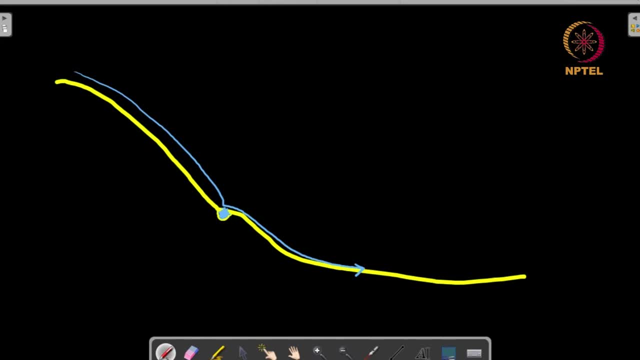 Some amount of water gets accumulated, And so this water is now not directly moving into the streams. This is an interruption in the flow of this water, So this is interception. Another way is in the form of trees, So when you have a tree, 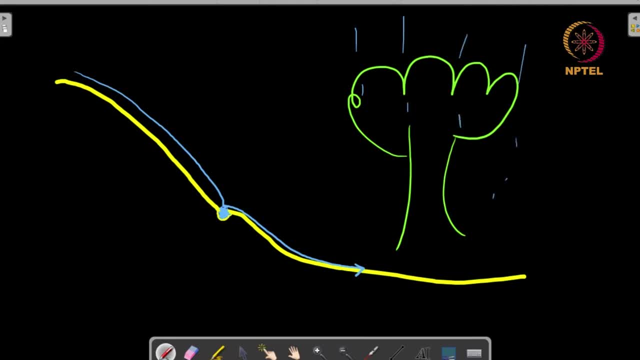 the water that was falling down in the form of rain water. it now does not directly reach into the ground, So the trees stop this movement of water and this water gets collected in these canopies. So this is the tree canopy, which is the leaves and the branches. 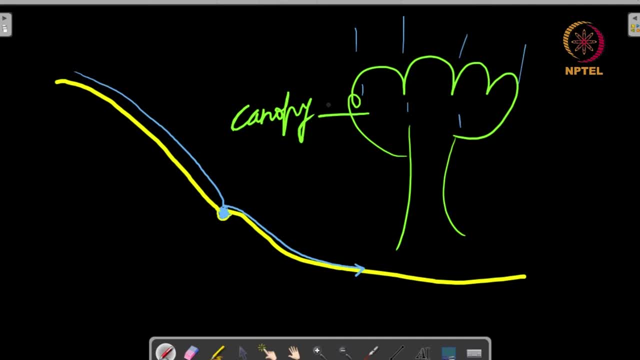 So these leaves and the branches, they hold the water, And after some time this water will start to move through the bark and through the stem of this tree, in a process that is known as stem flow, And then it will reach the ground. Now, if the water had directly fallen on the ground, 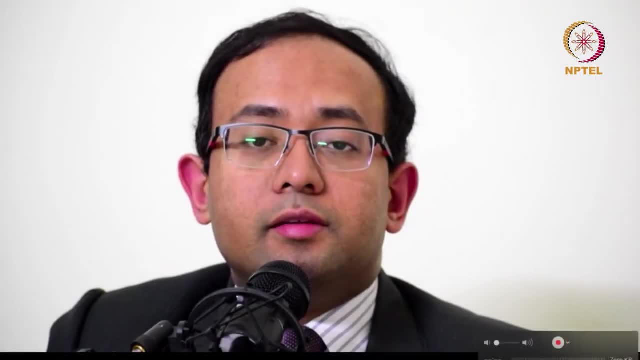 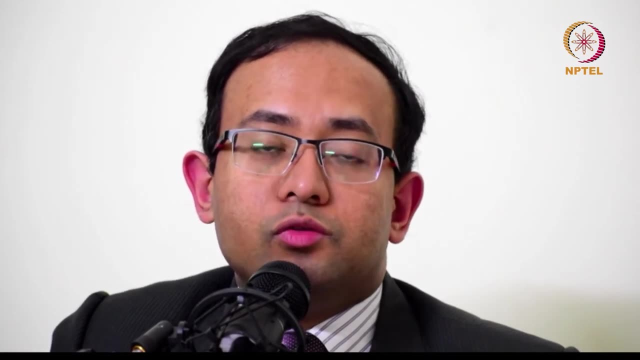 it would have fallen at a very high speed. So in that case the rain water would have done a lot of erosion and then it would have swiftly moved into the nearby streams. But what do these trees? do These trees stop that movement of water? 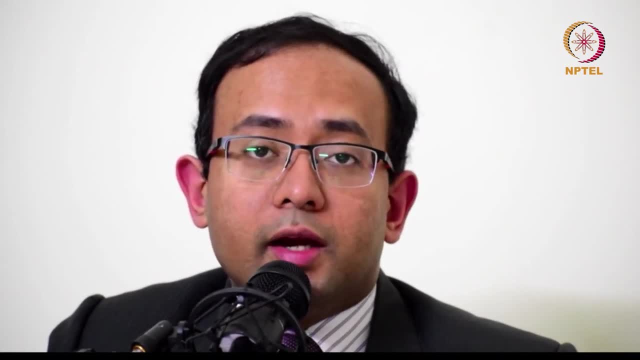 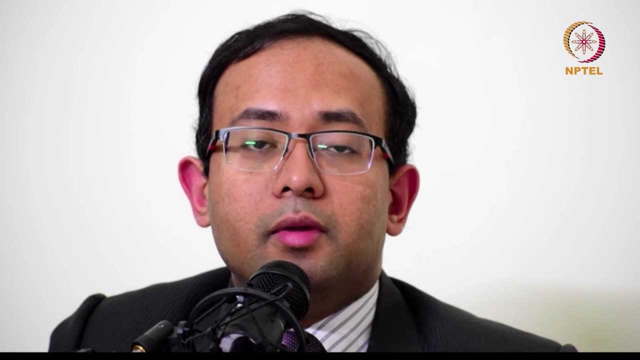 They interrupt the water from directly hitting the ground, slowing it down, And so the amount of erosion becomes less and the soil gets protected. And at the same time, when this water moves down, it moves through the stems of these trees. So if you stand under a tree, 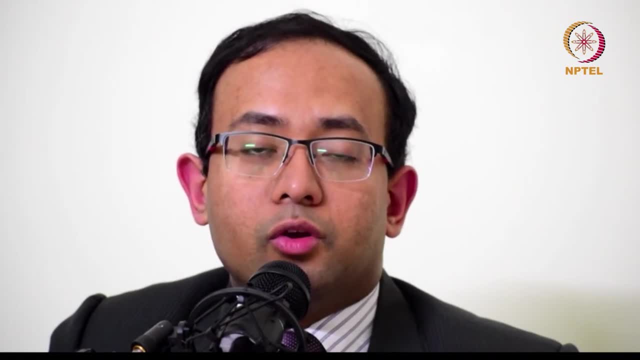 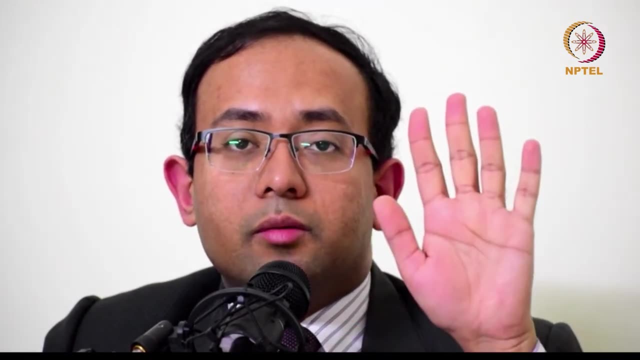 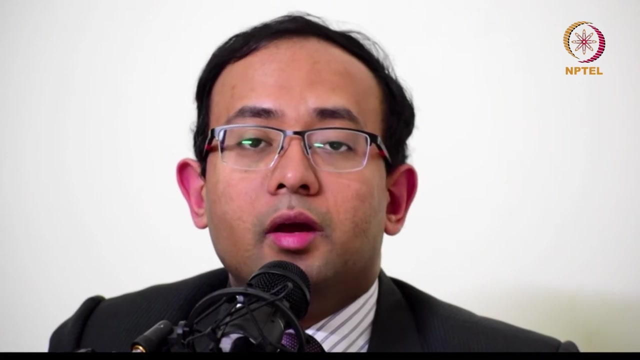 during a rain, you'll find that you are not getting hit directly by the rain water. But if you touch the stem of the tree, you'll find that it is damp. it is wet Because water is moving through the surface of the stem into the ground. 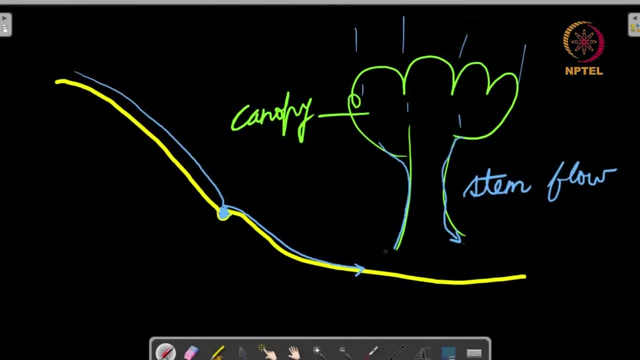 And typically the roots in these locations. they are able to dig into the soil. So when this water comes here now, this water will not move in the form of a surface flow. This will not happen, But it will slowly get absorbed into the soil. 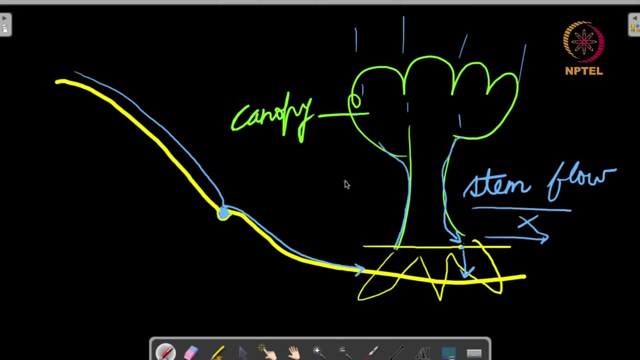 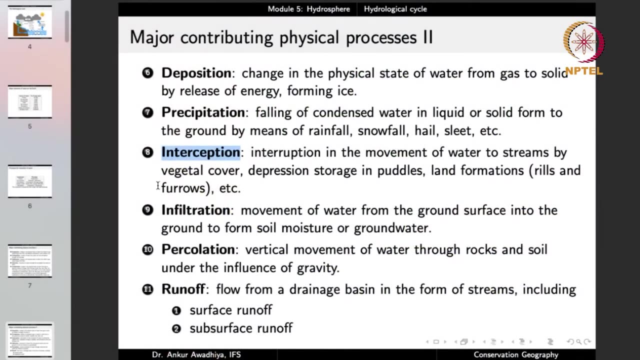 So it will become a part of the ground water, And so, in this way, the water is not moving into the streams in the form of surface runoff, but it is getting into the ground. So this is the importance of interception Now, after interception. 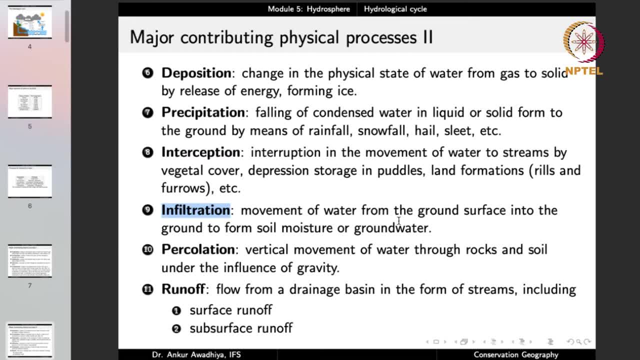 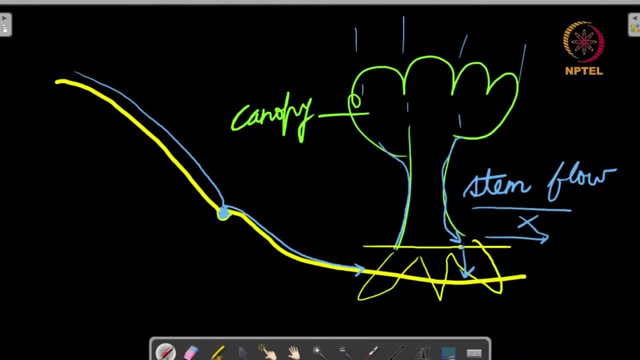 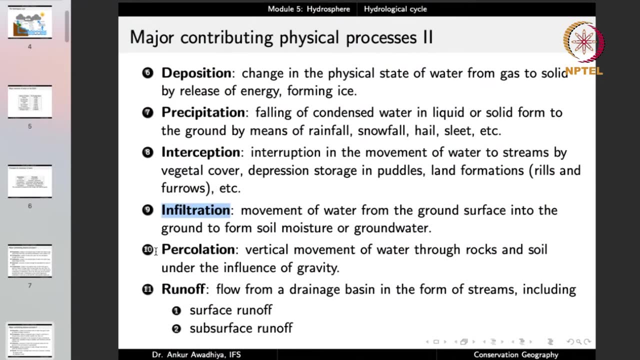 we also have infiltration. Infiltration is the movement of water from the ground surface into the ground to form soil, moisture or ground water. So after this interception, when the water is moving into the ground, this is infiltration. Once the water has entered into the ground, 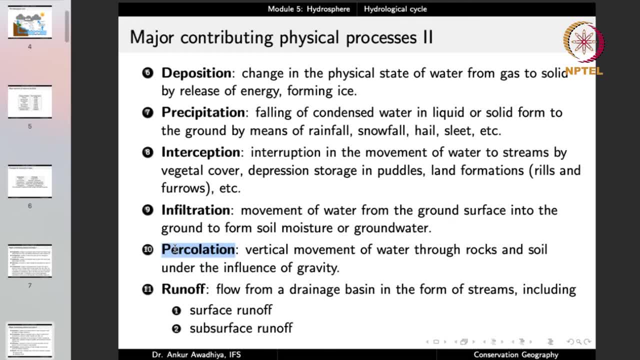 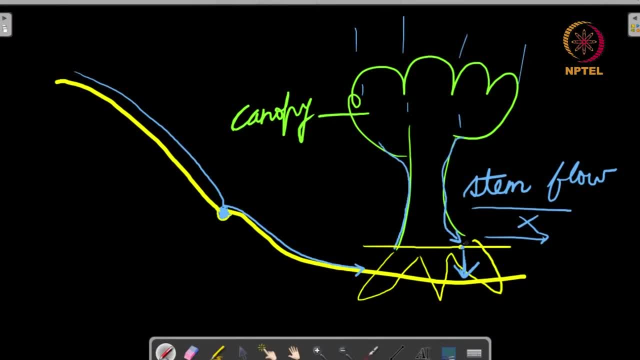 there will be percolation. Percolation is the vertical movement of water through rocks and soil under the influence of gravity. So once this water has entered into the soil- here in the form of infiltration, now it is moving down under the influence of gravity. 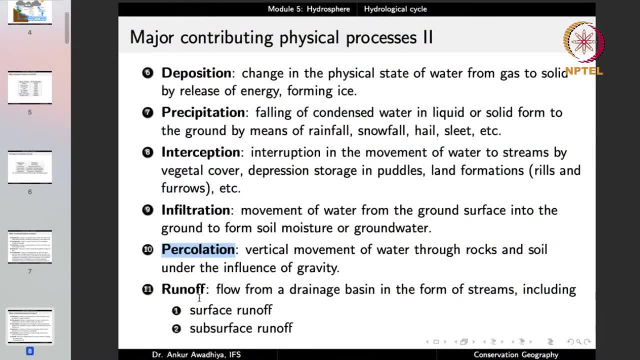 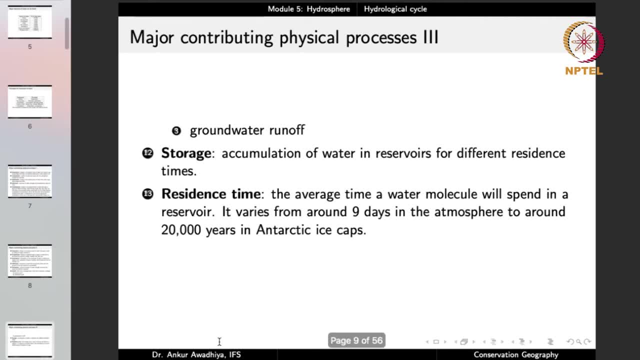 And this is percolation. Next, we have runoff, which is flow from a drainage basin in the form of streams, including surface runoff, subsurface runoff and ground water runoff. So, essentially, when we talk about the movement of water in the streams, 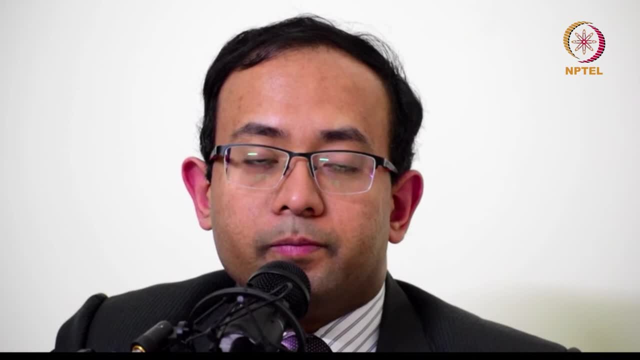 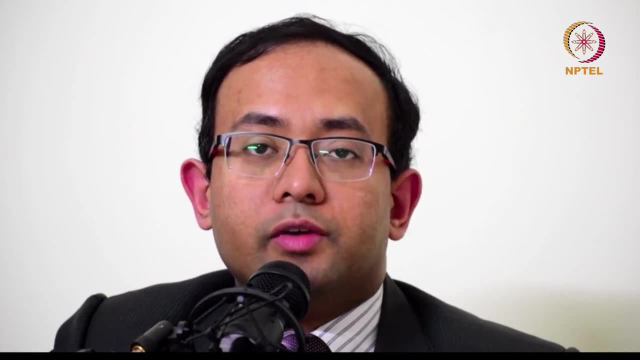 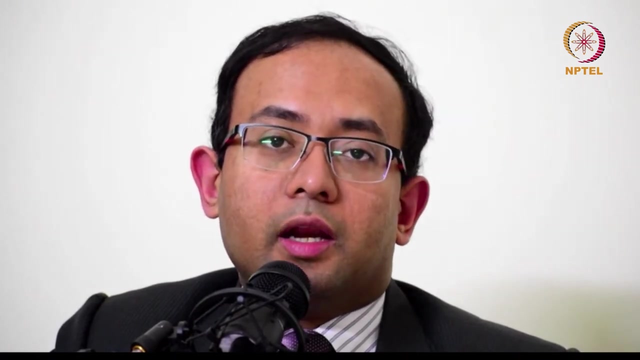 then we are talking about a runoff. Now, this runoff can occur on the surface, So when rain falls on the ground, it moves through various channels, It enters into a stream and then it begins to move out towards the oceans or towards an inland lake. 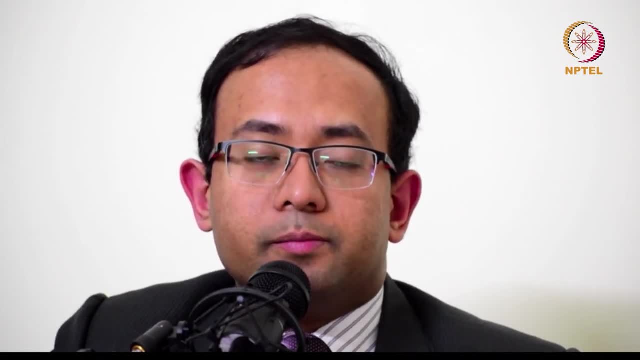 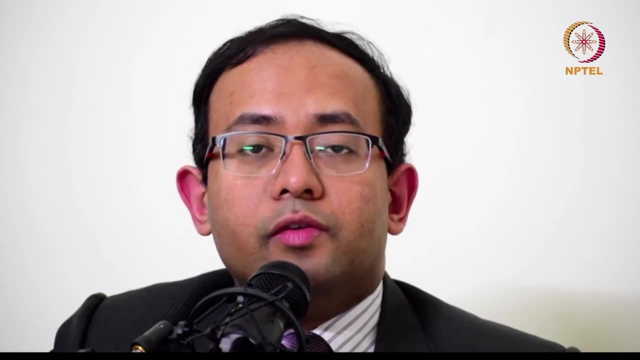 Now these movements are known as surface runoffs. We can also have subsurface runoffs and we can also have a ground water runoff. Now, ground water runoff refers to a situation where the ground water is moving into the streams. So essentially what is happening? 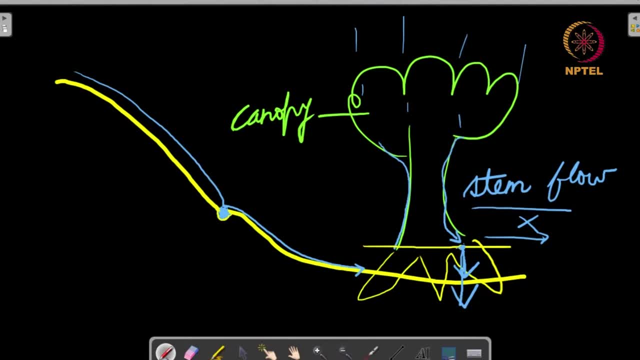 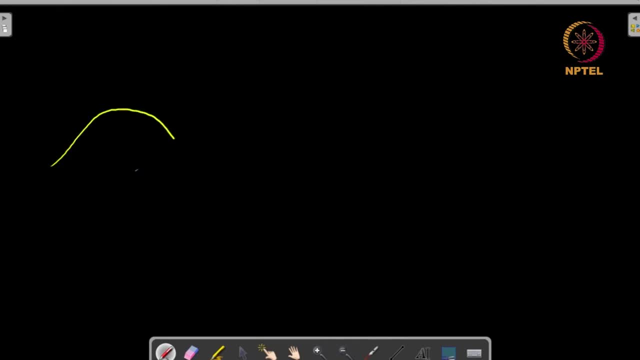 is that it is an opposite process to that of infiltration. So you have this. So suppose this is the land and here you have a stream, say a river, But suppose the ground water is at this level. So in that case, some amount of water. 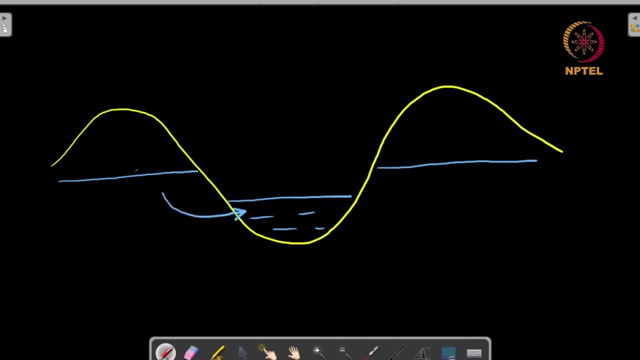 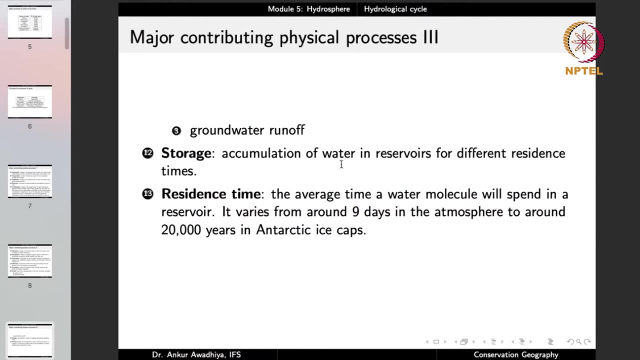 will begin to flow from the ground water into the streams And then it will begin to move away from this drainage basin, So this is known as a ground water runoff. Then we also have storage, which is accumulation of water in different reservoirs for different residence times. 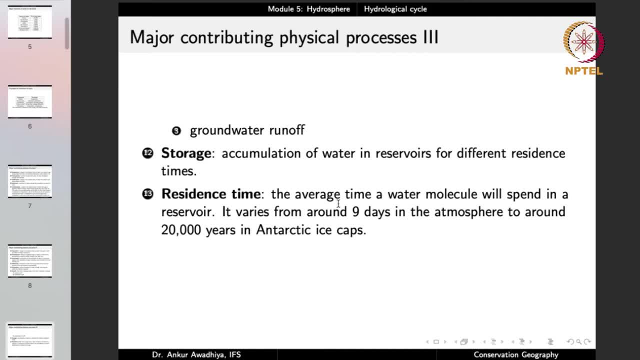 Where residence time is the average time a water molecule will spend in a reservoir, which varies from around nine days in the atmosphere to around 20,000 years in the Antarctic ice caps. So this is the average time a water molecule will spend in a reservoir. 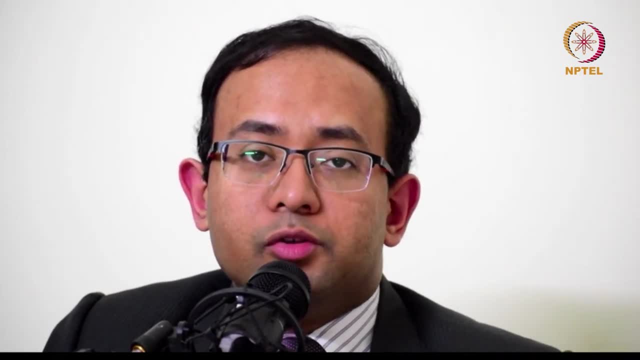 Now we have talked about different reservoirs, such as oceans or atmosphere, or ice caps or ground water, And when we talk about the residence time, what is the average time that a water molecule will spend in the reservoir once it has entered into this reservoir? 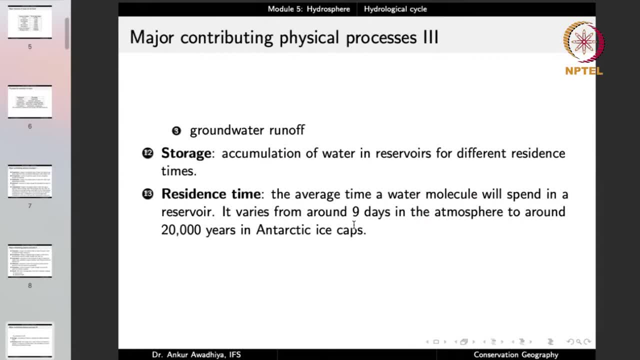 So the residence time can be as low as nine days in the atmosphere. So on an average, a water molecule stays in the atmosphere for only nine days, After which it gets condensed or it gets precipitated or deposited somewhere to around 20,000 years. 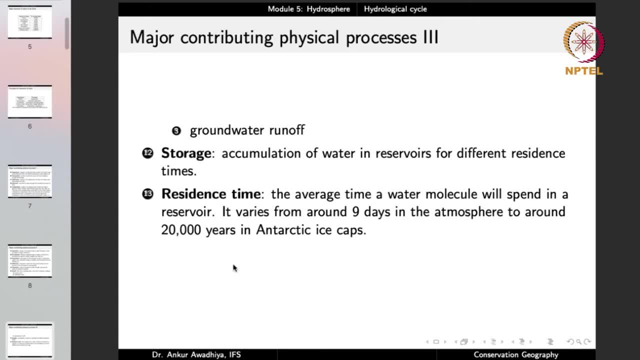 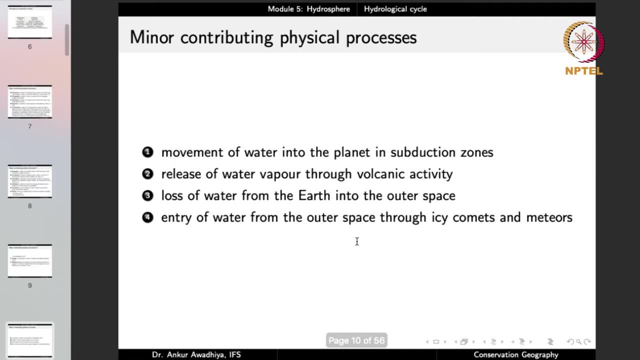 in the Antarctic ice caps. So if a water molecule has entered into the Antarctic ice caps, it can expect to stay there for around 20,000 years. Now, apart from the major processes, we also have certain minor contributing physical processes, such as movement of water. 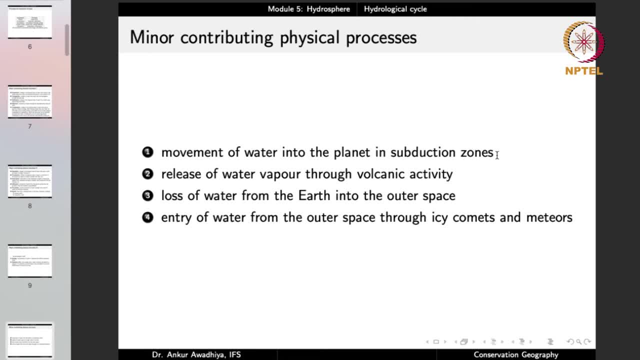 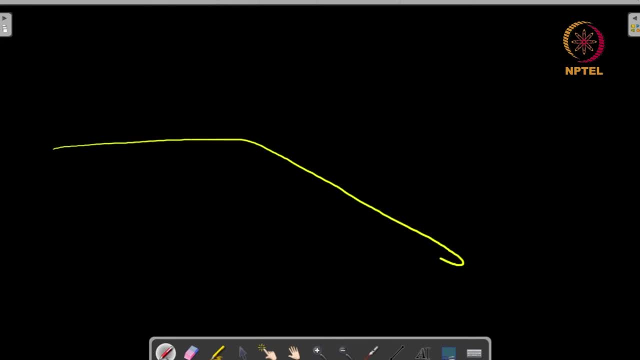 into the planet in the subduction zones. Now, you will remember that a subduction zone is an area where two plates are colliding and one of the plates is moving below another plate. So this is a region of convergence. Now, in this convergence, typically, if you have, 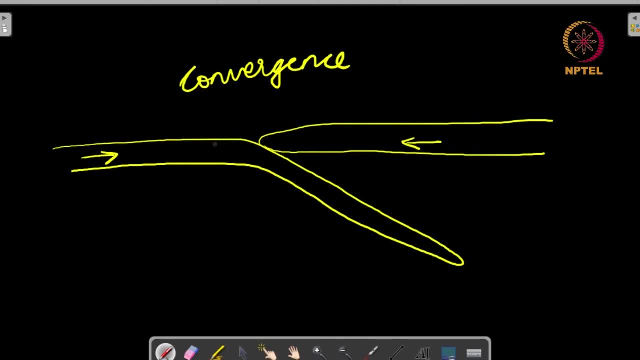 a convergence of, say, an oceanic plate with a continental plate, then the oceanic plate will move down And when it moves down, the water that was here in this plate it is also moving down. So this is a process through which water from the crust 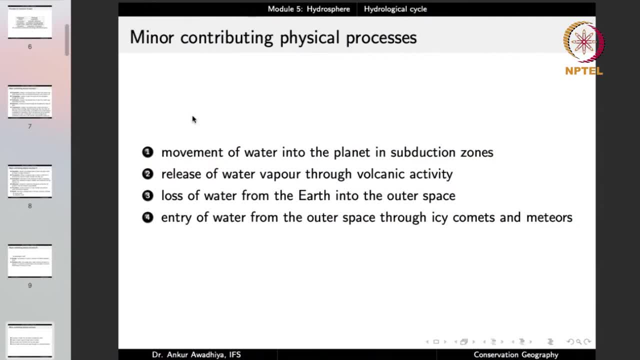 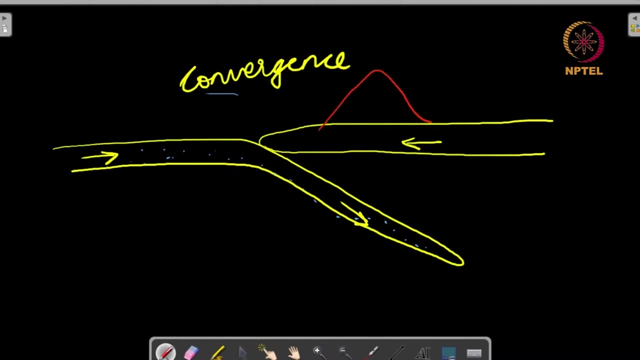 is moving into or towards the mantle. So this is a minor contributing physical process. Or another process is the release of water vapor through volcanic activity, And we had observed here that in most of the cases we find volcanoes in this region which spew out. 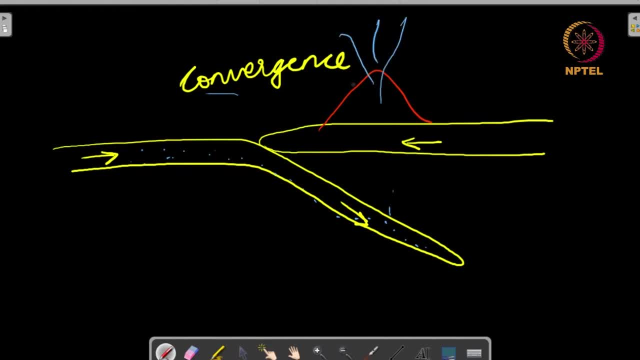 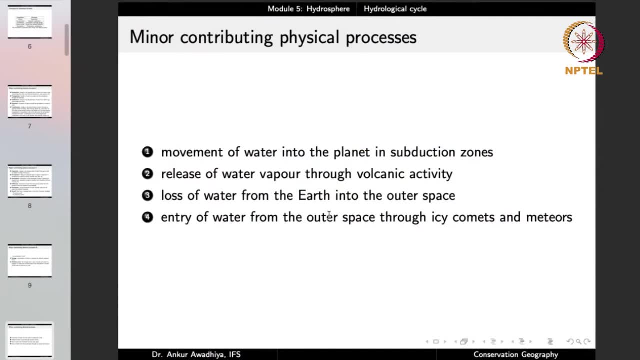 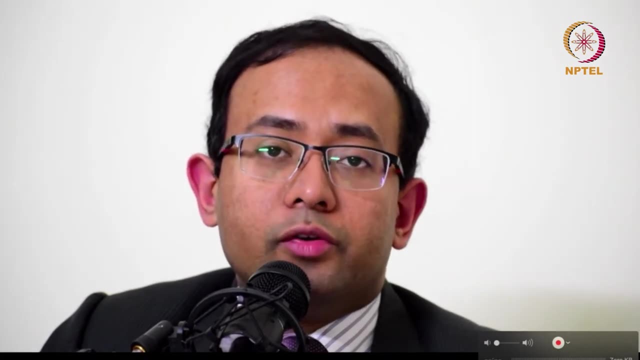 this water in the form of water vapor. So this is another activity that is happening. Then we have loss of water from the earth into the outer space. So when water is moving up in the atmosphere, a part of it can also get lost into this space. 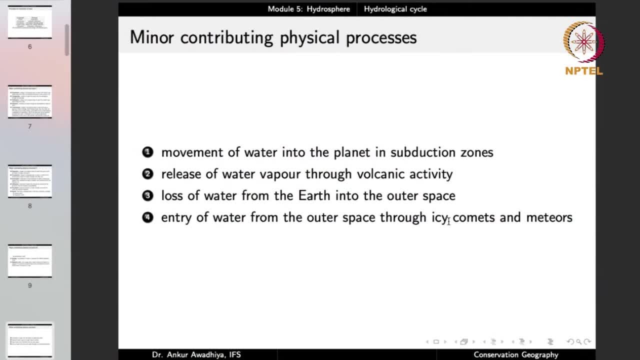 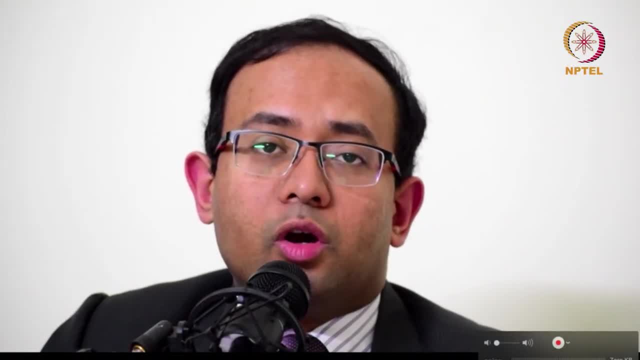 Or some water may enter into the atmosphere through things like icy comets and meteors, So these processes also happen, but by and large, when we talk about the hydrological cycle, these are very minor processes, So very small amount of water is moving through these mechanisms. 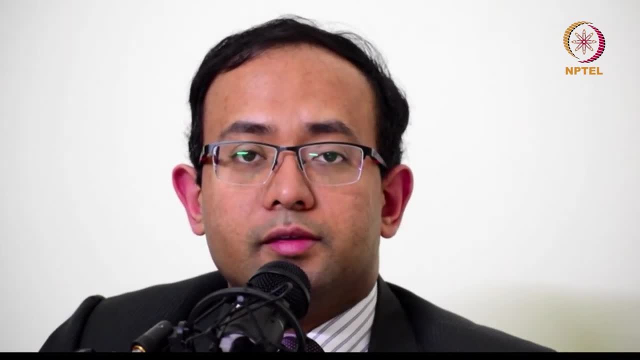 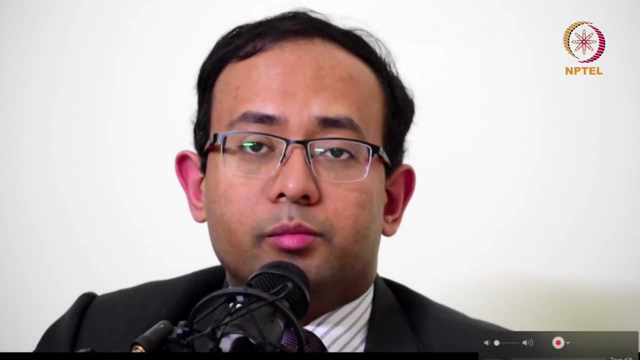 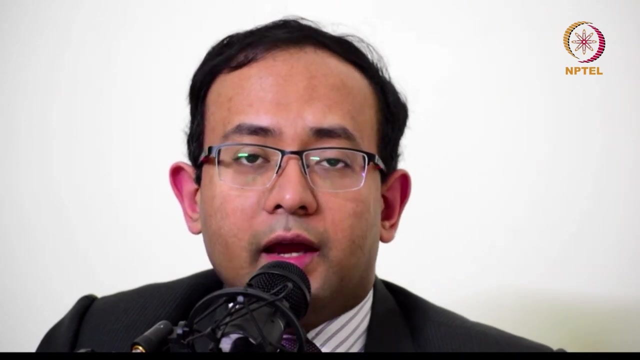 But it is important to note that these mechanisms also do exist. Now, when we talk about condensation, condensation can happen in a number of forms. So we can have condensation in the form of clouds, in the form of dew, in the form of haze. 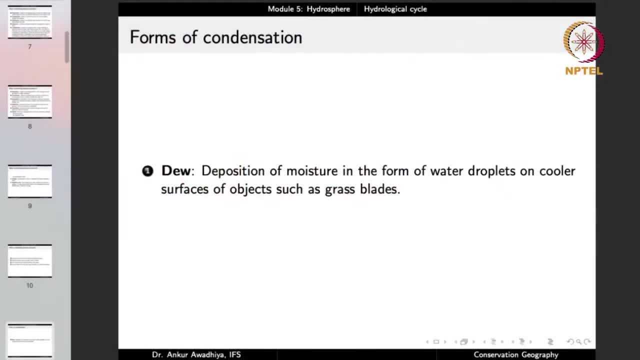 in the form of mist and a number of phase. So let us now explore some forms of condensation. The first one is dew. Dew is the deposition of moisture in the form of water droplets on cooler surfaces of objects such as grass blades. 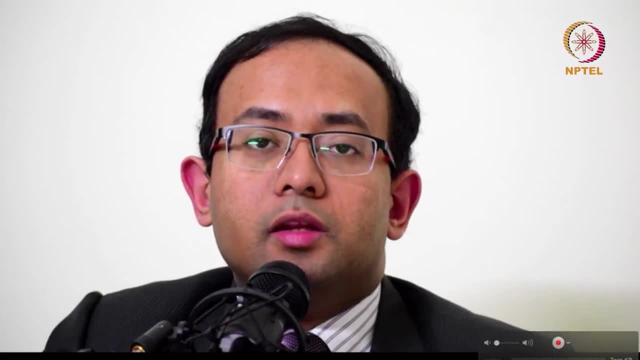 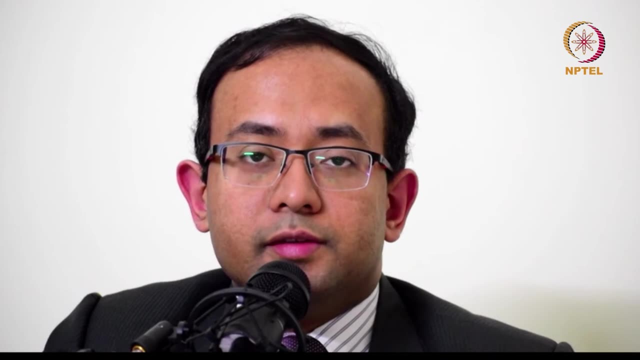 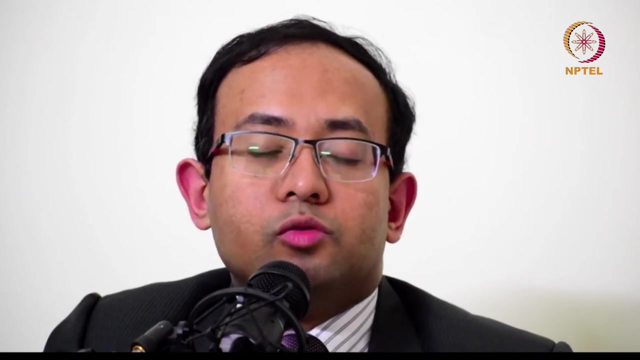 And you will typically observe dew formation in the winter months. So if you go out early morning in a winter month, you will find that on the cooler surfaces, such as grass or such as, say, the bodies of vehicles, you will find very small droplets of water. 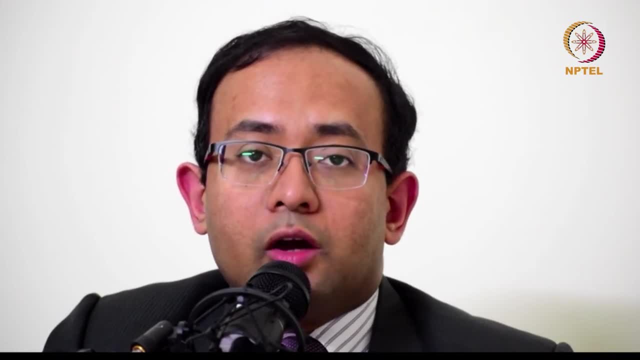 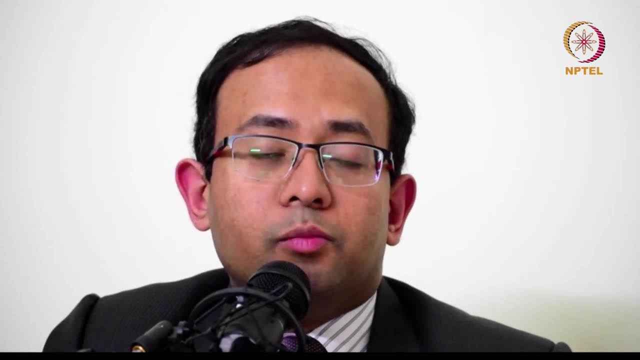 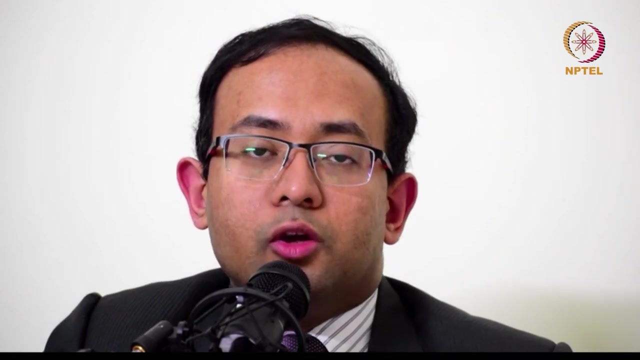 Now, in this case, because these surfaces are cold, the air that is near these surfaces, it crosses the dew point, At which point it becomes super saturated and it begins to shed out in the form of moisture, in the form of liquid water. So that is dew. 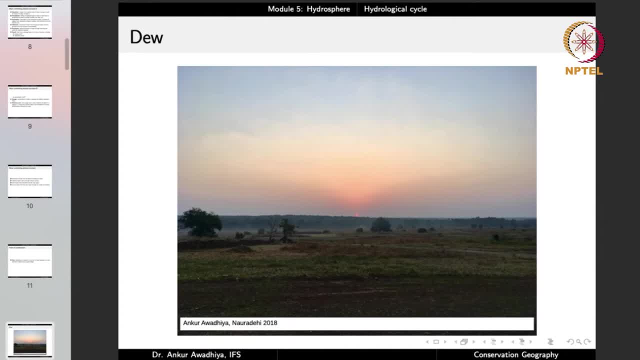 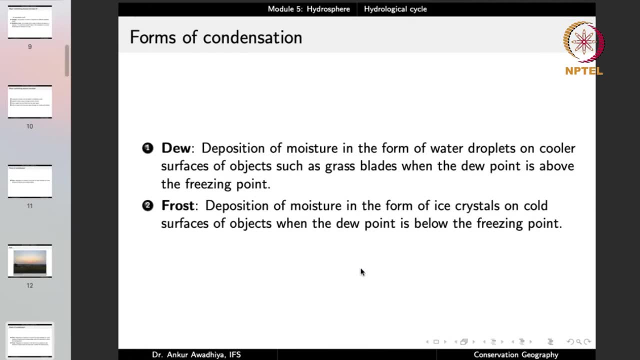 So typically you will observe dew in the case of early mornings, especially in the winter months, on things such as grass blades. Another is frost. Frost is the deposition of moisture in the form of ice crystals on cold surfaces of objects when the dew point is below the 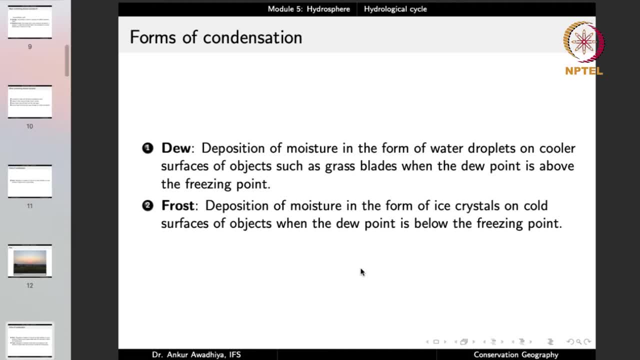 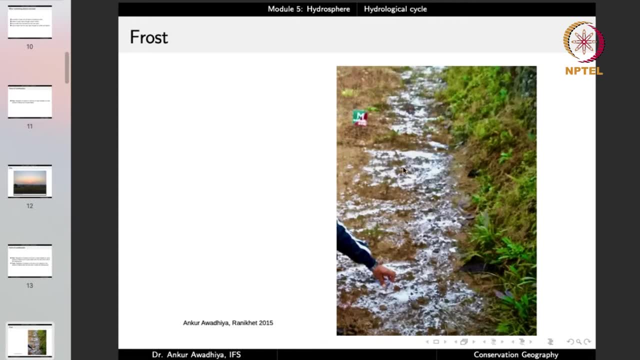 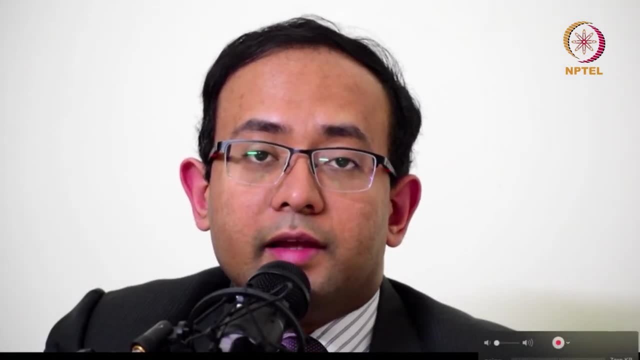 freezing point. Now, in this case, the water directly goes below the freezing point in the form of ice crystals. So this is how a frost looks like. So you will find that you have ice deposits on the soil, and this typically happens when the dew point. 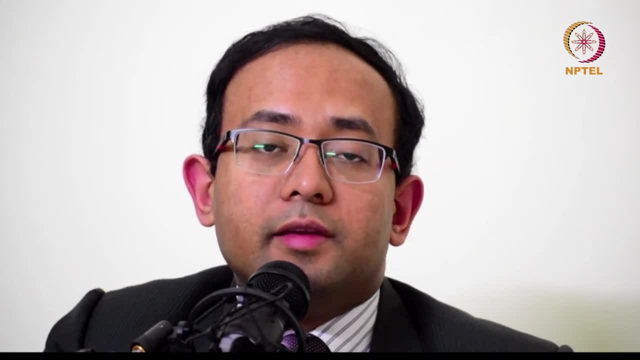 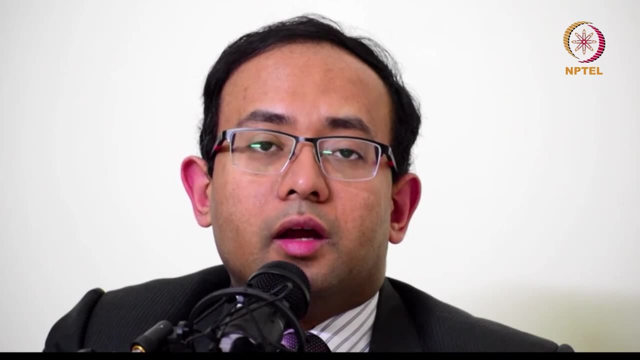 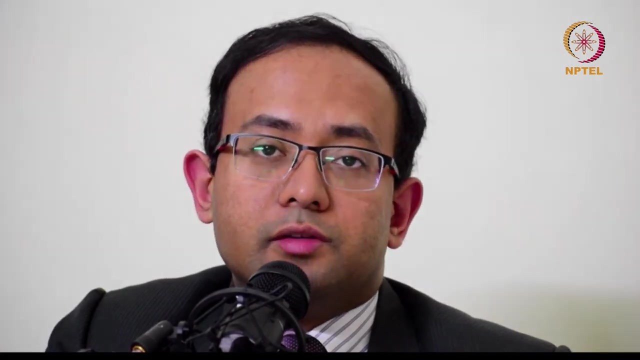 is so less or is at a so little temperature that it is less than the freezing point of water. So the air is able to hold the moisture till it is deposited in the form of ice crystals. Next we have fog, mist and haze, which is 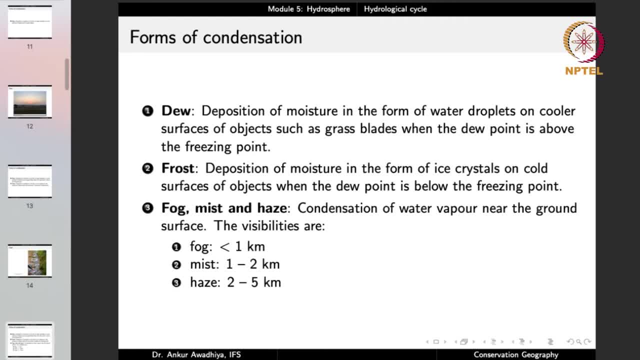 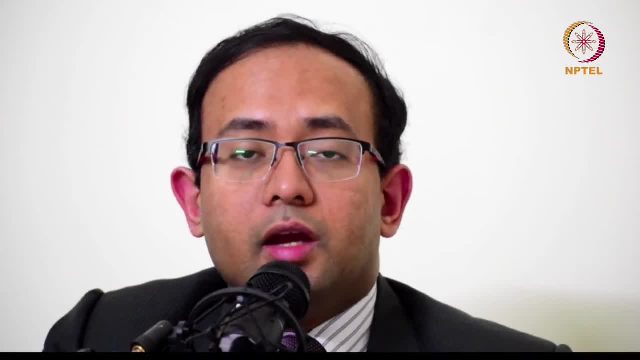 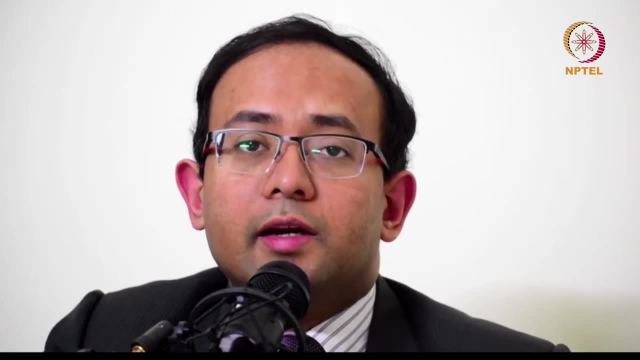 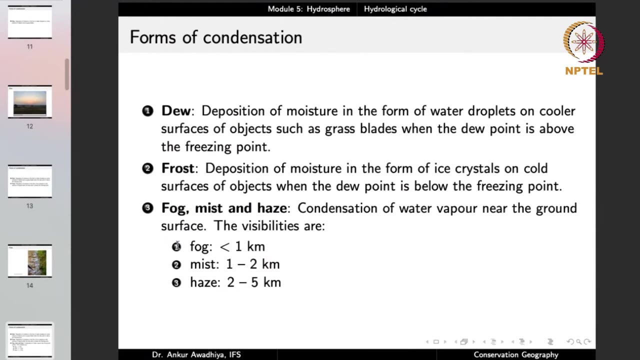 condensation of water vapor near the ground surface And this typically happens very similar to the formation of clouds. So in this case the water condenses in the dust particles, or say pollen grains or smoke particles very near the ground surface. So, depending on the visibility, 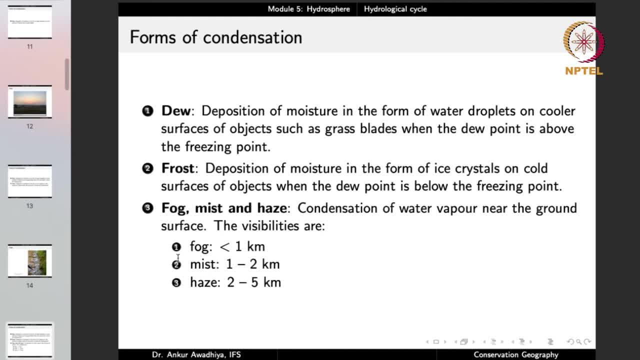 if the visibility is less than 1 km, we call it a fog. If visibility is between 1 to 2 km, we call it a mist. If visibility is between 2 to 5 km, we call it a haze. So this is condensation. 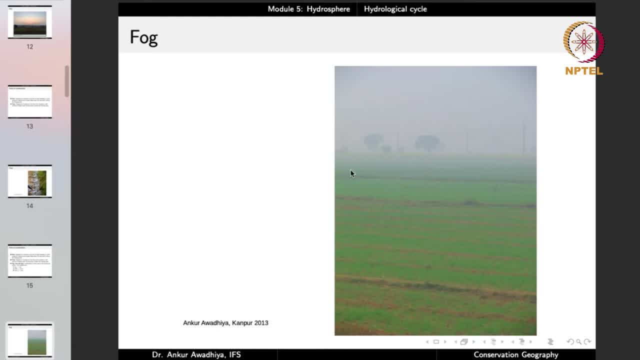 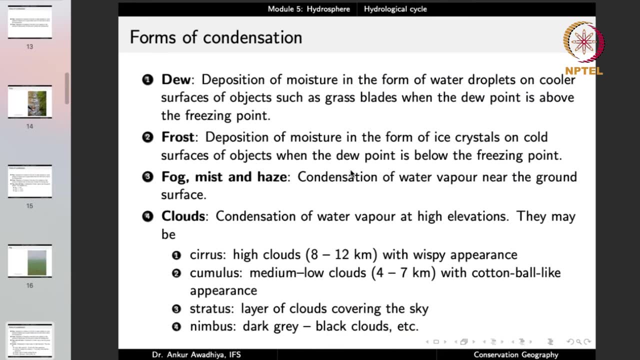 of water vapor near the ground surface but not on the ground surface. Next, we have clouds, which is condensation of water vapor at high elevations in the atmosphere, And you can have different kinds of clouds. So we have cirrus clouds, which are high clouds. 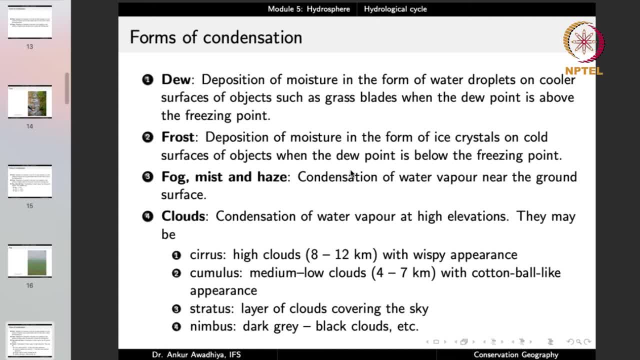 at a height of 8 to 12 km with a wispy appearance. Cumulus is medium low clouds- 4 to 7 km, with a cotton ball like appearance Or a large portion of the sky, And you also have nimbus, which is 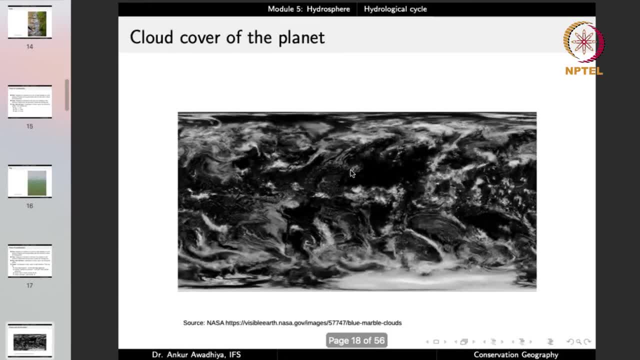 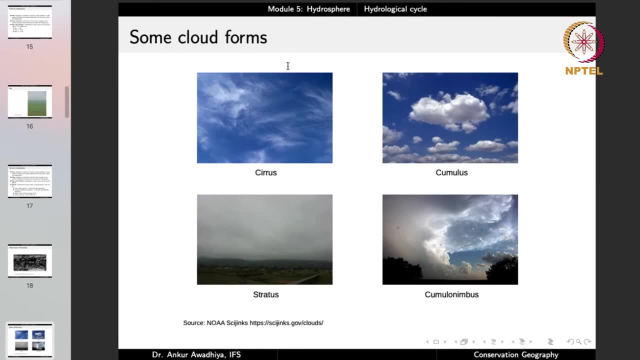 dark, grey to black coloured clouds, Typically the clouds that bring rain. So this is, if we look at the cloud cover of the planet. this is what it looks like. So you can observe that we have a horse's tail, So they have a wispy. 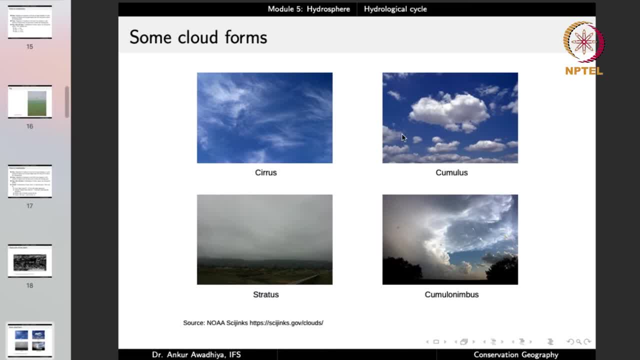 appearance. Then you have cumulus clouds. They look like cotton balls. They are at a middle altitude. You have stratus clouds which cover the whole of the sky And you have nimbus clouds, which have nimbus clouds, Or it can be. 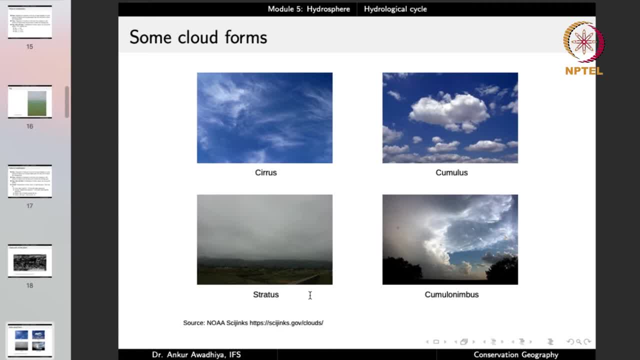 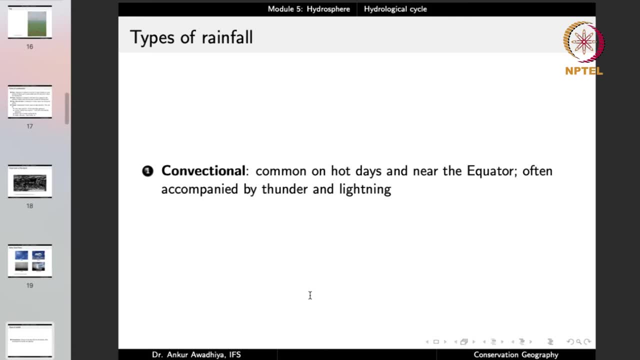 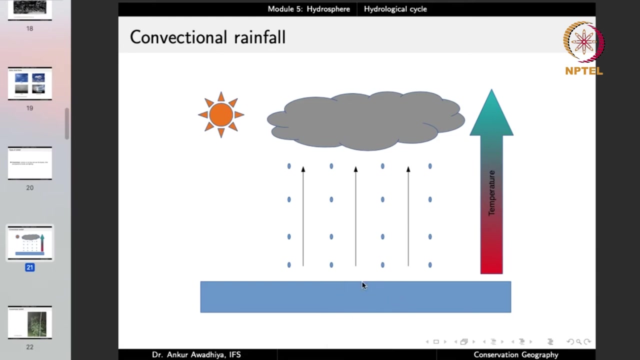 stratonimbus, which is covering the whole of the sky, but it is dark, grey or black in colour and bringing rains and so on. And when we talk about rain, there are different kinds of rains. We have convectional rainfall, which is common with water. 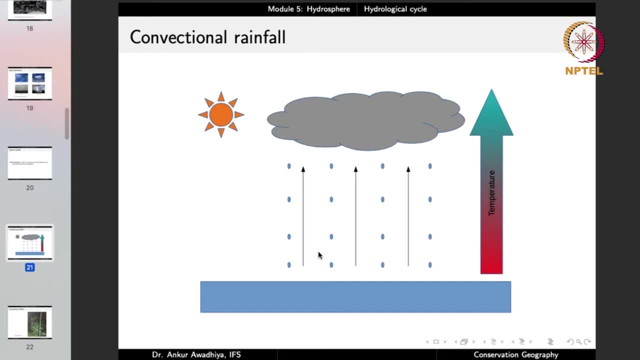 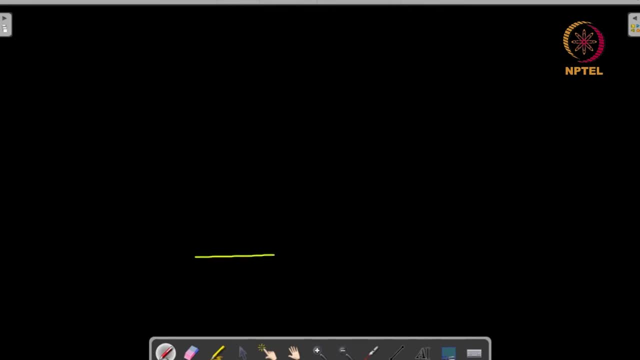 vapour. It moves up through the convectional currents that get set up. Now, what we are talking about is that once you have a surface, probably the surface also has some amount of water or some amount of water. So what we are talking about 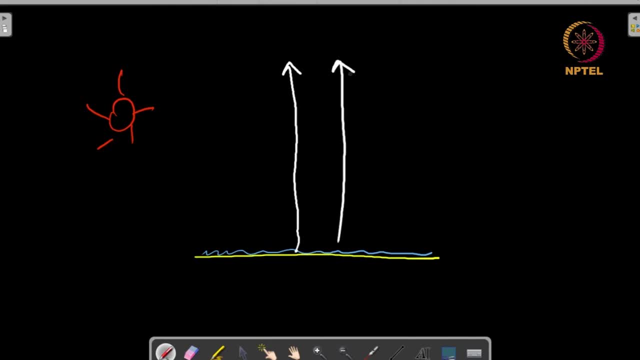 is that the air here is warmer and so it becomes less dense and it rises. So you have a movement of air upwards And along with this air, the water vapour also moves up. When it condenses, it forms clouds in this area, And when 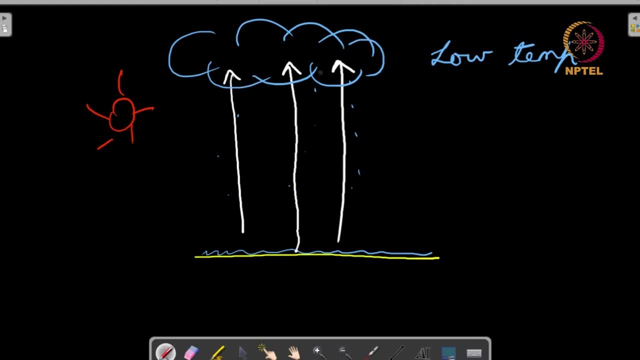 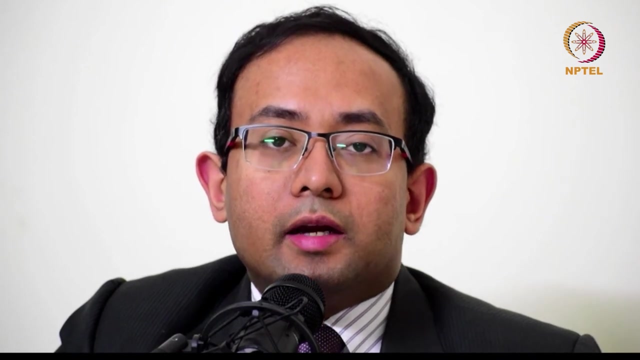 the clouds get formed, and when you have a lot of moisture that is moving into the clouds, the air becomes super saturated and then it starts to condense here. So essentially in the morning times and in the evening, at that time the clouds will begin to give out. 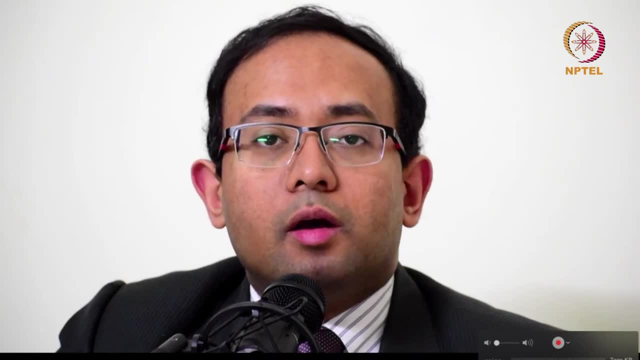 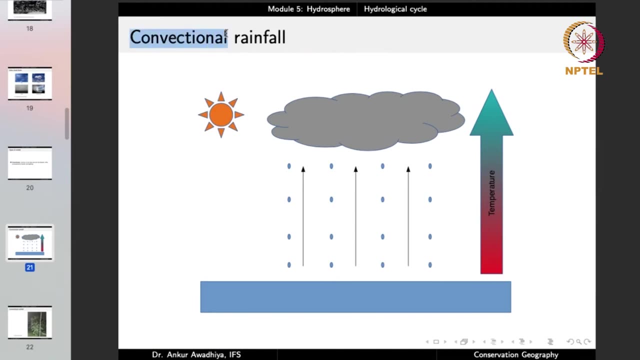 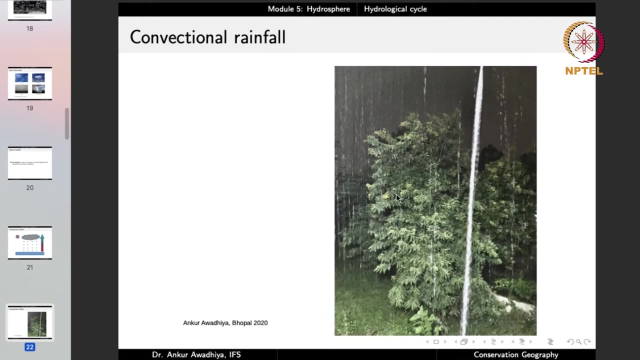 rain, And so you will have a very intense amount of rainfall, often accompanied by thunder and lightning. So that is convectional rainfall. It is powered by the rain, and often this convectional rainfall is a very intense rainfall. So here in this, 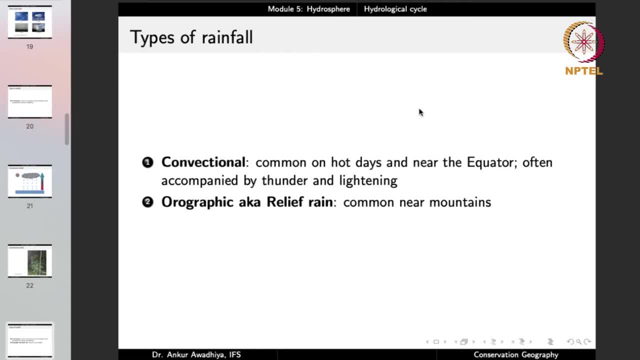 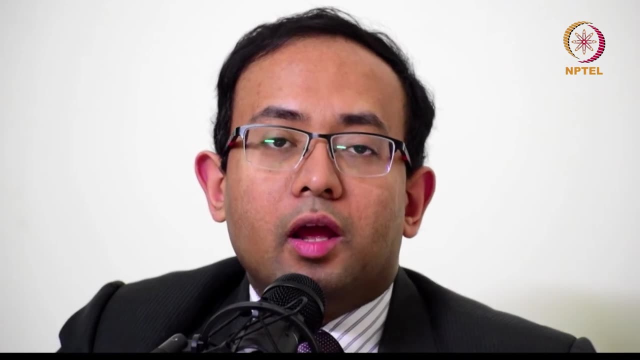 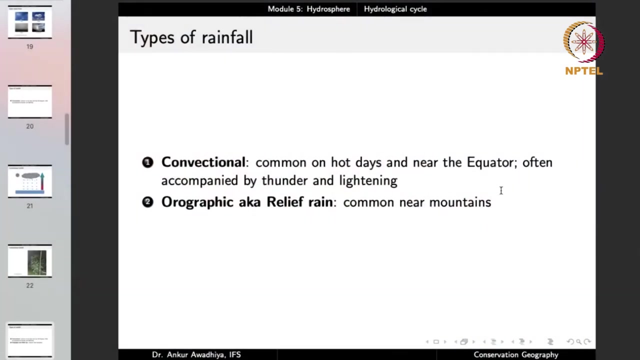 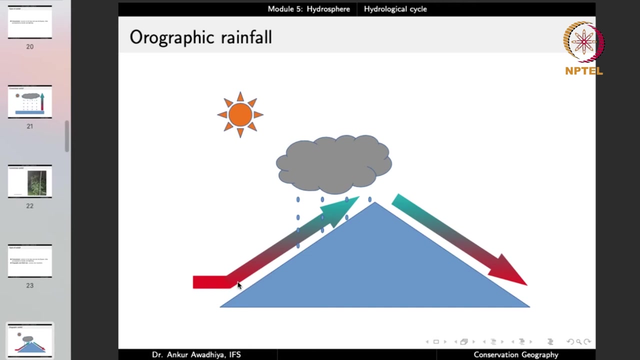 picture, you can see that there is a very intense amount of rainfall that is occurring. Another rainfall is the orographic rainfall, or the relief rainfall. Now, in this case, the rainfall is common near the mountains, And what happens is, when you have a wind, that 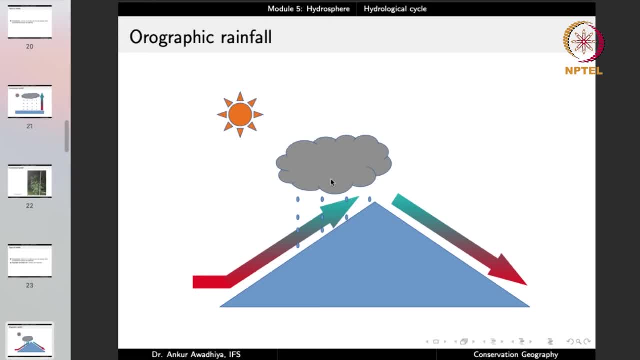 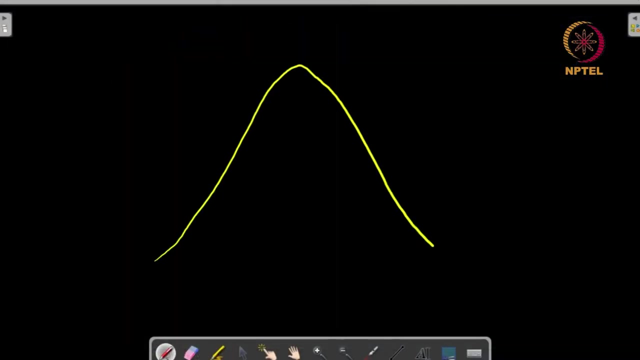 is blowing towards the mountains. when it reaches the mountains, it typically gets warmed, and so you will have a heavy rainfall on this portion, but not any rainfall in this portion. So if this is the wind direction, if you have a mountain like this, and if the wind 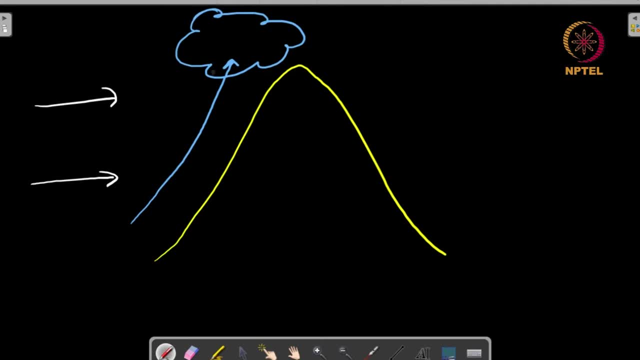 moves in this direction, you will have an upward movement, and when it moves down on the other side of the mountain, it gets warmed, And when it gets warmed there is no further rainfall on this side. Now the left side that is facing the winds is known. 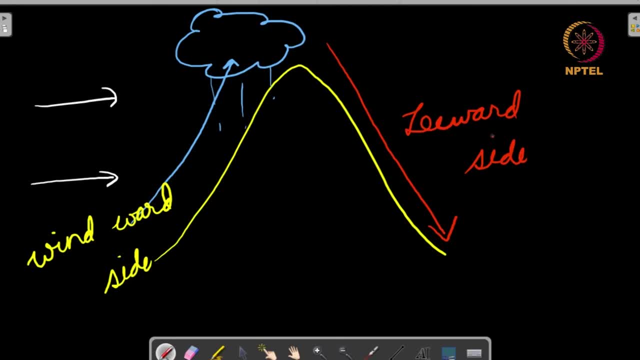 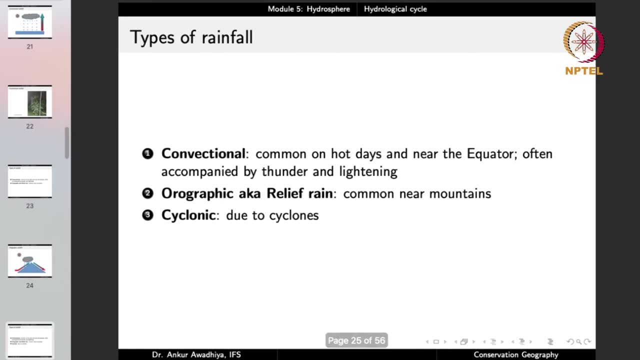 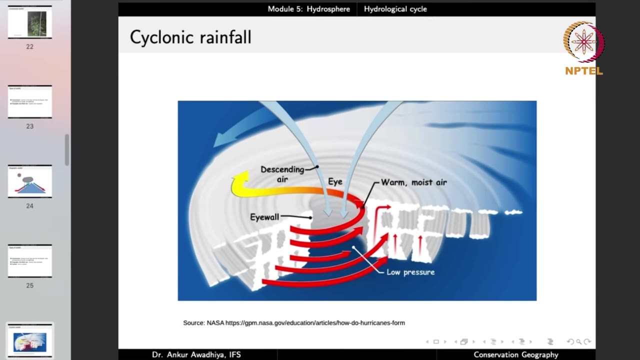 as the winds and very little rainfall on the other side, which is the leeward side. So this is the orographic rainfall. Third, we also have cyclonic rainfall. that occurs with the cyclones and we had observed that in the case of cyclones, you have 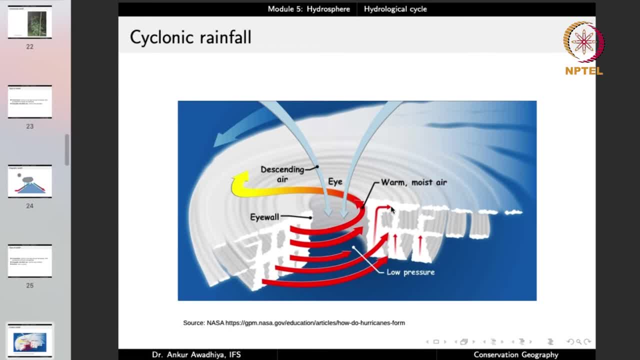 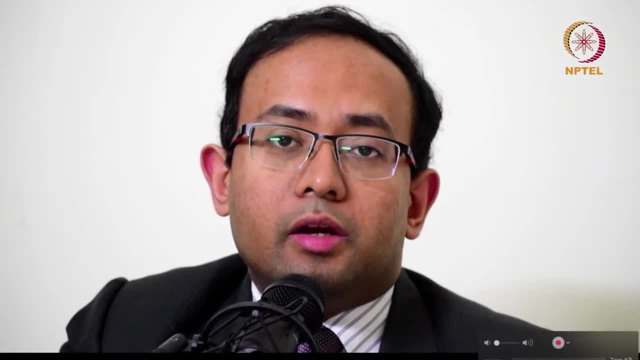 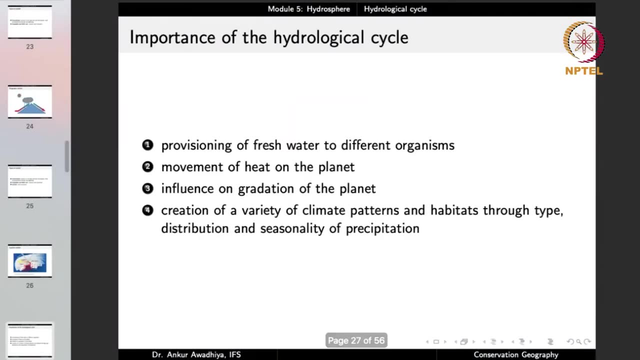 a very rapid movement, and this rainfall is only associated with the cyclones, and so this is known as the cyclonic rainfall. So these are the three major rain types You have convectional rainfall, orographic rainfall and cyclonic rainfall. So what? 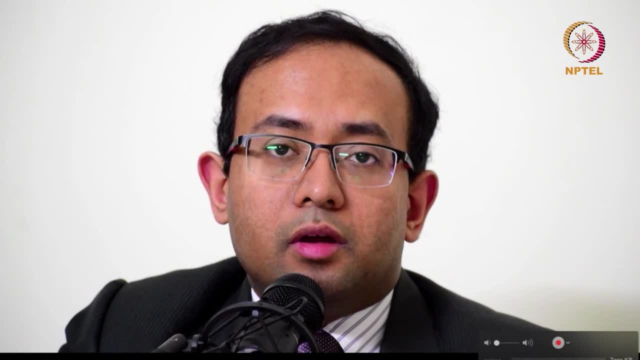 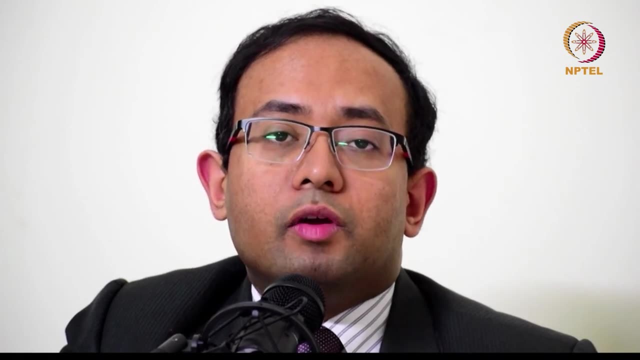 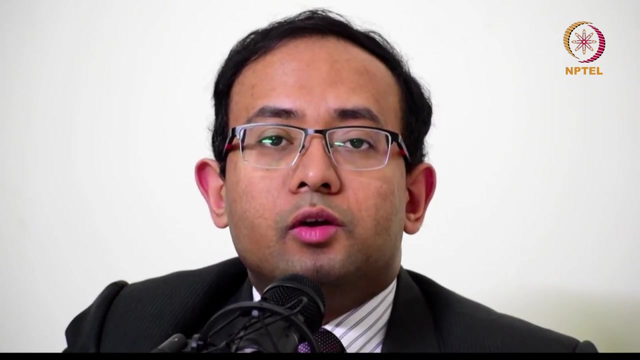 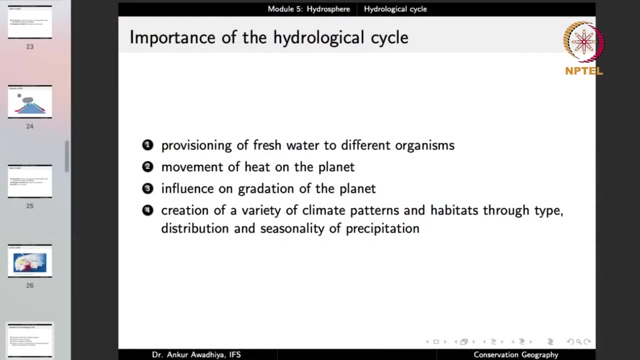 is the importance of the hydrological cycle? Well, it provides water bodies. If we did not have the water cycle, then where would they get the water from? Because of the hydrological cycle, the water from the oceans is being moved into the land areas and 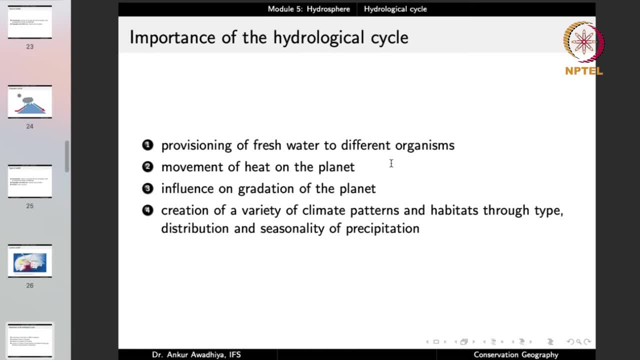 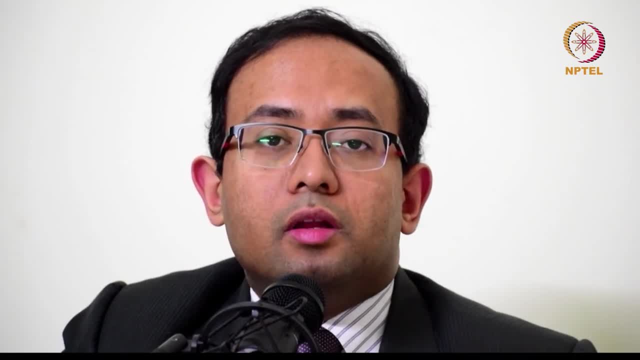 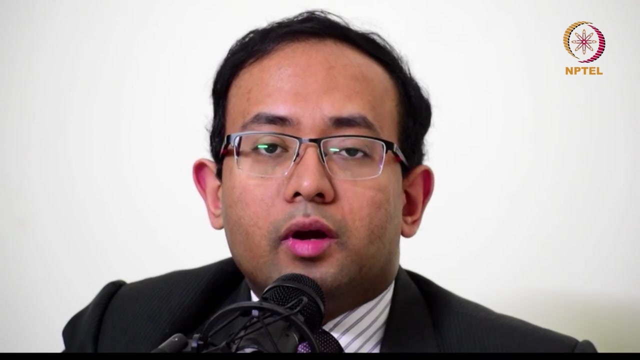 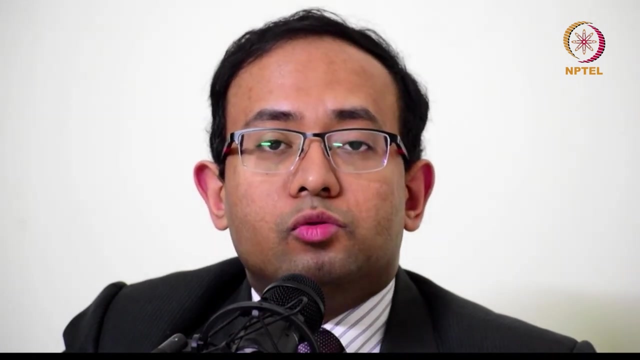 so the hydrological cycle in a way sustains all the life on this planet, or most of the life on this planet. So the hydrological cycle is the cycle of water moving from the ocean to the ocean. So the hydrological cycle is the cycle 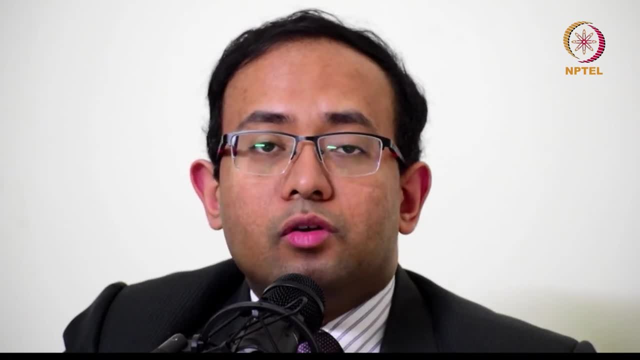 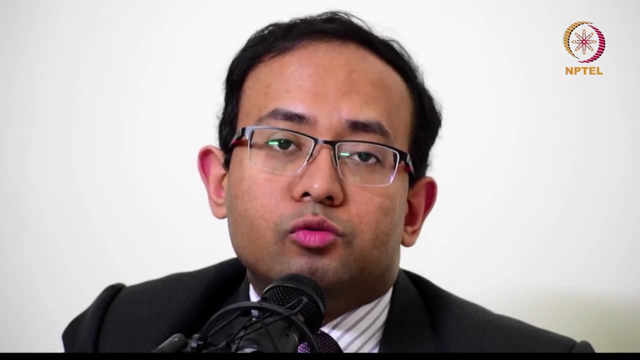 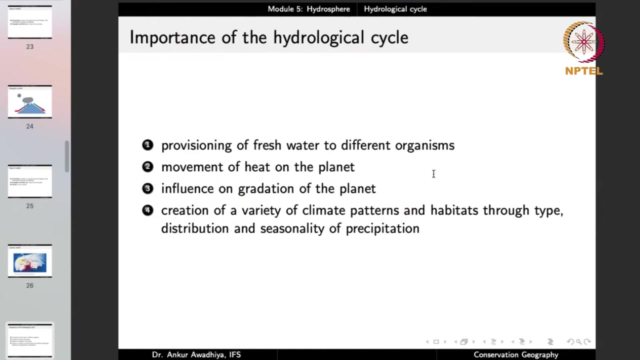 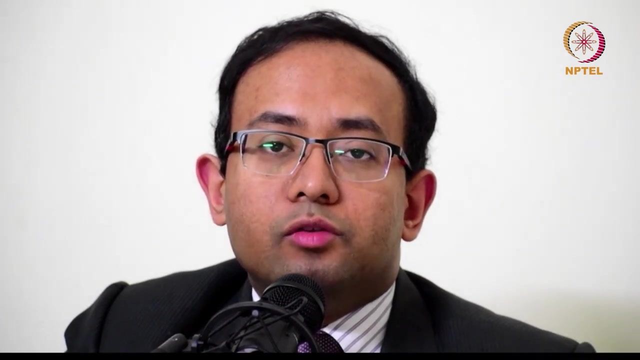 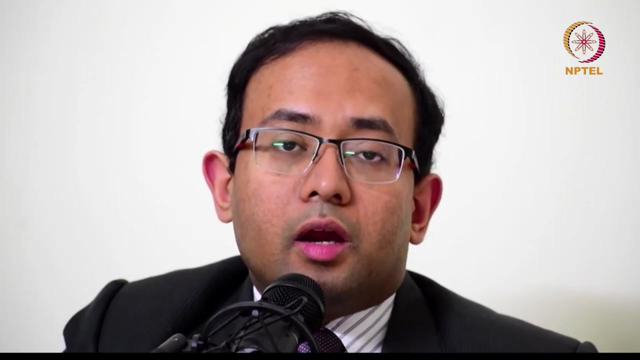 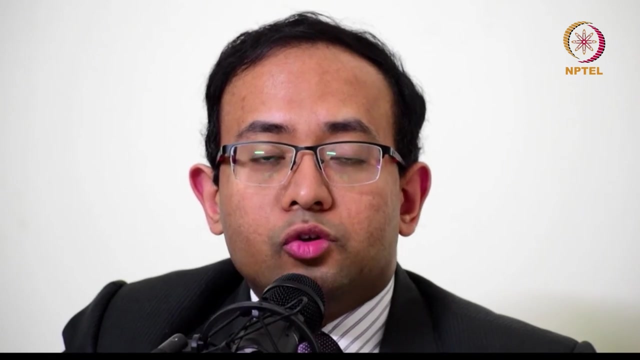 of water moving from the ocean to the land areas. So the hydrological cycle is the cycle of water moving from the ocean to the land areas. So the hydrological cycle is the cycle of water moving from the ocean to the waters and also near the 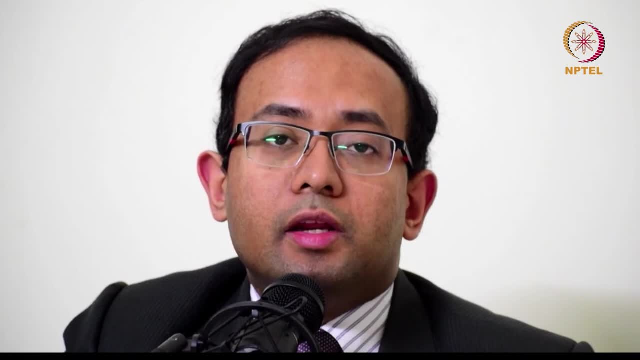 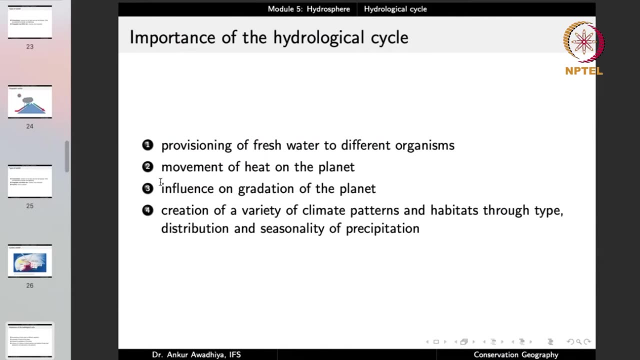 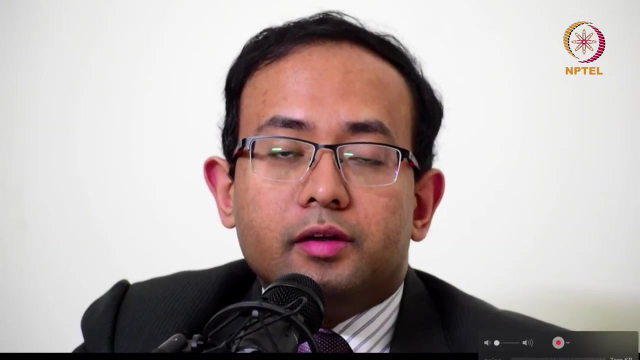 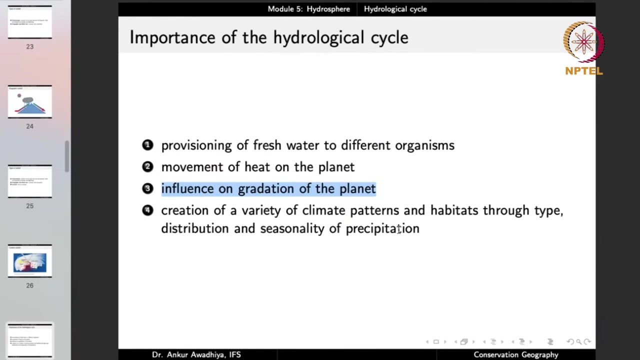 deltas. So in a way it is playing a role in the gradation of the planet. It is a very important geomorphological agent. So this is another importance of the hydrological cycle. It plays a role in influencing the gradation of habitats. 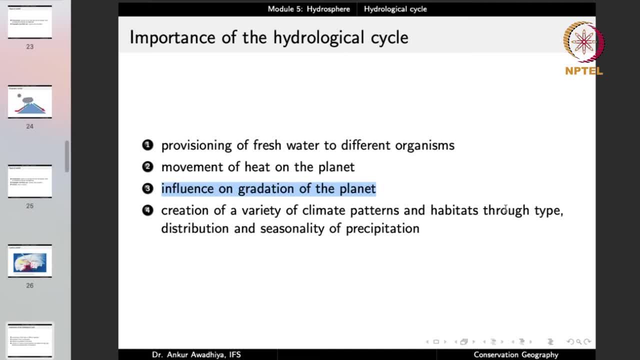 through type distribution and seasonality of precipitation, Type meaning that whether it is in the form of rains or it is in the form of snow, So if you have snowfall, there will be a very different habitat that gets created, full of ice and snow. 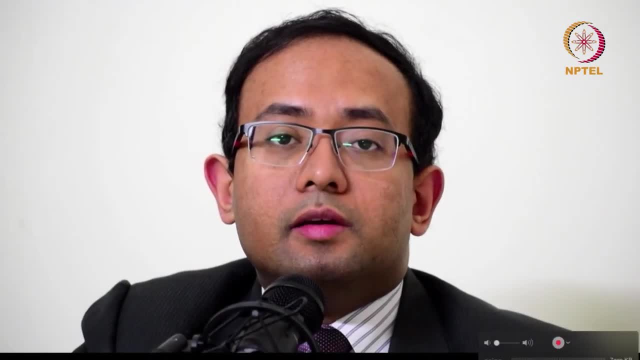 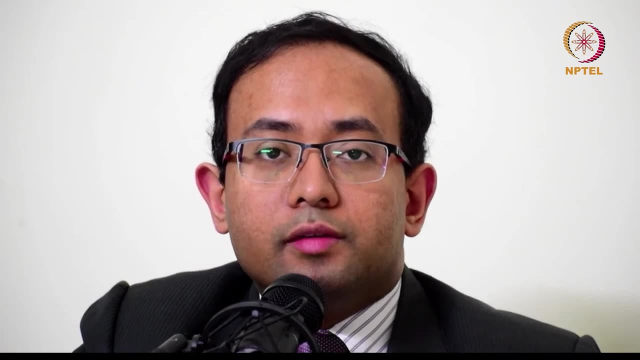 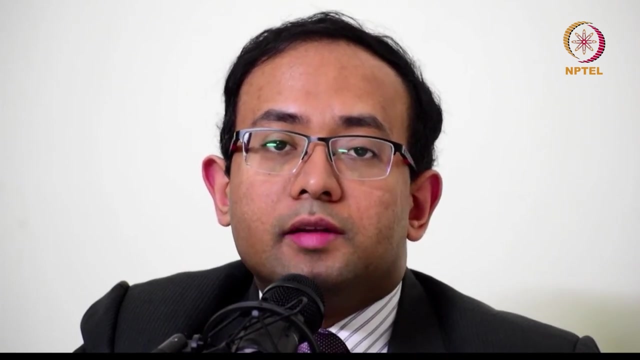 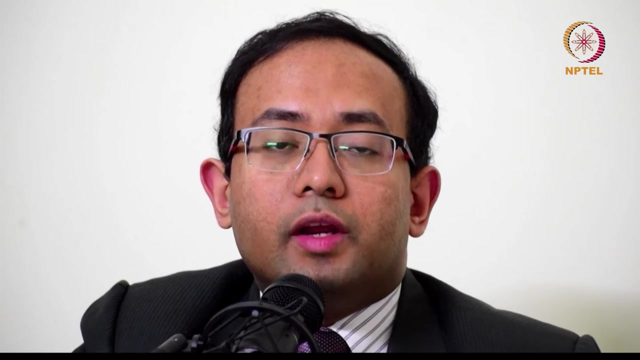 If there is rainfall, it is a very different climate. Say, tropical forests or equatorial rainforests, they get a heavy amount of rainfall. And those areas that do not get a large amount of rainfall, those areas that get a very scanty amount of rainfall. 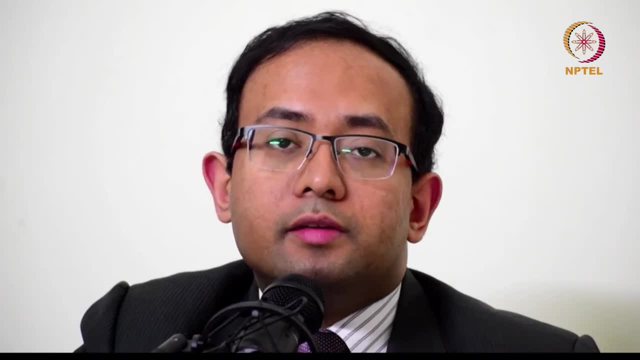 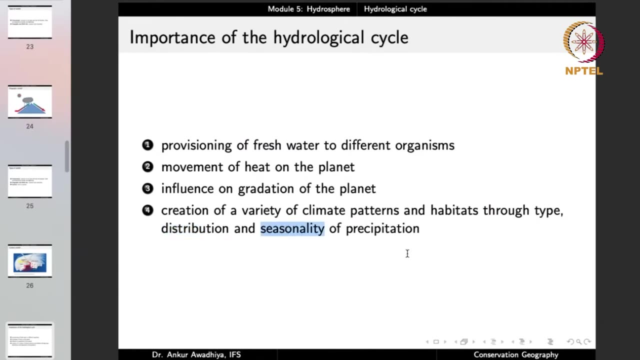 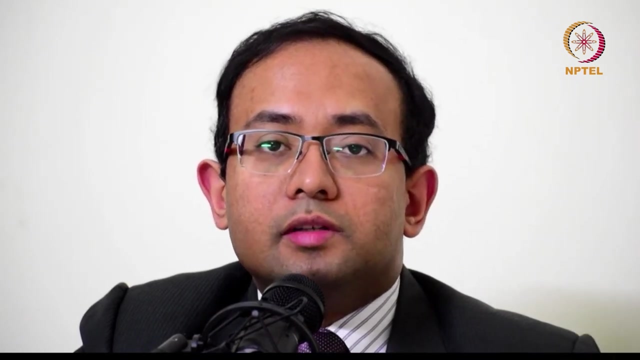 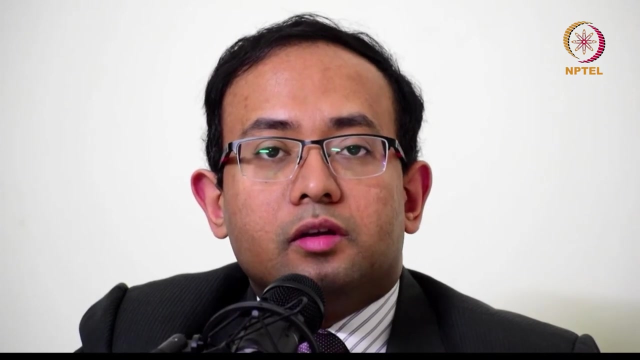 they become deserts, And so the distribution of rainfall means different habitats and seasonality of precipitation. So in certain areas you have lots of rainfall in a very short period of time, which results in a flood, like situation In other areas. the rainfall is distributed. 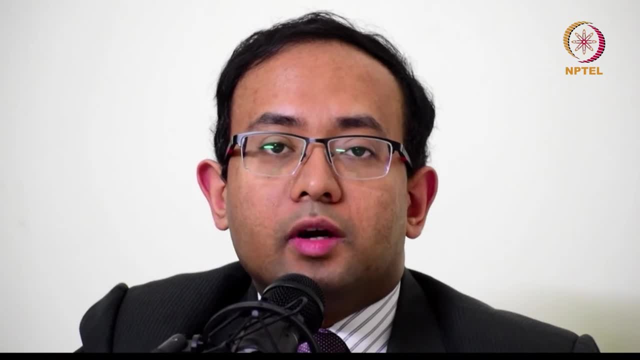 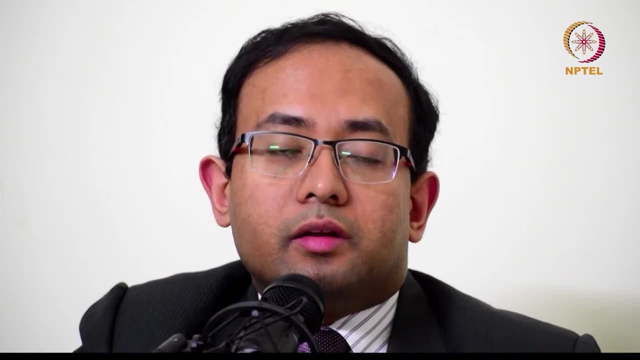 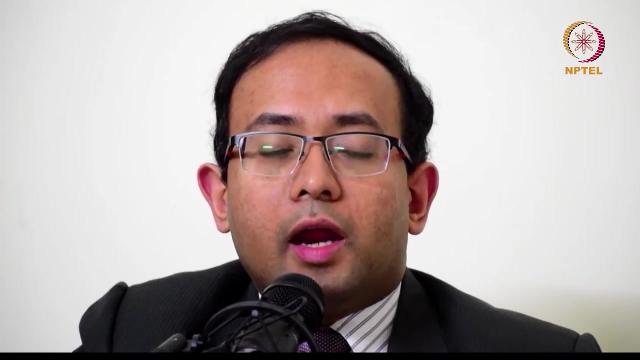 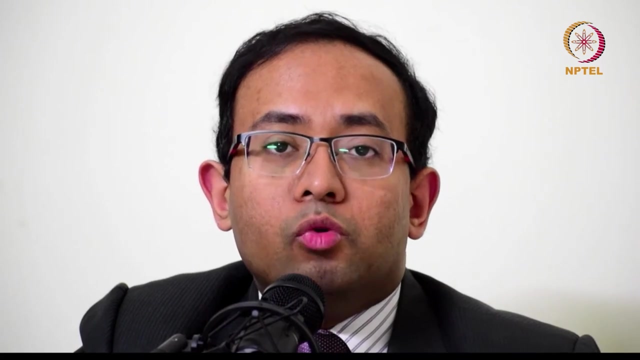 over a very large number of months, So the seasonality is different and in those areas you do not get that much rainfall. In other areas like marshes and the areas that do not receive floods are a very different habitat And so the type distribution. 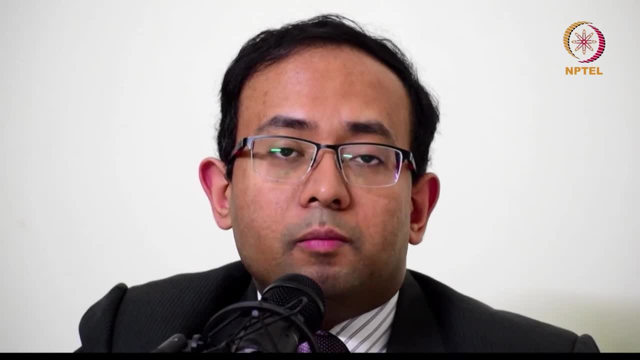 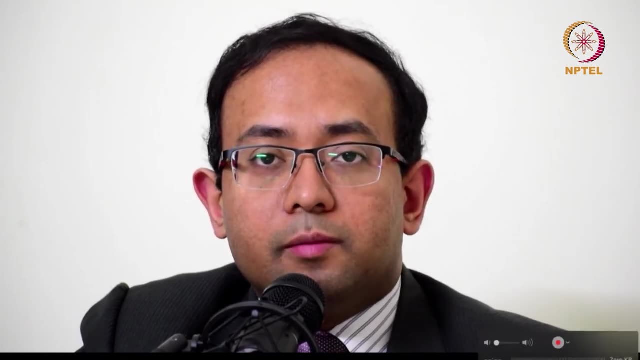 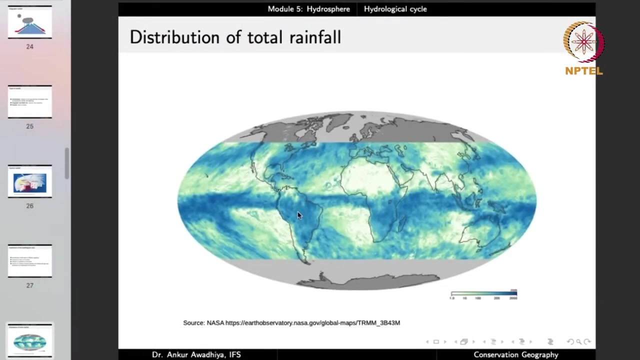 and seasonality of precipitation creates various forms of habitats. More the number of habitats, more will be the biodiversity. So the hydrological distribution is the distribution of the rainfall. If you look at the distribution of total rainfall, we will find that areas that are near 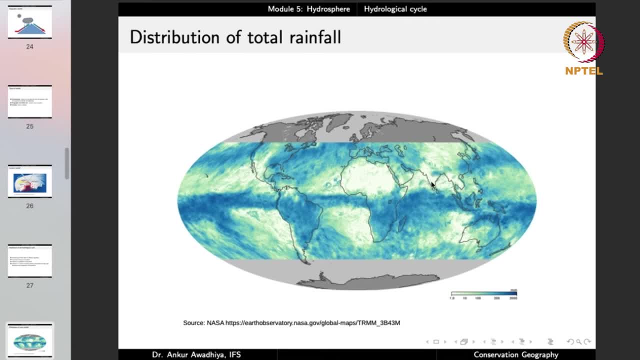 the equator, they get a very heavy amount of rainfall, Mostly convectional rainfall, And otherwise you have certain areas that get more amount of rainfall and certain areas in Africa, in Southeast Asia, we have a very heavy amount of rainfall And in those areas 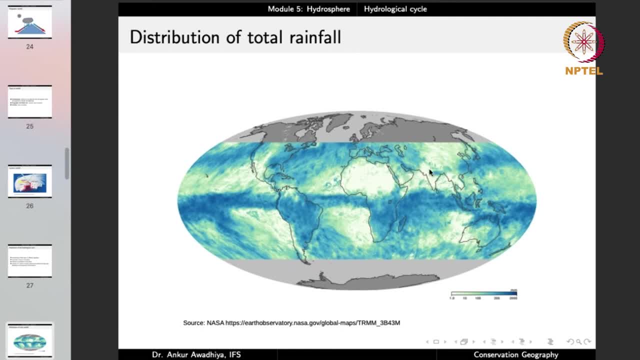 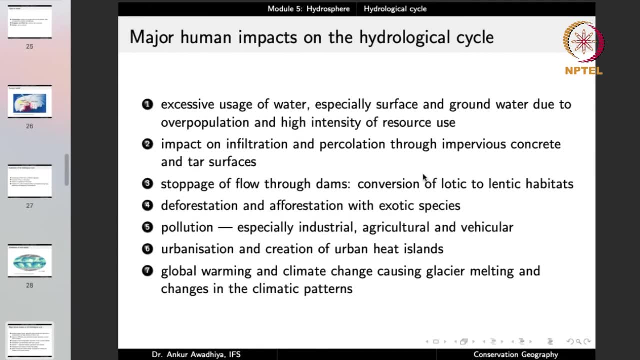 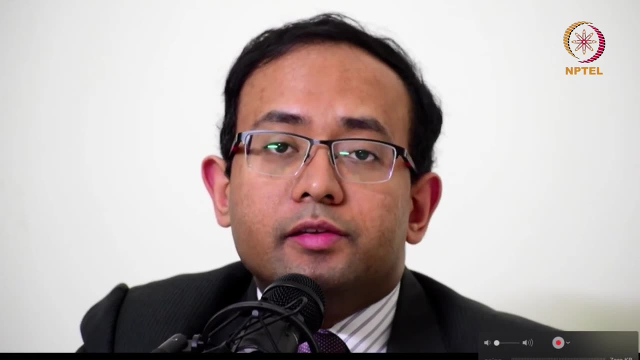 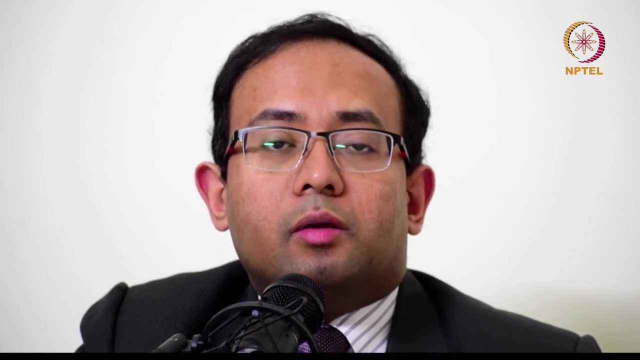 where we get less amount of rainfall, we have the deserts. So this is the Sahara desert, this is the Arabian desert, this is the Thar desert. So the distribution of rainfall is very high. So if you look at the geological cycle, you will. 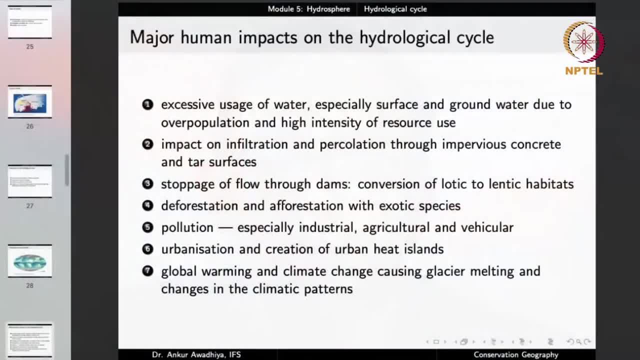 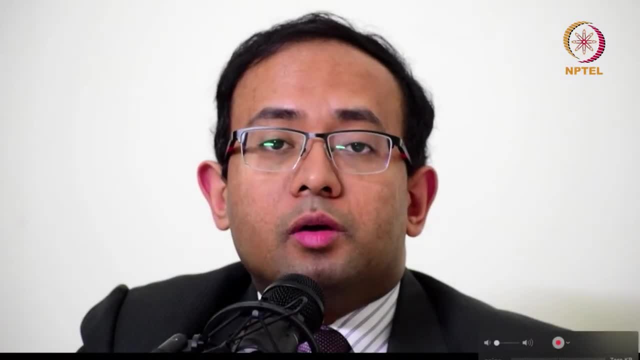 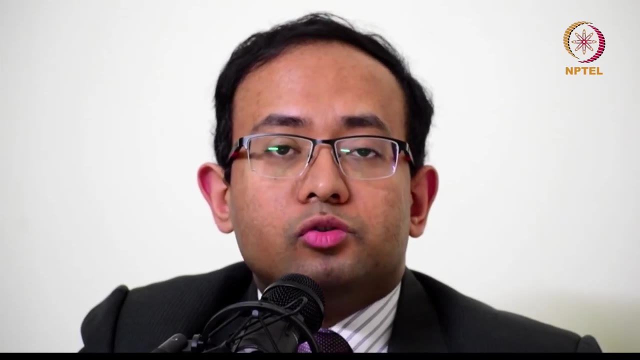 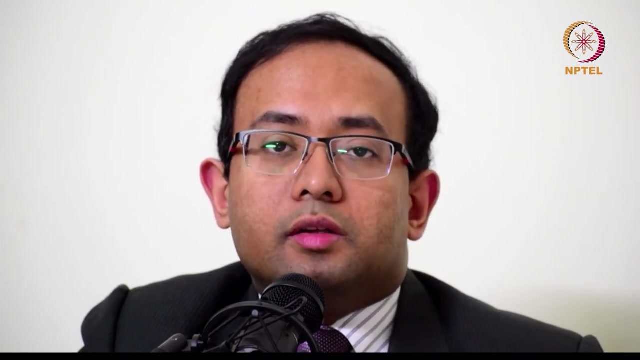 find that you have a very high amount of rainfall, And this is a very high amount of rainfall, So this is a very high amount of rainfall. The areas that were known for the lakes now no longer have those lakes because all that water has been used. 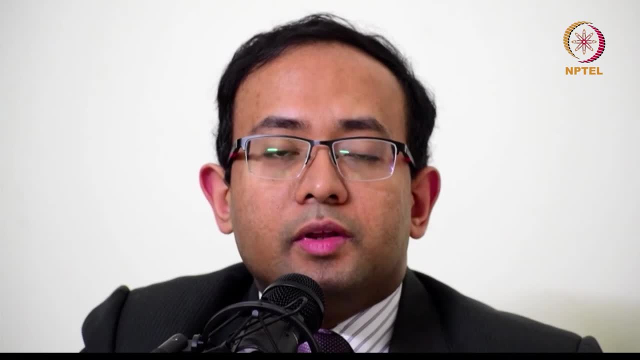 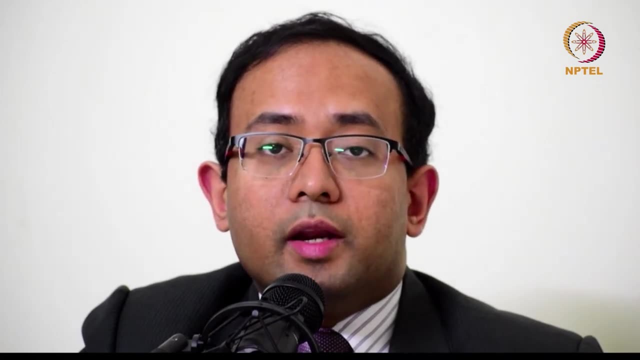 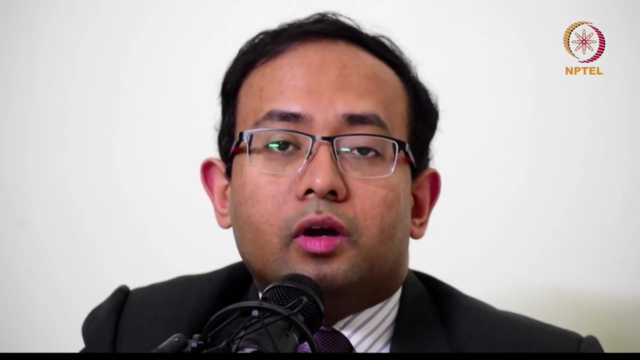 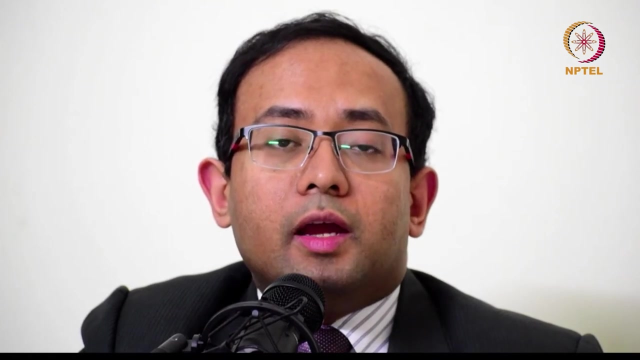 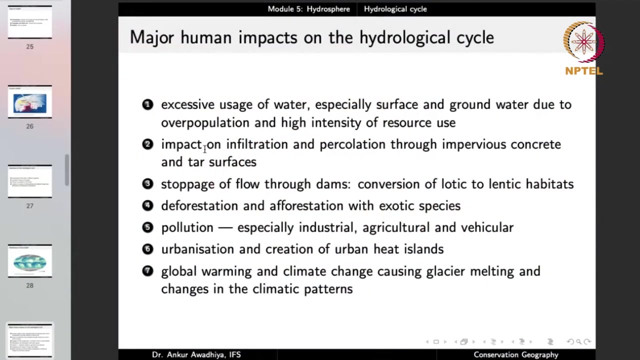 up. In certain cases, all that water has been drained out to make way for things like buildings. So you will often see that if you do not have the wetlands, then the amount of groundwater will go down, Because wetlands act as locations where a 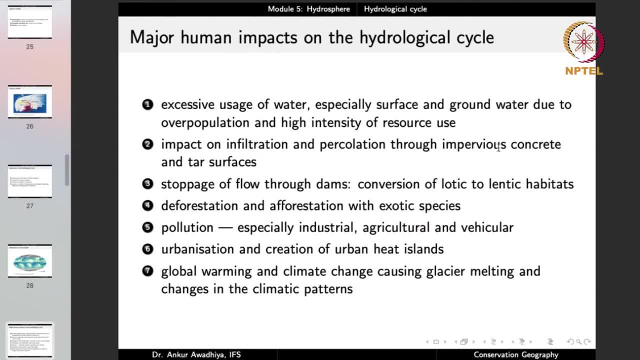 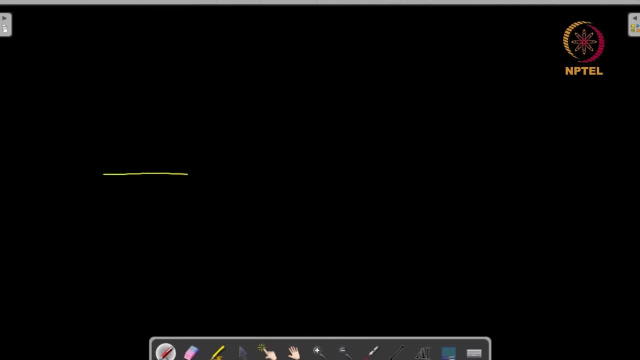 large amount of infiltration of surface water happens, Then most of the ground would be just covered with grasses, And grasses aid the infiltration of water by creating hindrances to the water movement. So, essentially, the water that falls in the form of rainwater. 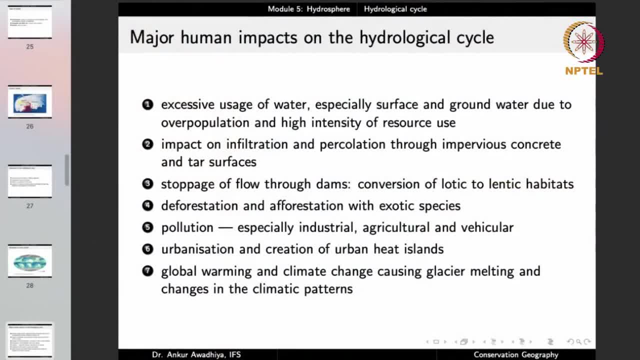 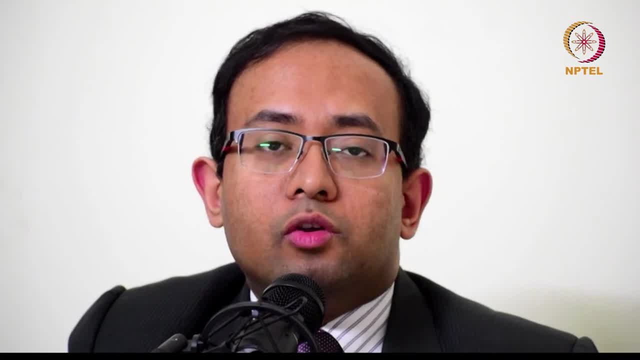 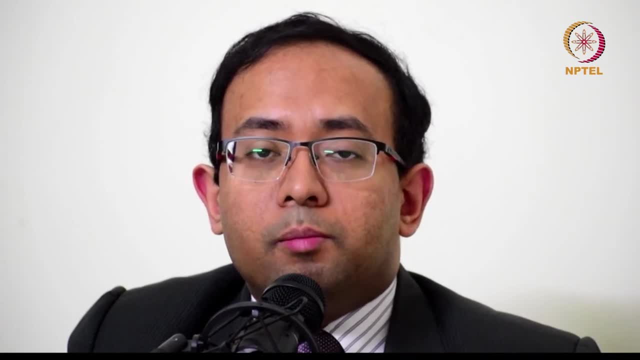 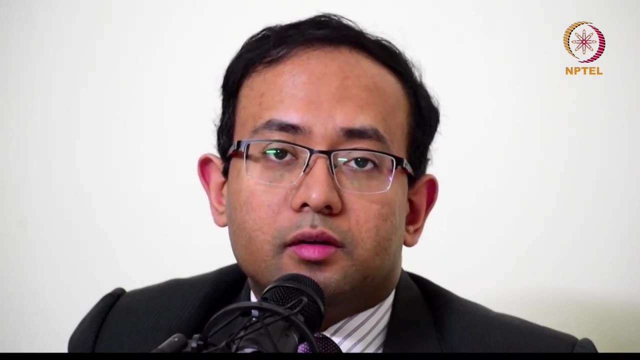 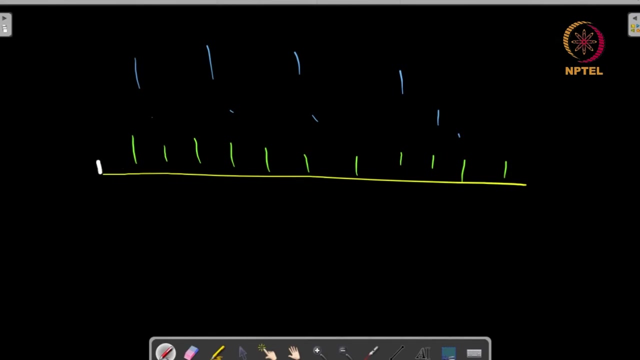 it is not able to move that fast because all these grasses are moving on the surface of the groundwater. So if the water is running, you have to make it to walk. If the water is walking, then you have to make a concrete surface, and we. 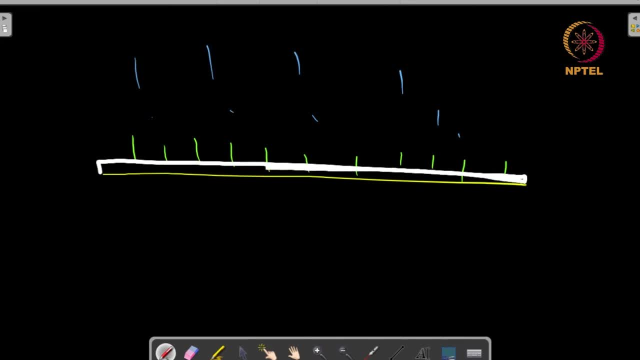 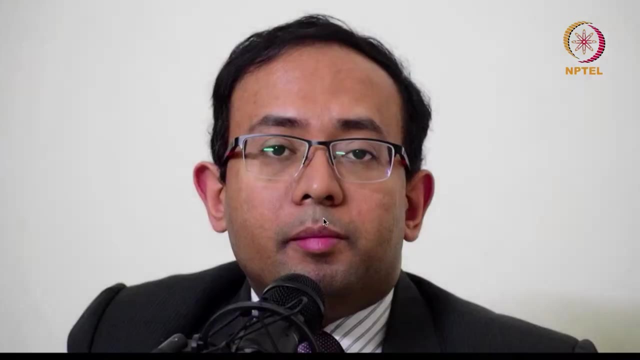 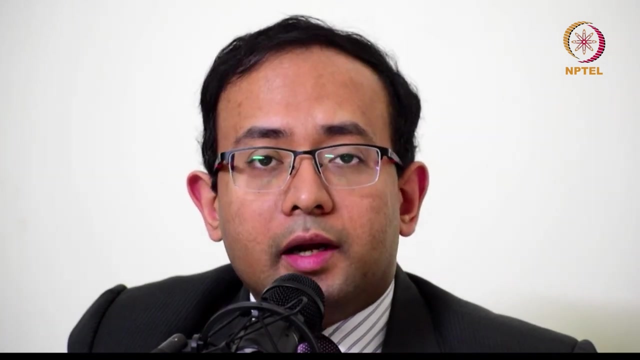 are covering this whole area with a concrete surface. Now, if you have a concrete surface, or say a tar surface, then this water has nowhere else to go. It will only flow down, There will be no water, and all of that is hindering the flow. 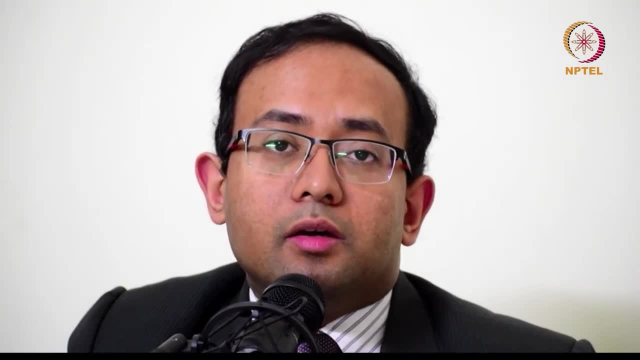 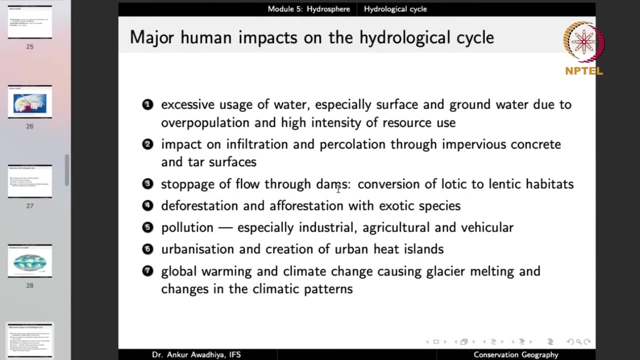 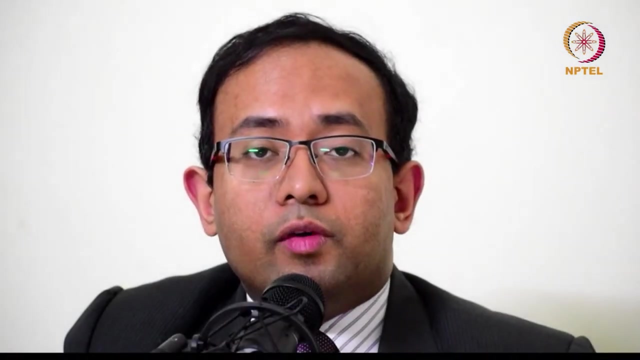 of water into the groundwater reservoir. So that is another impact that we humans are having on the hydrological cycle. We are stopping the flow of water through dams, converting the lotic habitats into water. Now, if we talk about the hydrological cycle, the water that 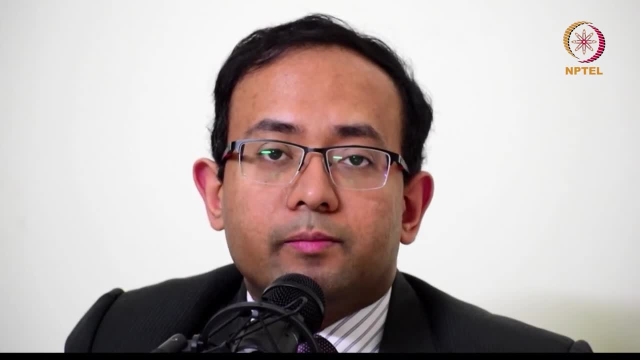 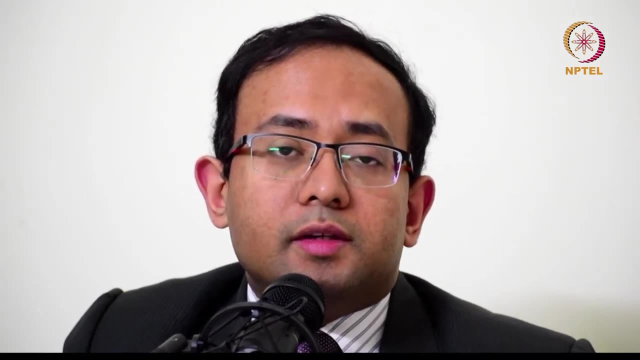 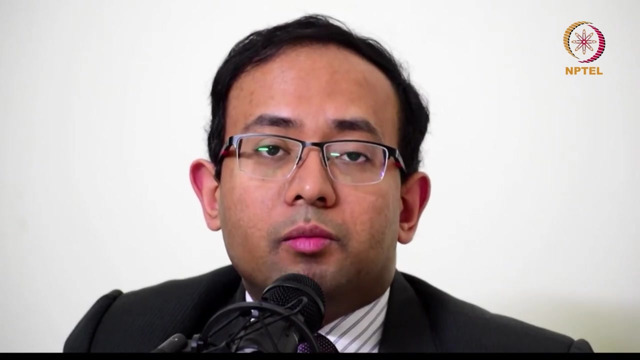 was falling on the ground. it was moving towards the oceans through the streams, through the rivers. Now, when we stop that water, what happens is we create an artificial wetland. Now, this artificial wetland may be in a sediment that were being moved by the rivers. 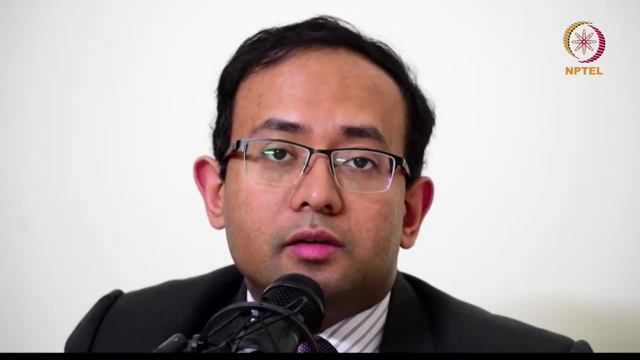 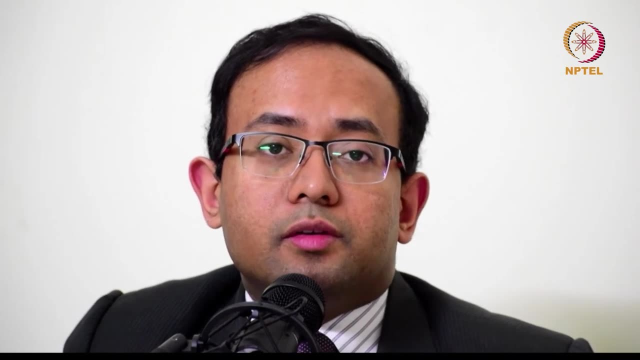 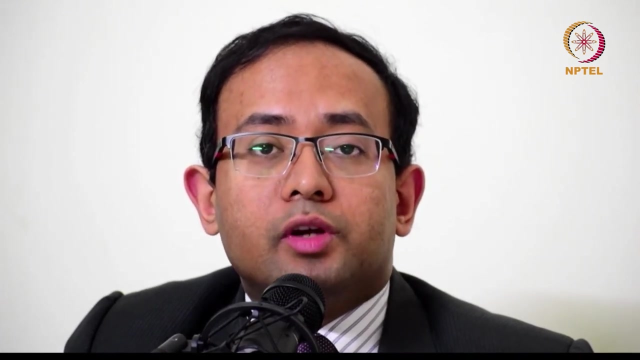 The salts that were being moved by the rivers. they are now stopping, they are now getting accumulated, and that will lead to environmental consequences. So we are not just over utilizing water, we are not just hindering the movement of water, but we are also reducing the amount. 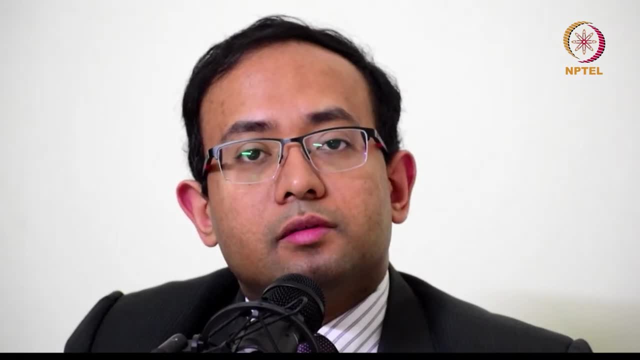 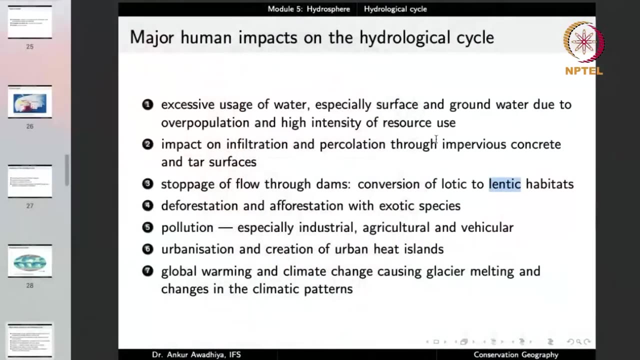 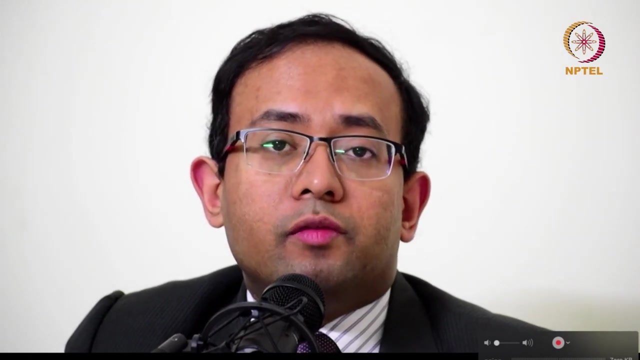 of sediment that is being brought by the rivers. So we are now facing a situation where a large number of our deltas are shrinking, they are disappearing. Then we are doing deforestation and, at times, afforestation, but being done with the trees. then we are impacting. 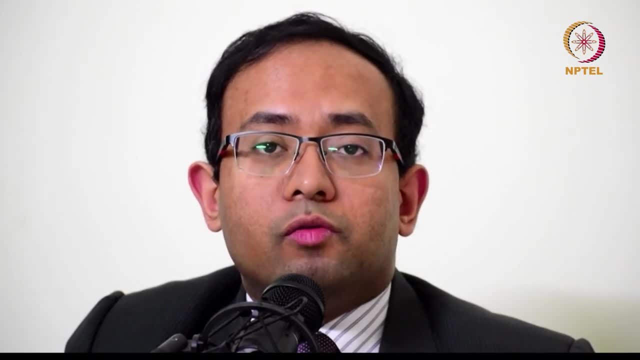 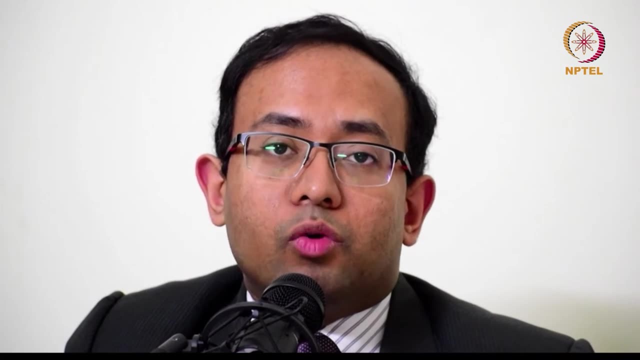 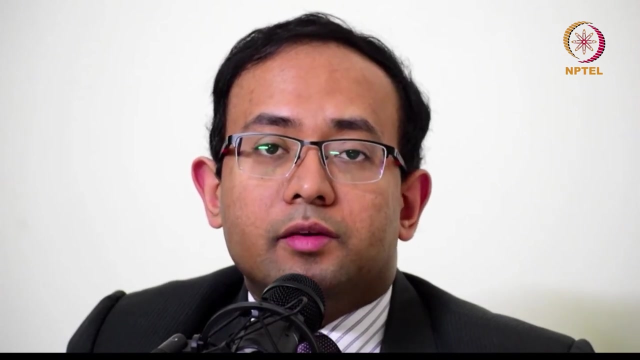 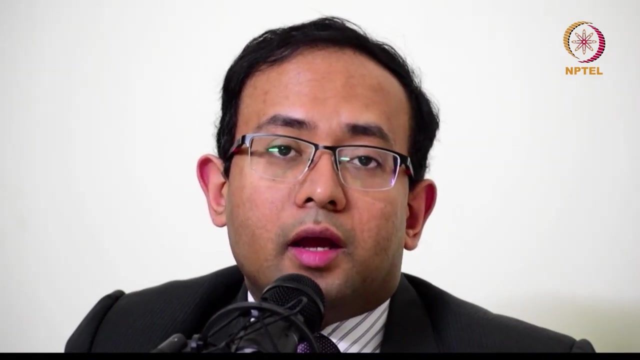 the hydrological cycle, not only because the trees perform a vital role of transpiration, but also because the trees hold up the water and aid in the ground water recharge. So in a number of cases we are cutting up the trees, making way for, say, agricultural fields or 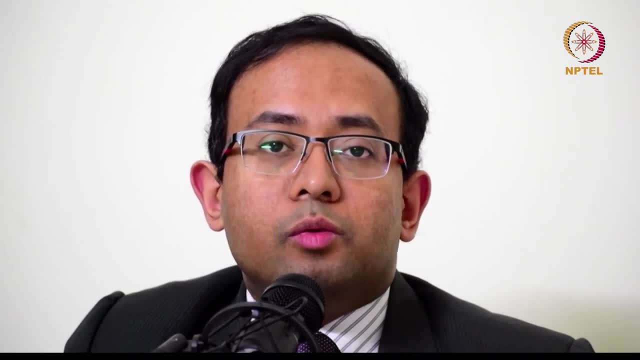 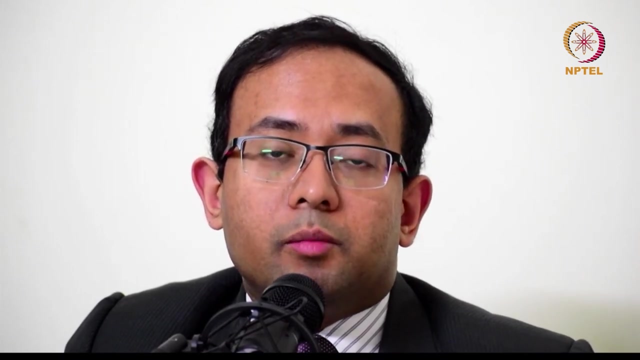 habitations. So we have to change the species composition. So we remove those species that are natively suited to that habitat and we plant trees brought from outside. Now, these trees that are being brought from outside, they might not be that well suited to the 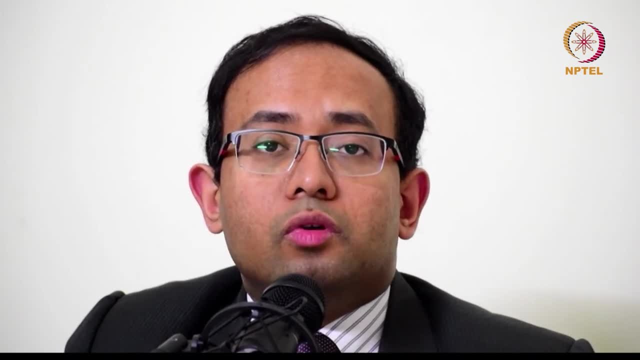 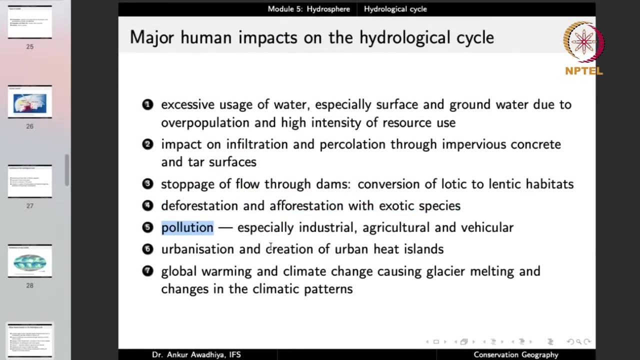 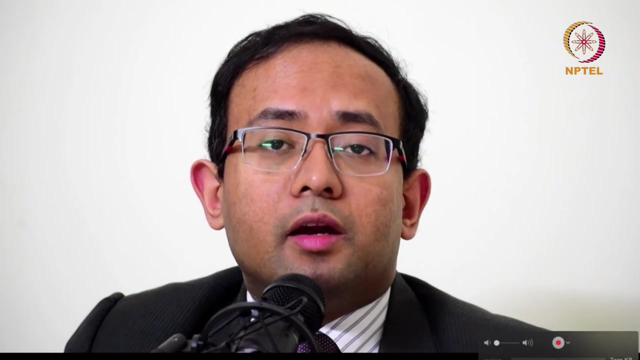 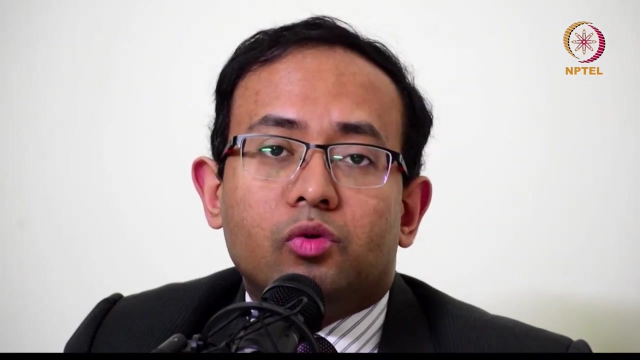 habitat. So essentially it is possible that they take out this particular habitat. So this is another impact that we are having: Pollution, especially industrial pollution, agricultural pollution and vehicular pollution. So all of these pollutants that we are generating, a large portion of it is 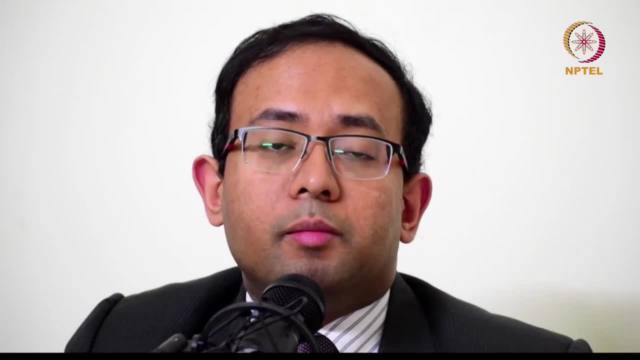 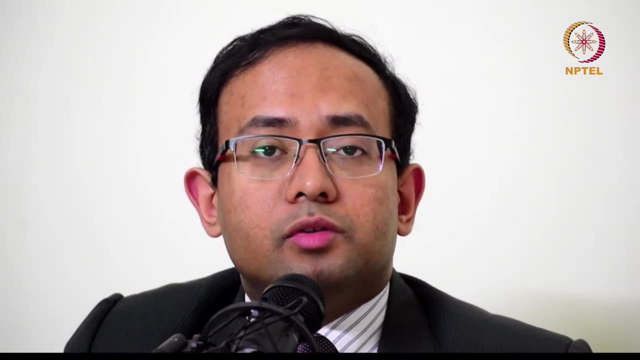 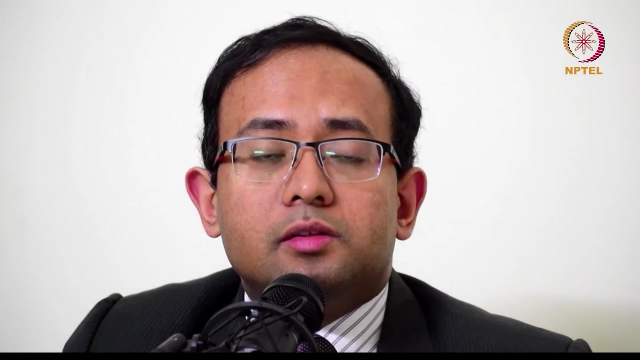 getting into our water bodies. If you look at the plastic bags that people throw out a large portion of their water bodies, they get trapped in these plastics. they eat up these plastics. that choke their elementary canals. but at the same time it is also polluting. 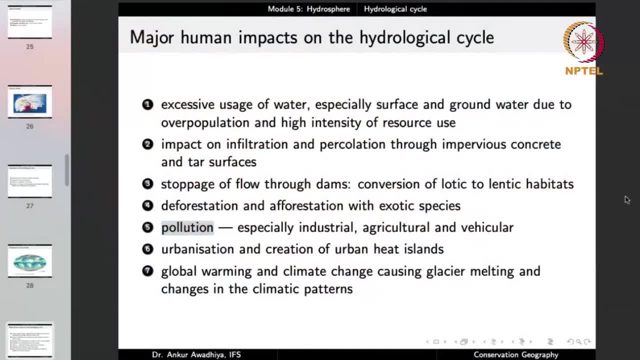 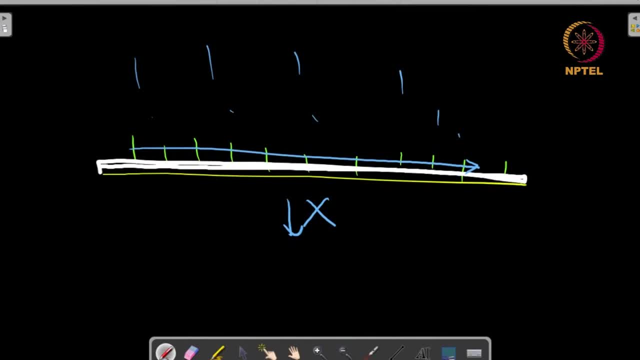 by releasing a large number of chemicals into these water bodies. So this is another impact: Urbanization and creation of urban heat islands. So what is an urban heat island? So in a certain area, you have a concentration of buildings and roads, So these 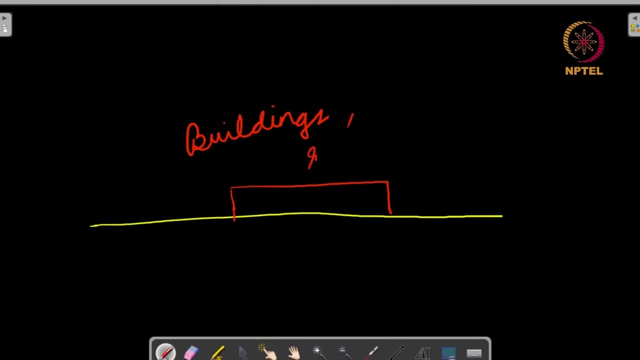 are large in numbers, but things such as trees or things like wetlands, they are less in number. If you look at our cities, you will find this situation. So in the cities we have a large number of buildings, we have a large number of roads, and there 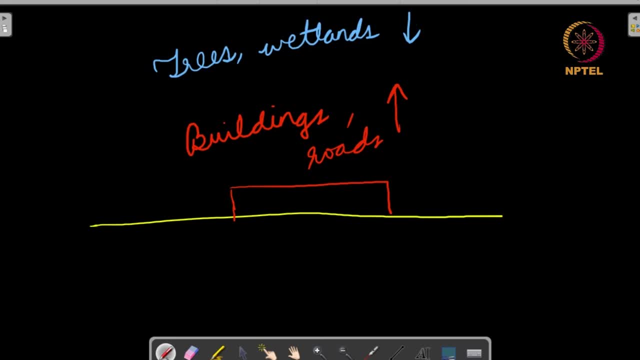 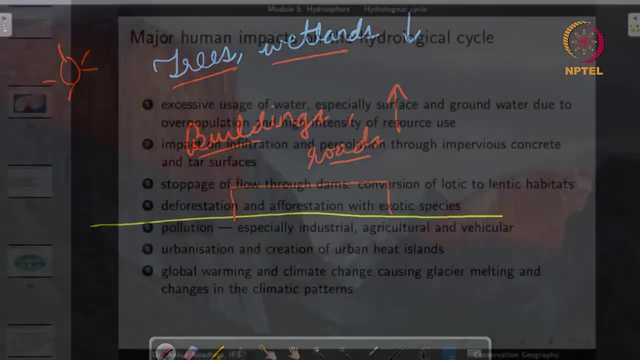 is very little amount of trees and wetlands because they have essentially been removed to make way for buildings and roads. Now, when we talk about the energy from the sun, if you have trees, they will be shade. if you have wetlands, they will be shade and in. 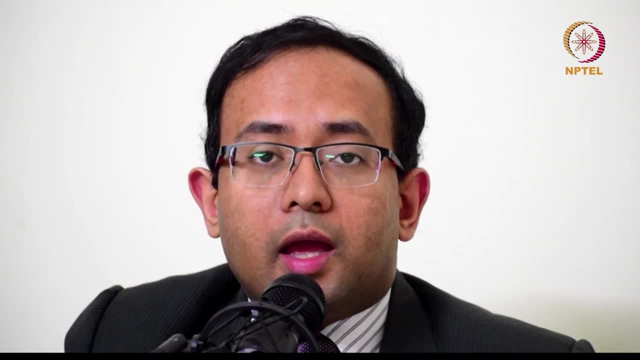 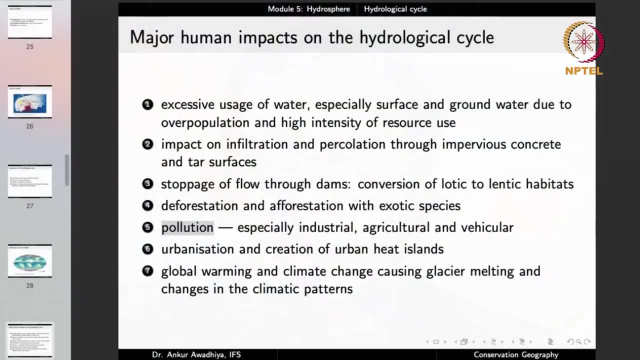 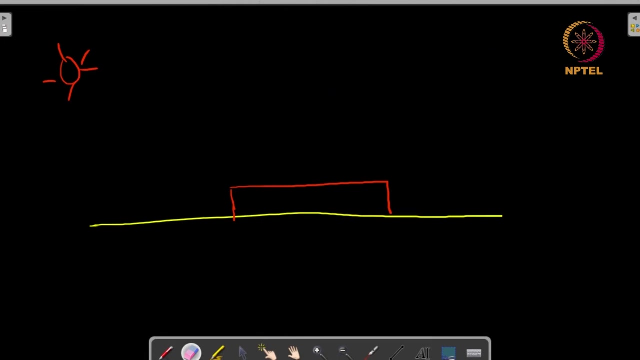 the case of these structures, the buildings and the roads, they absorb the heat, they retain the heat and in that case what happens is that these areas become warmer than their surroundings. So, essentially, if you look at these areas, if we say, be average, but then the temperature here will rise, then it will fall again here. 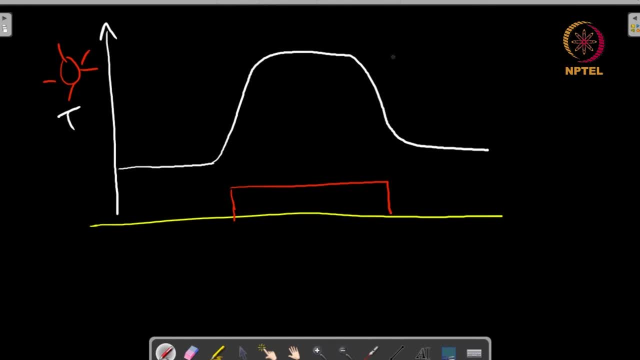 So this now looks like an island on a temperature chart. So this is an urban heat island: urban because it is being created through urbanization, heat because the temperatures are high, and island because this is an anomaly of high temperature that is surrounded by areas that are having a lesser temperature. 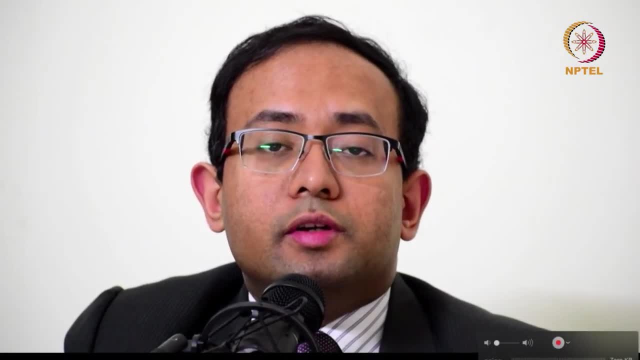 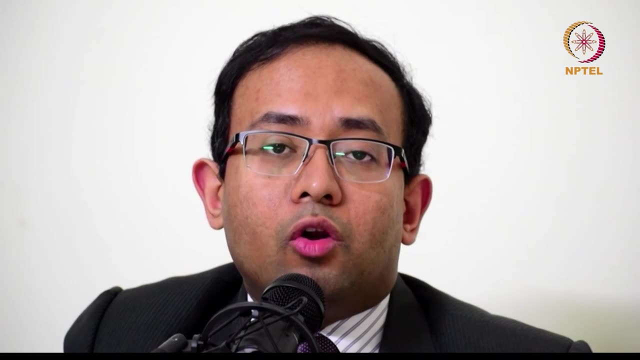 Now, when we create these urban heat islands, we also disrupt the hydrological cycle. Why? Because in these areas we are creating a situation where a lot of convection will happen because these areas are getting heated up, But because these areas have less amount of water, we are putting dry air upwards. 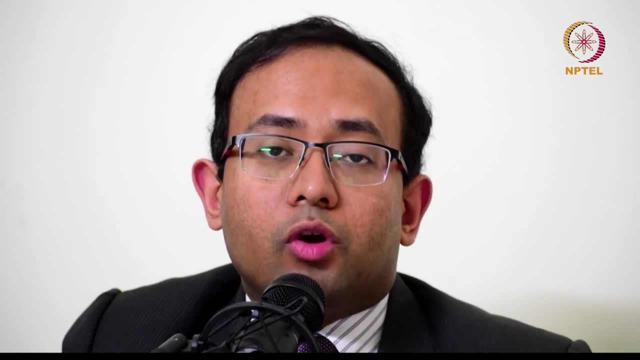 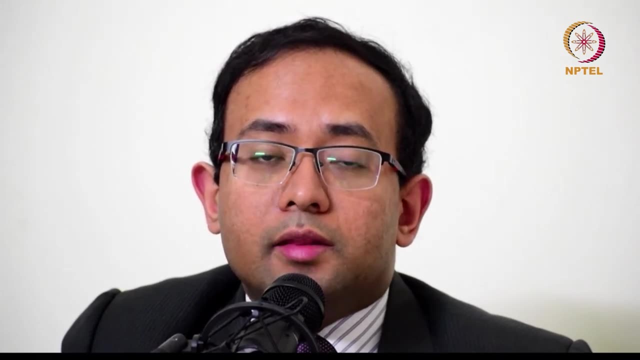 At the same time, When we talk about, When we talk about precipitation, when we talk about condensation. condensation can only happen when the temperatures in the upper atmosphere are low. Now, in this case, we are adding up heat into the upper atmosphere as well. 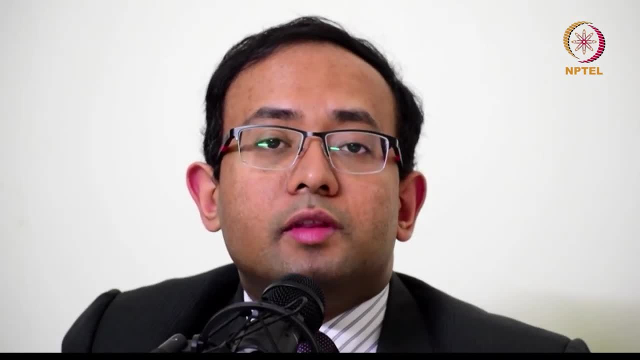 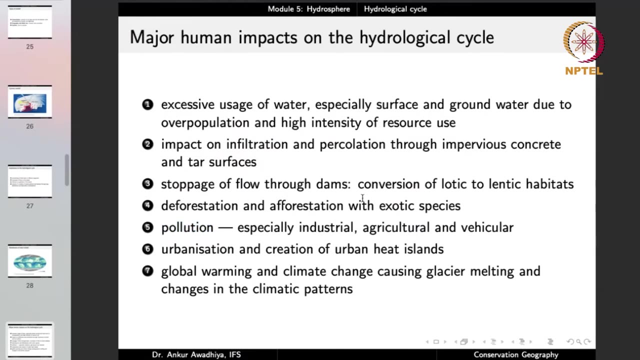 So this disrupts the hydrological cycle. We will not have that much amount of rains as we were having before, So this is another impact on the hydrological cycle: creation of the urban heat islands. Another impact is global warming and climate change. That is causing the melting of glaciers and changes in the climatic patterns. 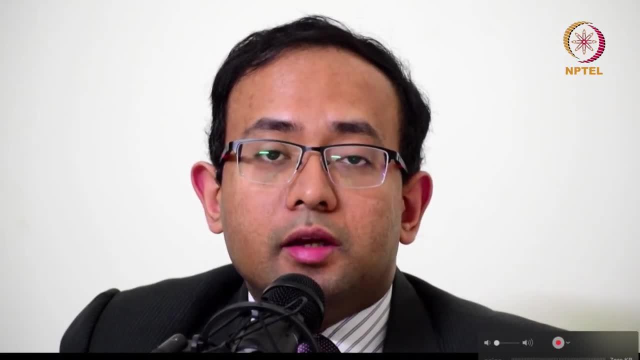 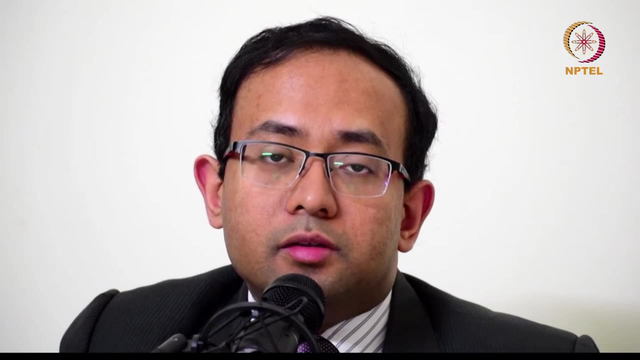 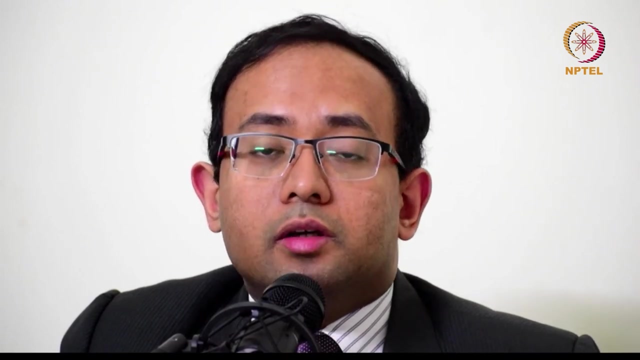 So, through global warming, what we are doing is that we are changing the temperatures of the planet. The planet is becoming more and more warmer. We are changing the wind patterns, We are changing the places where rainfall used to happen, We are changing the type of precipitation. 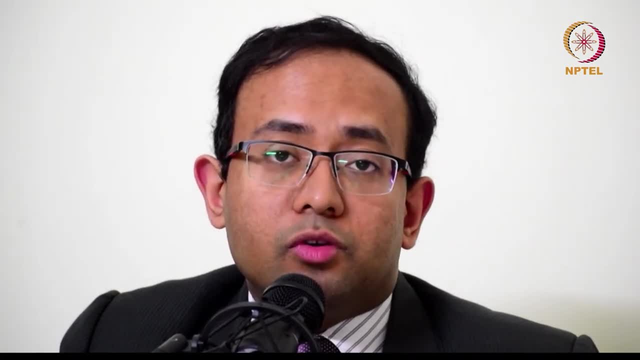 We are changing the seasonality of precipitation, We are changing the distribution of precipitation, We are changing the temperature, We are changing the temperature of precipitation. So, in effect, what is happening is that we are getting more number of extreme climatic events. 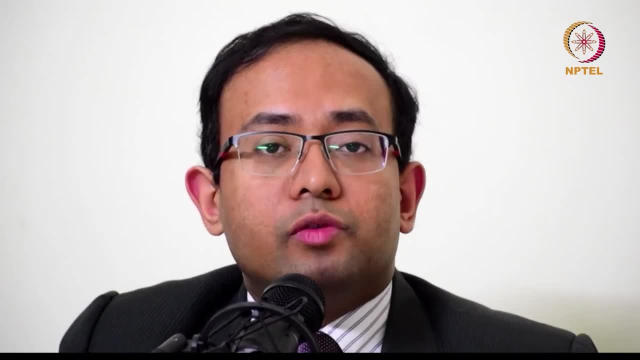 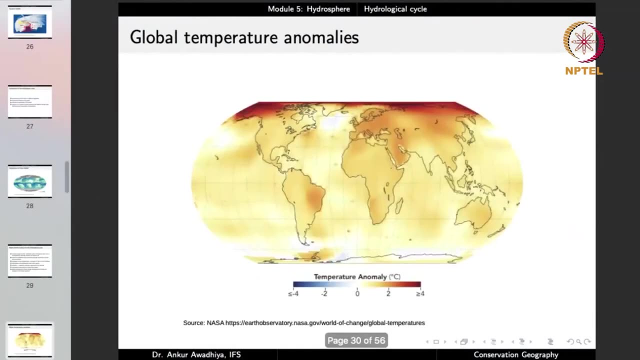 We are pushing certain areas towards droughts, We are pushing certain areas towards floods, which is another disruption to the natural hydrological cycle. So if we look at the global temperature anomalies, we find that here the yellows and the reds represent an increase in temperature and blues represent a decrease in temperature. 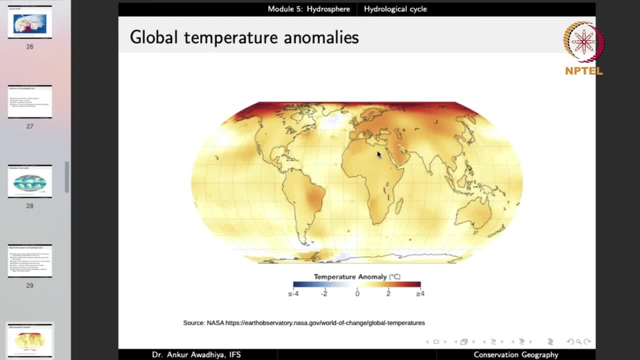 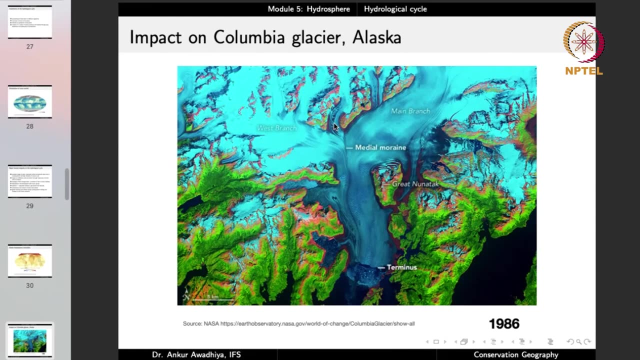 And if you look at the world map, we'll find that roughly every place is now yellow or red, except, say, a few patches here or a few patches here. roughly all of the world is heating up Now. what kinds of impacts is it having? 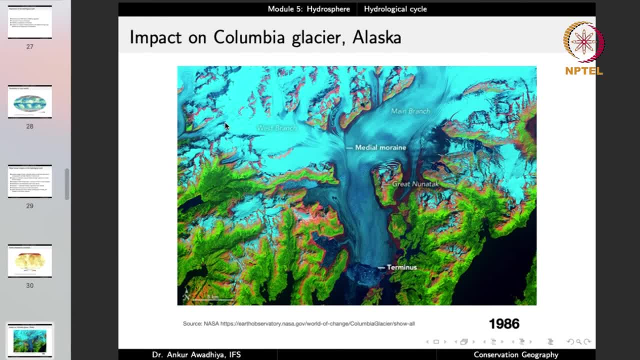 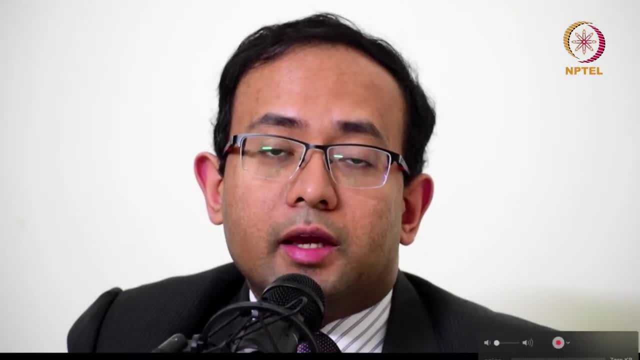 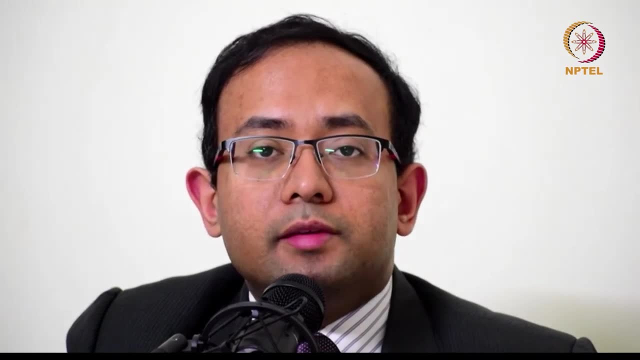 So this is an image of the Columbia glacier in Alaska and this is a false color composite, So this is Not exactly the color that we accustomed to saying. the true color composite would have shown a glacier in white color, but this is a false color composite, which means that we are playing with the bands of the satellite. 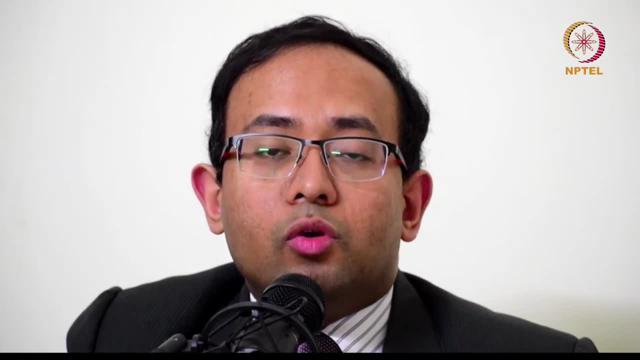 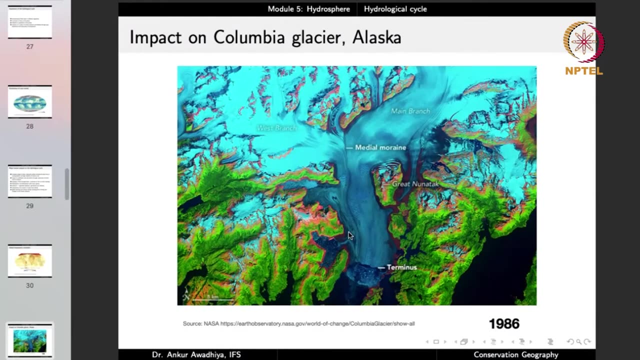 imagery so as to enable us to look at the phenomena more clearly. So in this band combination it is easy to see things like the moraines. Now, in this case, this is an image from 1986 and we find that this Columbia glacier, it has a west branch, it has a main branch. there is a medial moraine in. 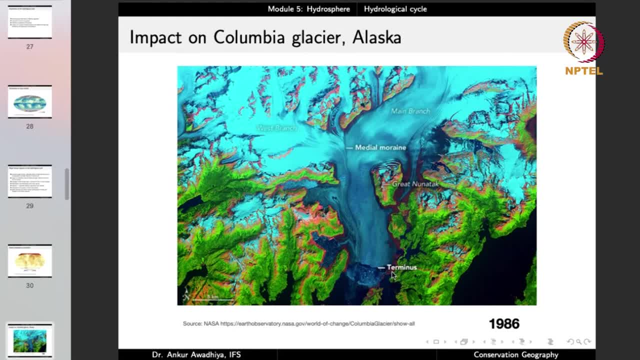 between, and this is the end of this glacier. So this is a pretty large size glacier. This scale is five kilometers, so the width of the glacier is somewhere around three kilometers in this area and it is getting ice and snow from all of these different areas. Now let us look at what we have. 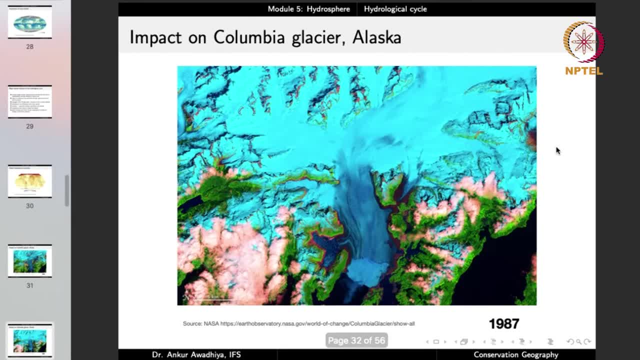 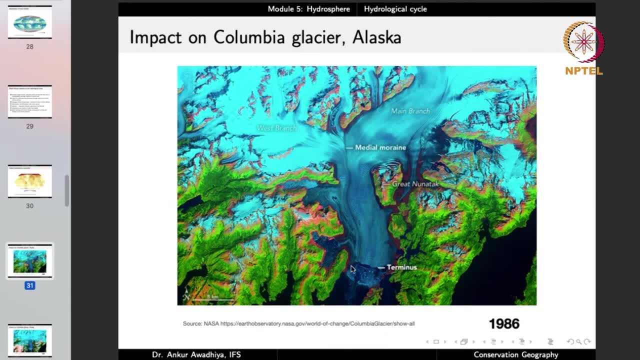 done to it. So this is the image from 1986.. This is the image from 1987.. So the major difference, what we are observing here is in this location. So earlier this was the the terminus, and we find very small number of ice chunks that. 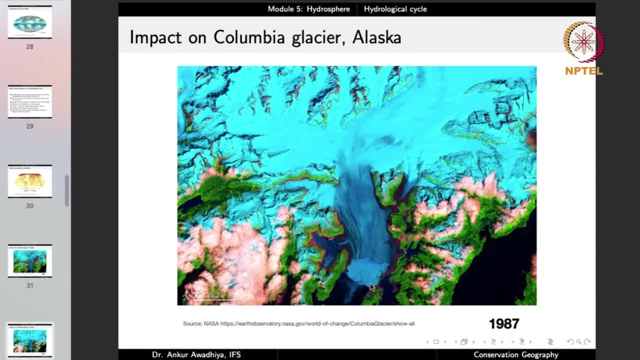 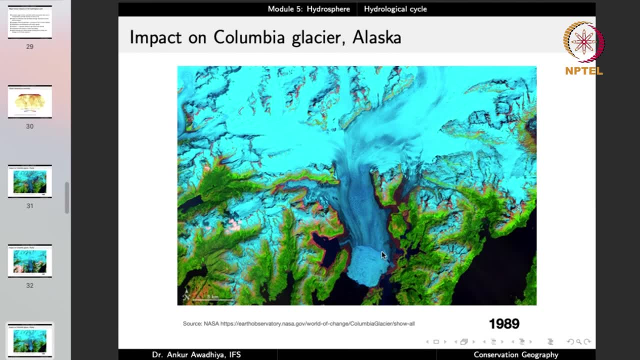 are moving into the ocean. Now. the ice chunks are much more in number By 1989. now the tip has shifted back, So earlier we had started from a terminus at this point, So let us put the cursor here Now. the terminus is here. 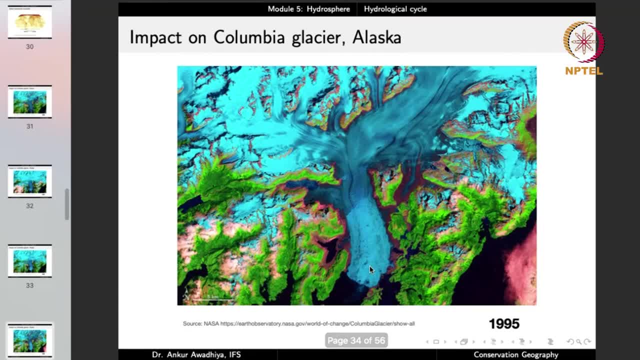 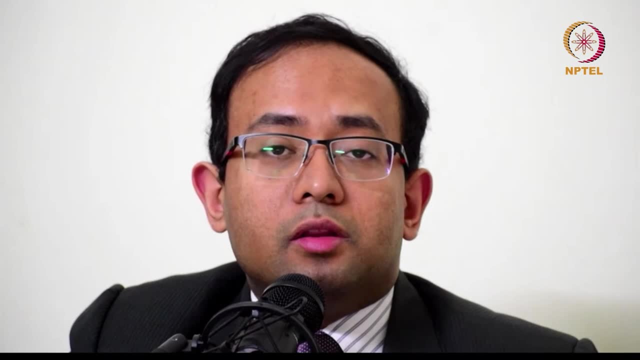 So this is the image from 1989. this is 1995, and you can observe that now the glacier has shifted to this location. The glacier is melting, The glacier is disappearing. Now remember that when we talked about the ice caps, in the case of Antarctic icecaps, the water had a residence time of roughly 20,000 years. Even in the case of the Alaskan glaciers, the water has a residence time of several thousands of years. but now the water that we just was stored up, that would have remained in that place for very long period of time- that is now melting up at a very fast pace. 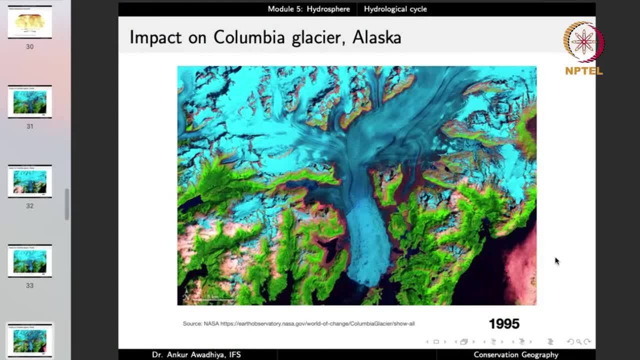 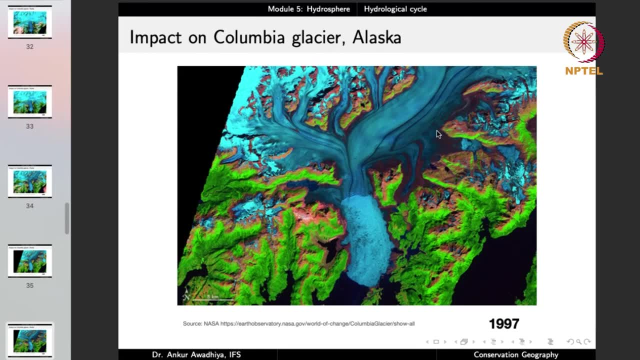 So this is another change that we are bringing. So this is the image from 1995,, 96,, 97, and now you are observing that the ice is changing its color because there is now a rapid amount of melting everywhere. Now the melted water creates pools, it creates small streams, and so they look very different. 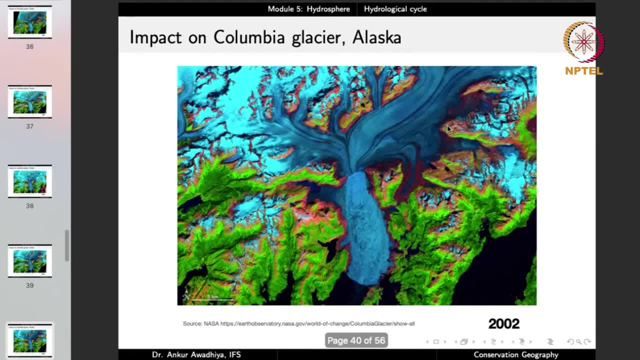 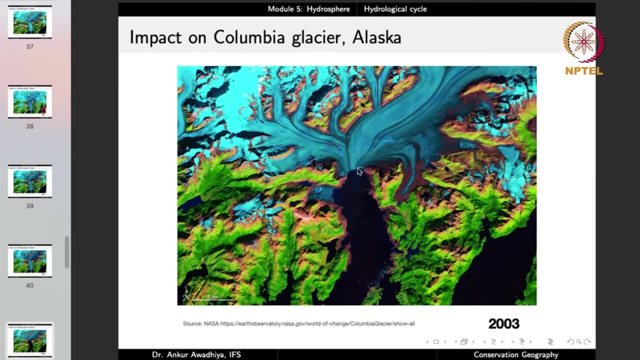 This is 1999,, 2000,, 2001,, 2002, 2003.. So we had when we began, we had the terminus here. now you have the terminus here, So all of this portion is now gone: 2004, 5,, 6,, 8,, 9,, 10,, 11,, 12,, 13,, 14,, 15,, 16,, 17,.